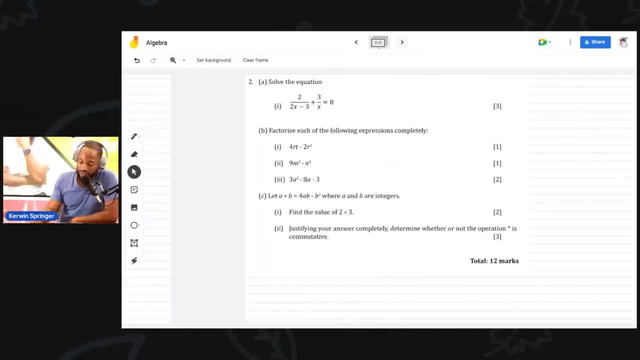 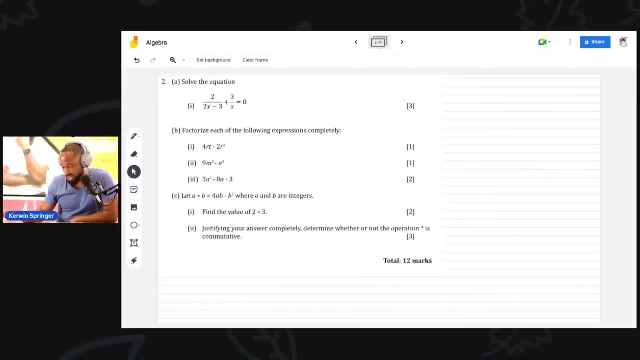 to see you. Jerome Kasim, Everybody press like on the stream Now that I'm live here. now that I am live here, YouTube should send it to more people, So more people should be coming in. All right, so I hope you can make the numbers We make. 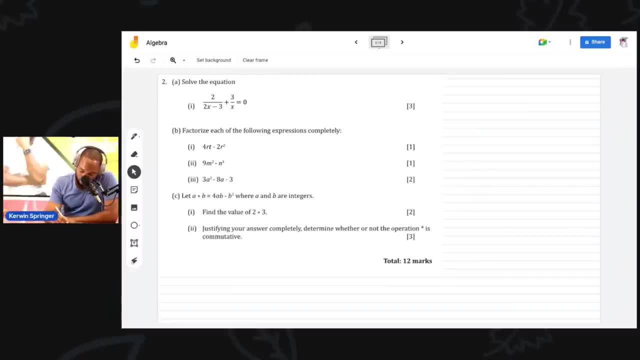 let's see, maybe at 200, 300.. So there you see two. all right, well, let me know when you reach 200.. If we reach 200, 2x minus 3 plus 3 over x is equal to 0.. This topic is called algebraic. 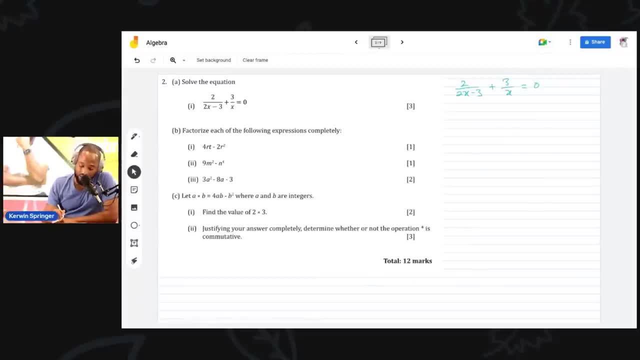 fractions, algebraic fractions, And the key to this topic is being able to find the LCM of an algebraic expression. So, in this case, what I want you to do every time you see this, and it's very popular- in number two, we're doing algebraic. 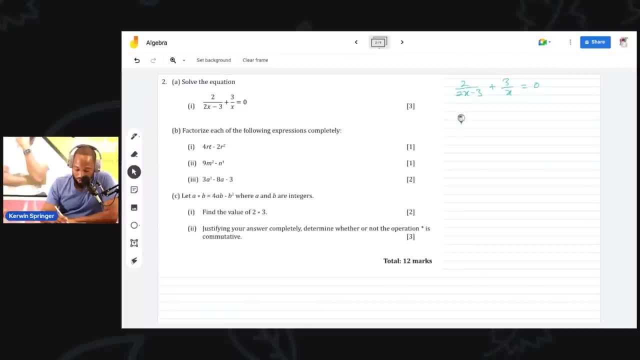 It's to just put the product of the two of them. So put 2x minus 3, put it in brackets and multiply it by the x and put a line like this. They call that a vinculum, or viniculum or some. 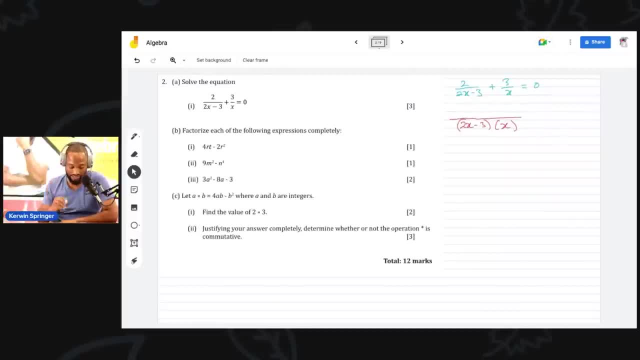 kind of thing. And then this is the LCM thing, like this- Remember this Watch- like two-thirds plus one-fifth, and then we get the LCM, which is like 3 by 5,, 15. So 15, and then it'd be like: 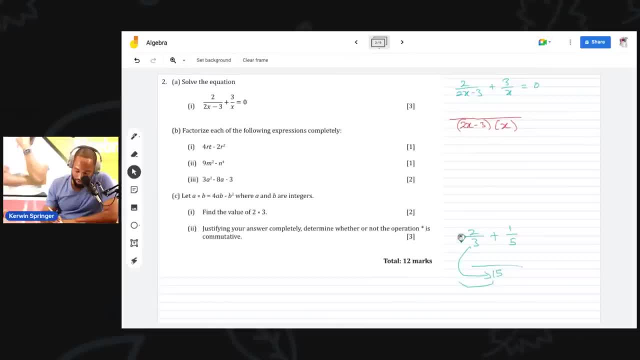 3 could go into 15, five times, and then you see 15 times, and then you see 15 times, and then you see 5 by 2, 10.. That's the same vibe we're doing. It is the same vibe. same vibe, ladies and gentlemen. 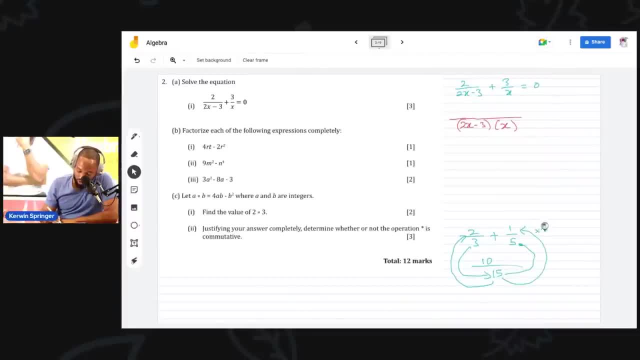 5 into 15,, 3.. So you'd say 3 by 1 is 3.. And they used to make all the right-out all the weekend and things for that back in the days. Now you don't need to write all the weekend for that. 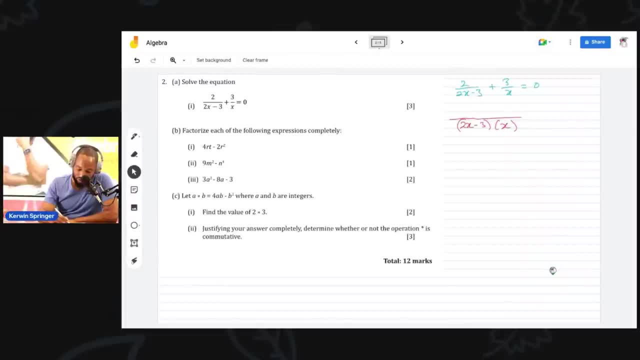 So tell me if you're going to follow what happened here. I'll say 2x minus 3 into the denominator. It will cancel with this and the x will come out and the x will have to go and multiply by the 2.. 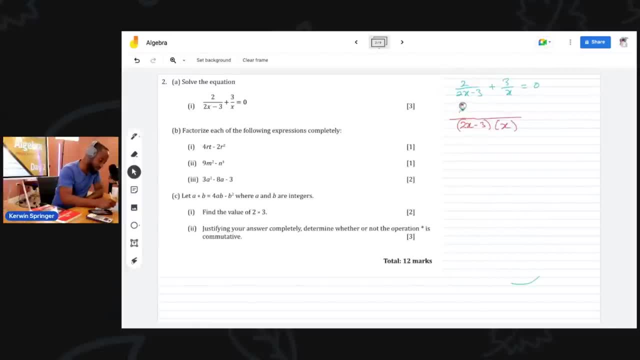 All right, agree, You agree. So it'll end up with 2, and you can think of the x coming here one time, And then, similarly, you should end up with 3 by 2x minus 3.. 2x minus 3.. So why is it in the chat? if you understand that flow, That is. 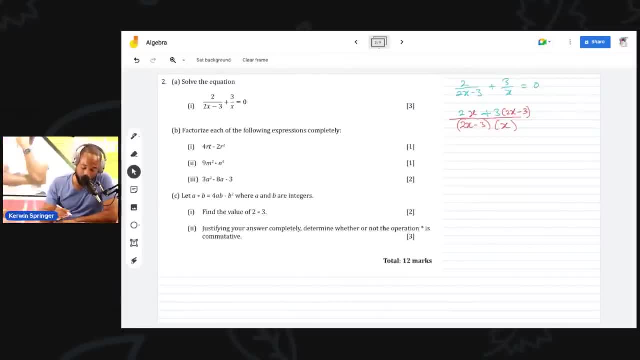 that is very likely. what's going to show up in your exam? You're going to see something like that in your exam. One of this, one of this, is going to be in your question 2.. So now we have 2x plus 6x minus 9.. If it's blurry, if it's blurry, it's on you. 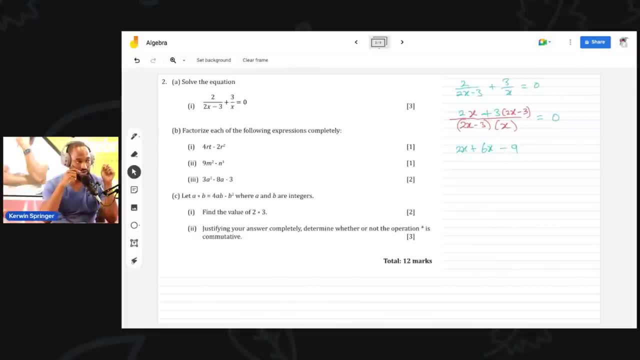 And this is coming across crystal clear. So if it's blurry, you have to go on your YouTube setting and increase your visual setting from maybe some kind of low to higher quality, right? Okay, 2x plus 6x, What did I do? What did I do? class? 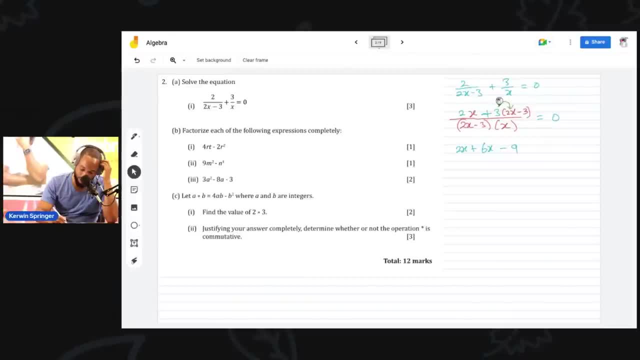 We start off kind of slow today. boy, I multiplied the 3 by the individual terms in the bracket. That's called expansion or distribution. So verify that my numerator. Look, it's a good day And what's going in the denominator? 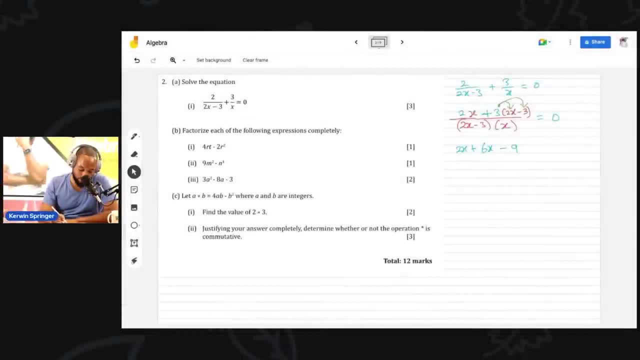 What's going in the denominator? What's going in the denominator? So, what's going in the denominator? It's 2x minus 3.. And x is equal to 0.. Now, because this is equal to 0, it means that the denominator is 0.. 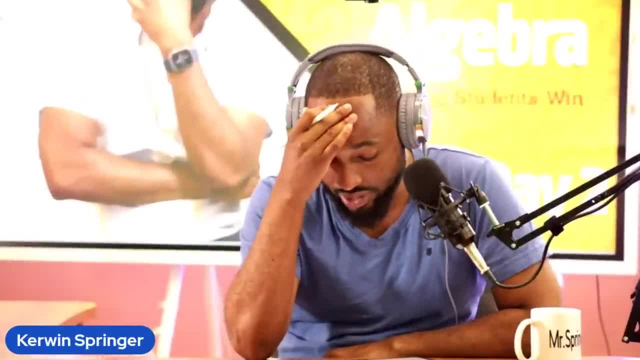 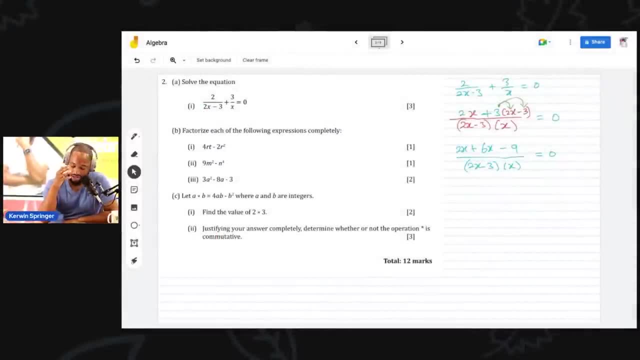 For this to be equal to 0,. the only thing that can happen is that the denominator is equal to 0. So that kind of that kind of um eliminates the denominator from the situation. I'm thinking of another way I can do this. 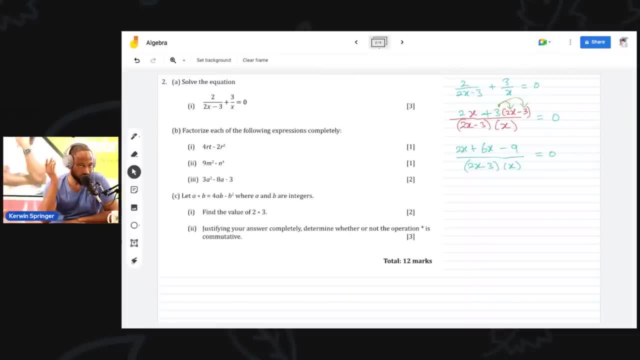 There's actually a faster way. I'm seeing that I could have mashed up this question, But anyhow, this is what's going to happen here. The denominator- I shouldn't say equal to 0.. The denominator, when it multiplied across, will be eliminated by the 0.. 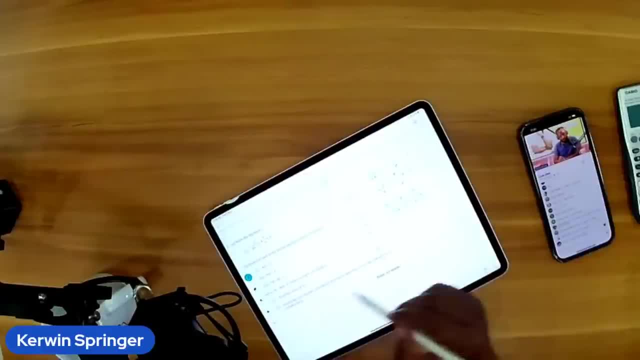 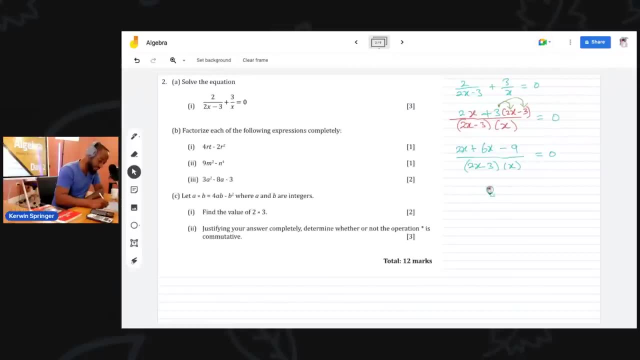 So, like, if I multiply the denominator by the 0, I would get? I would just end up with 2x plus 6, which is actually 8x minus 9 is equal to 0. So 8x is equal to 9, and x is equal to 9 over 8.. 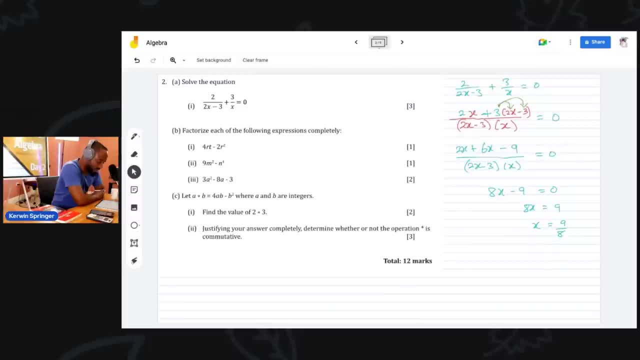 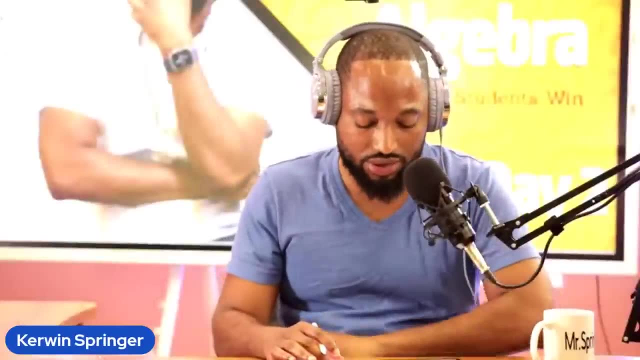 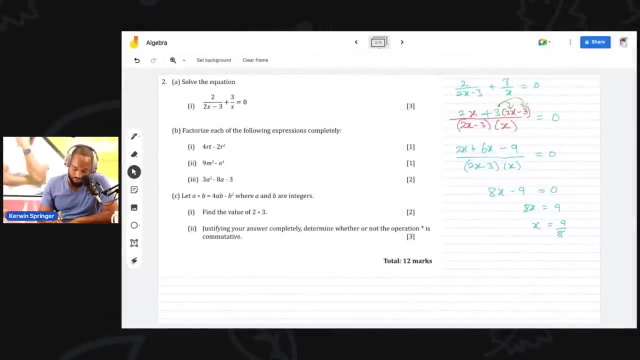 How many of you all get that 9 over 8.. Tell me, if you understand that, if it's making sense, What's the next way we could do this thing? What is another way we could get this done? Well, instead of using that LCM technique, which you have to know anyway, 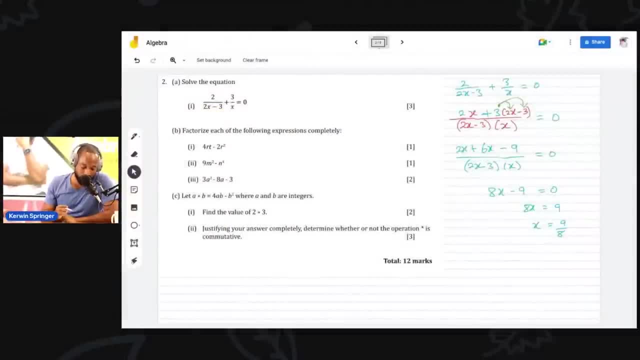 You had to know that LCM technique anyhow. But if you want to not use the LCM technique, you could use the famous cross-multiply technique. It's a kind of cross-multiplying thing. Tell me if all you've seen this other way we could solve this question. 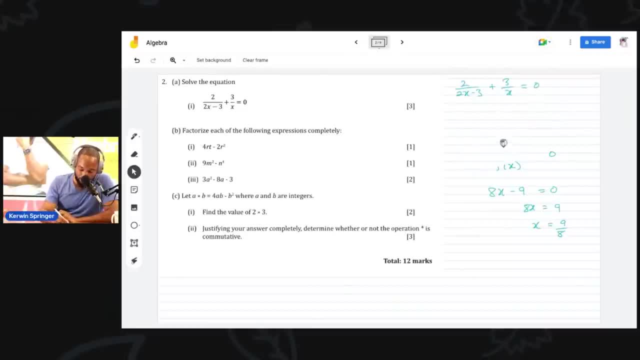 What we could do is bring across this term. Think of it as a term and we bring it across. So can you see that this would be 2? Over 2x minus 3. When you bring it across, you get negative 3 over x. 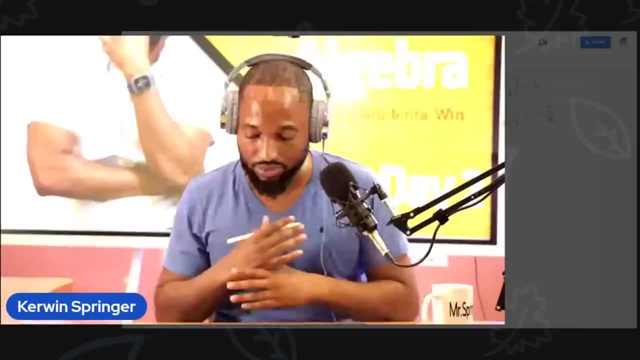 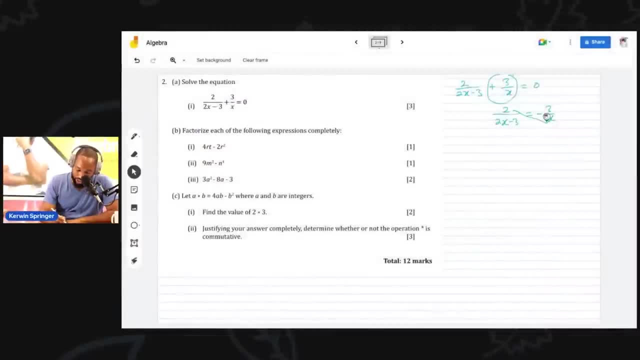 Then we do that kind of cross-multiplying: Wee-bye, daven-bye, levi-bye, chi-bye. We're going to do that kind of cross-multiplying. So the 2 will multiply by the x and the 3 will multiply by that. 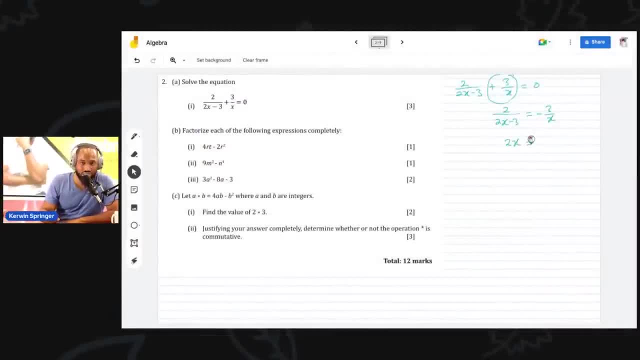 Watch it. So you're going to get 2 by x and the 3, let's have the 3. take the negative sign. So this is going to be negative 3 by 2x minus 3.. And we can't well, sorry, x by 2 is 2x, right. 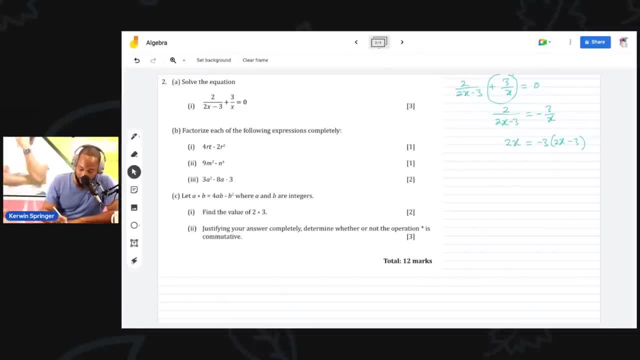 So, and we kind of boil down to the answer there already, because you'll end up with: 2x is equal to negative, 3 by 2x is 6x, And negative 3 by negative 3 is plus 9.. 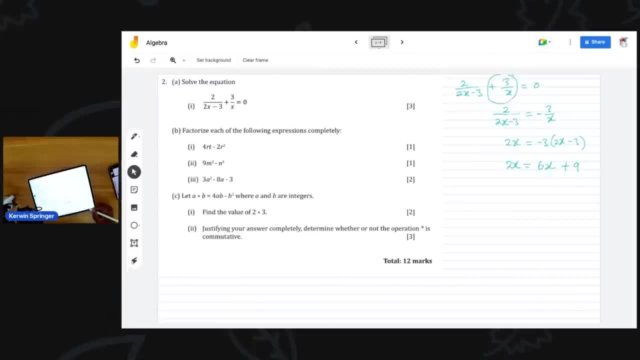 And when I bring across the 6x, what happens? It's actually negative 6x, because negative 3 by 2x is negative 6.. When I bring across the 6x, what happens? What happens, What happens. 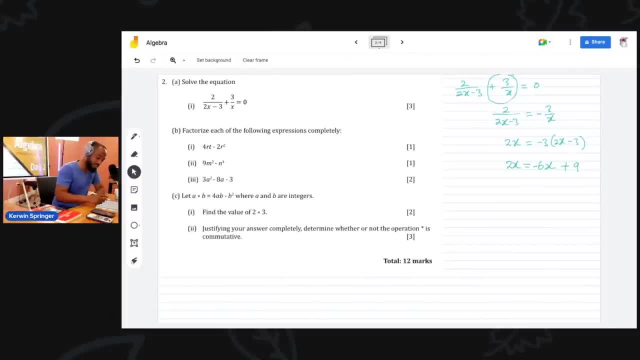 When I bring across the 6x. right, Tamara, if I bring across the 6x, we could just pin Christy's comment on the screen, because Christy can help you people who screen blurry. You'll get 2x plus 6x is equal to 9.. 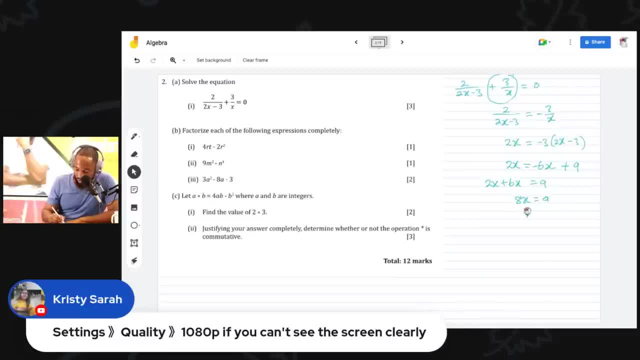 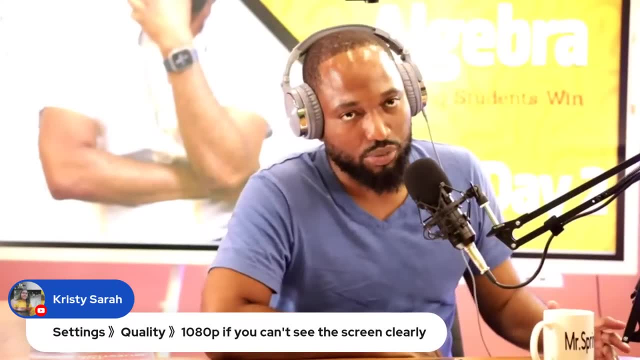 So that's 8x equal to 9.. And then it's just x is equal to 9 over 8.. So this way you didn't have to think about the LCM, And I think this is an easier method if you're not a superstar in mathematics or anything like that. 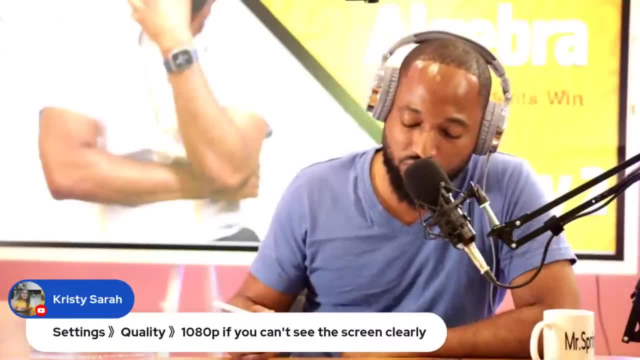 So you just bring across the 6x, You just bring across this and you cross, multiply and then you distribute and you move forward with your life. So that's the answer here. The answer is that x is going to be equal to 9 over 8.. 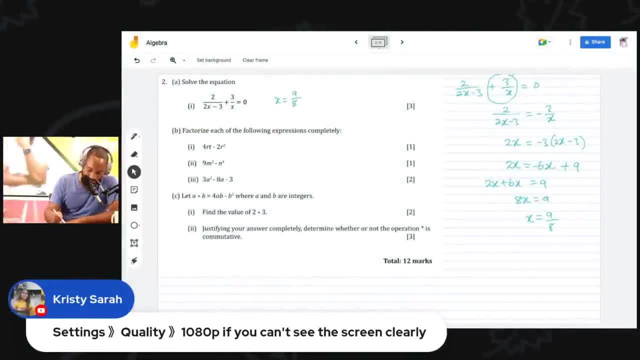 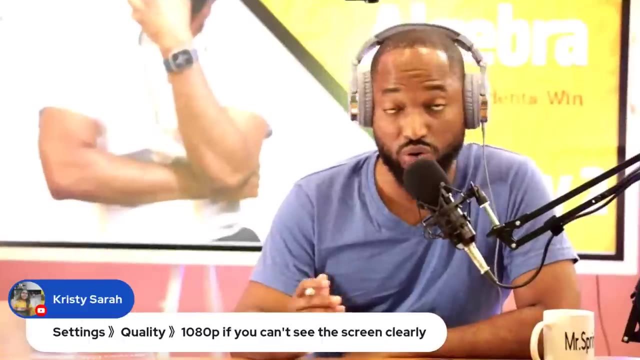 I want to clear up this space, to do the working for the next one, Because we need to factorize And in CX you will be asked to factorize either difference of two squares, quadratic equations- basic factorization- or grouping. factorization and grouping. 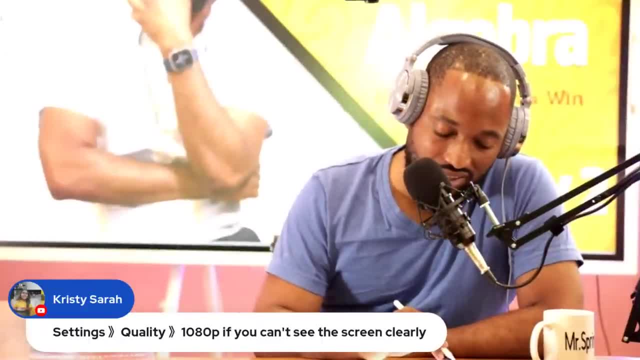 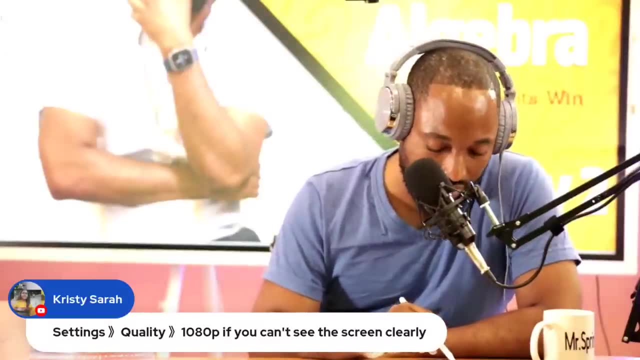 That's why they bring the four terms. So from this I could see this is just a basic factorization. It have the R squared here, yes, which kind of hinting towards a quadratic equation. but then it has an additional variable. 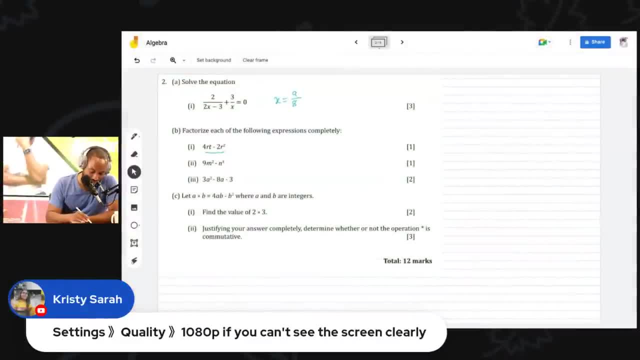 There's an additional variable, t. So what are t doing there? You see that t, So it's not really a quadratic because it have two variables. That's not a concern. That's messing us up. So you just need to find the like terms here and then hope for the rest. 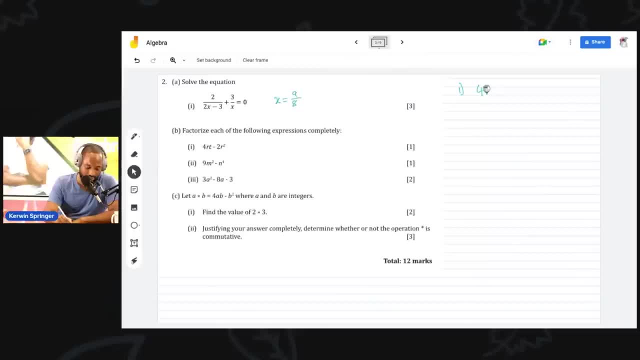 So for part one we'll have 4Rt minus 2R squared. What's common, what's common, what's common? So the questions with factorization, when you have basic factorization: what is common, what is missing? 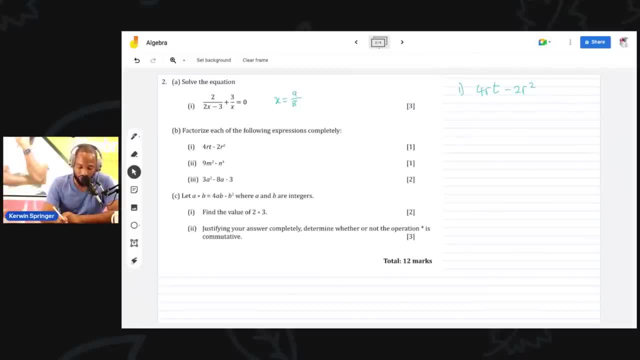 Two questions to ask What is common? Just 2 and R, 2 and R, So I can extract the 2 and the R, So I'll put equal for the 2 and the R here And then in the brackets. I want to put back what is missing from the individual terms. 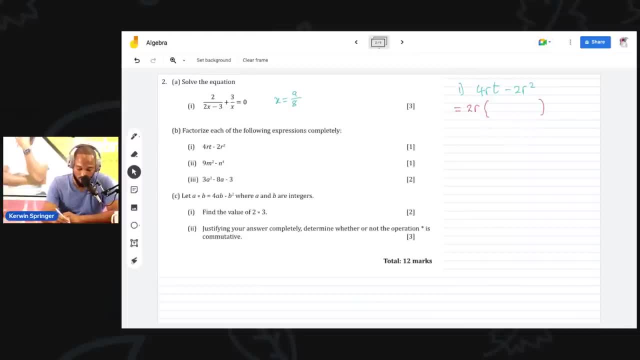 So what is missing? A 2, because I'll need the 2 by this 2 to create the 4.. So 2 and a t, because there was no t here, So 2t, that's good. 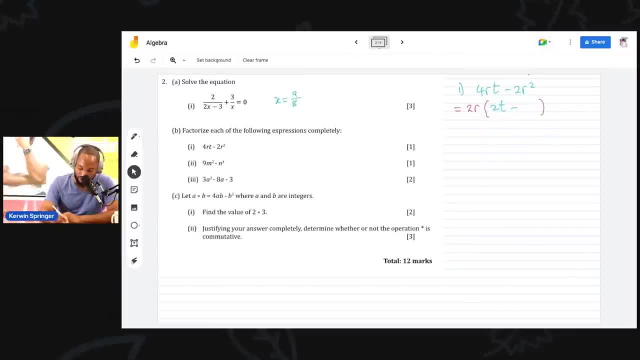 And this one already has the 2, so I don't need to put the 2, but it's missing an R. R by R is R squared, And just like that. Jason, well done, Jason. well done Jason again. and Shemar. 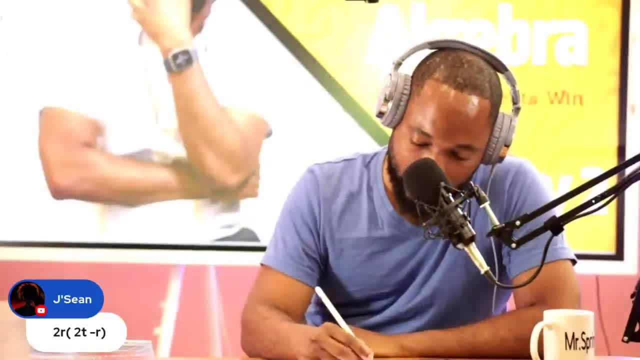 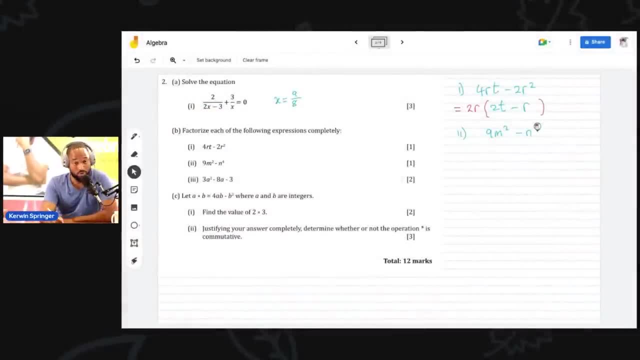 Yeah, man, people getting this thing up, people getting this thing up. What about the next one? 9m squared minus n to the power of 4.. So this could be a difference of 2 squares. because we seen, and the reason I know, I can't do basic factorization here. there's nothing really common here. 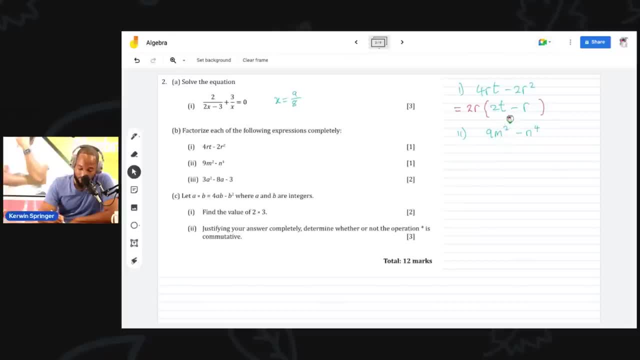 And there's a square here. there's a 3 to the power of 4 here, but don't worry, that is just like n squared by n squared. So this is 9m squared. 9 is a square number. so it's strong indication that I have to do. difference of 2 square terms. 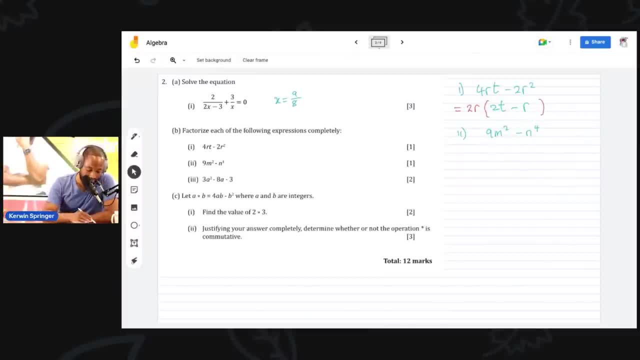 So I need to find the individual square root of each of the term like this: This is one of the techniques. we show how to do this difference of 2 squares. So we say the square root of 9m squared, the square root of 9 is 3, and the square root of m squared is m. 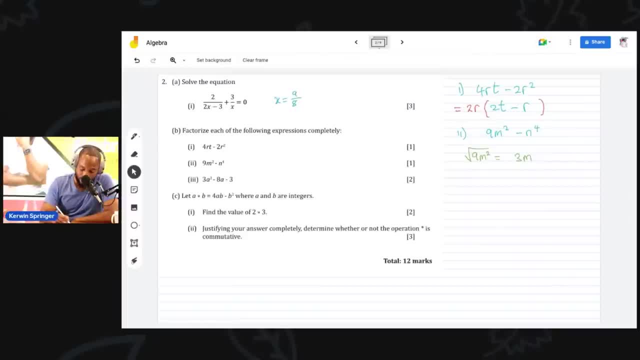 3m multiplied by 3m will give me back 9m squared. And what's the square root of n to the power of 4? 3m, 3m, 3m. The square root of n to the power of 4 is actually n squared. 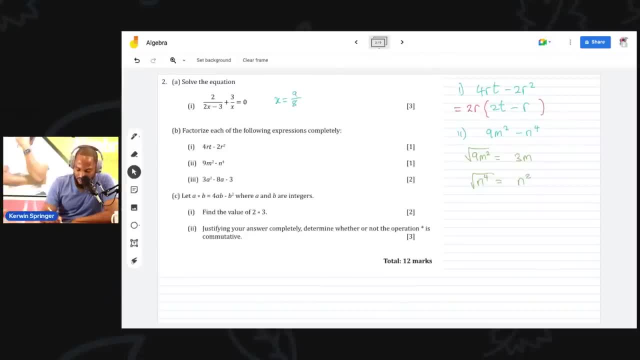 And we did some indices yesterday. So if I think we do some indices, n squared by n squared is n to the power of 4.. So if I get the square root of n to the power of 4, it means it's n squared. 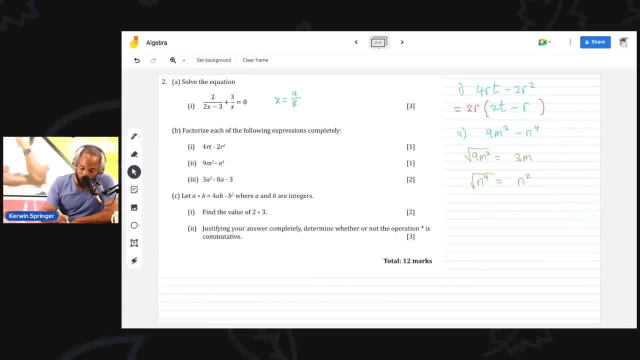 Making sense. So now that I have the square root of both terms in the difference of 2 squares, I can finish off strong and say: therefore, hit them a little. therefore, 9m squared minus n to the power of 4 is equal to these two terms. 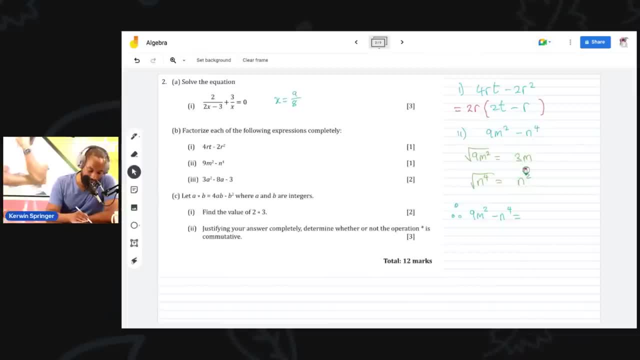 I want to put them in a kind of binomial situation like this: 3m minus n squared multiplied by. I'm running out of space here, boy. Oh Jesus, Jesus and ages, All right, let me see, let me see. 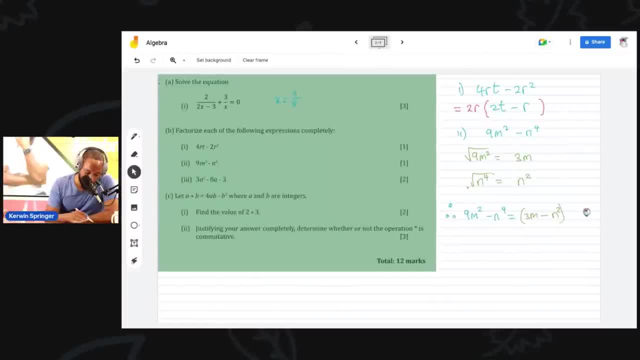 Pull this, pull this back a little bit. All right, so now we have 3m plus n squared. Yeah, we good there. So what do you think You can do them questions? I'm kind of taking my time and explaining each one. 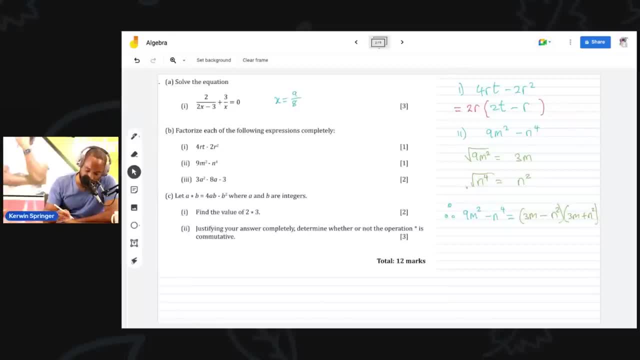 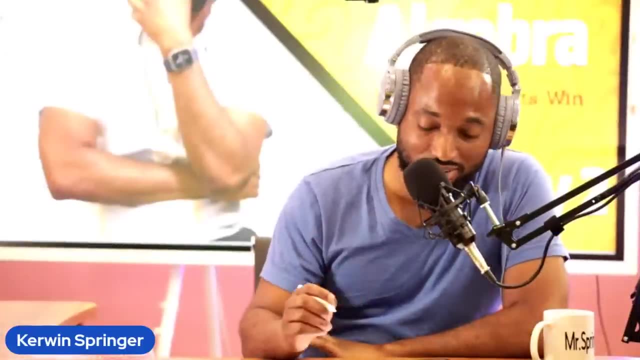 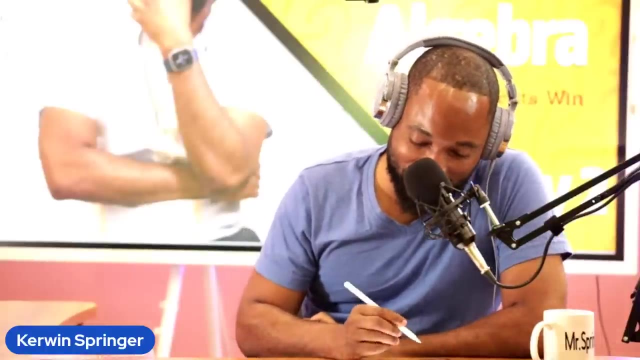 I'm not going super fast. We'll see how much of this we can get done today. I have a kind of deadline here because the engine is going to be some hundred feet in here. So, all right, the last one. What's the last one? 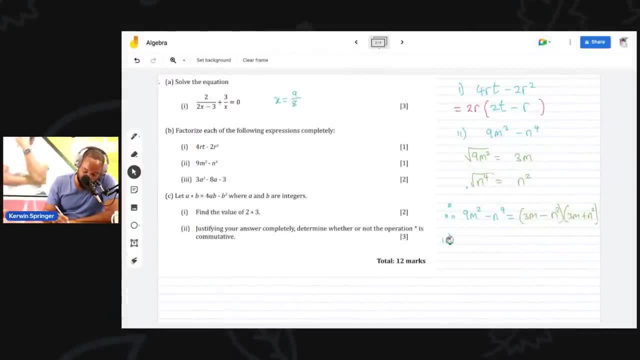 The last one is clearly a quadratic. Clearly that's a quadratic. It's using a, though, instead of x, And with quadratics we use the AC method, where we say: we want two numbers that will multiply, And you can look up my video on this on YouTube. 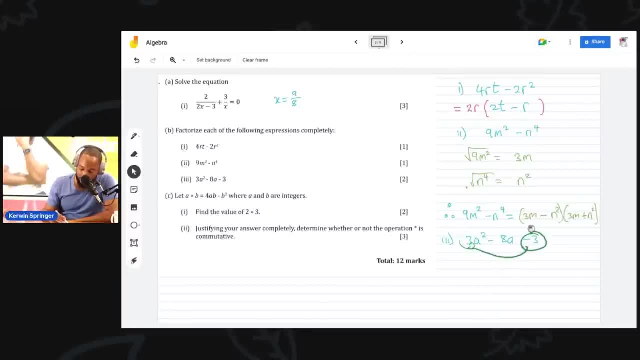 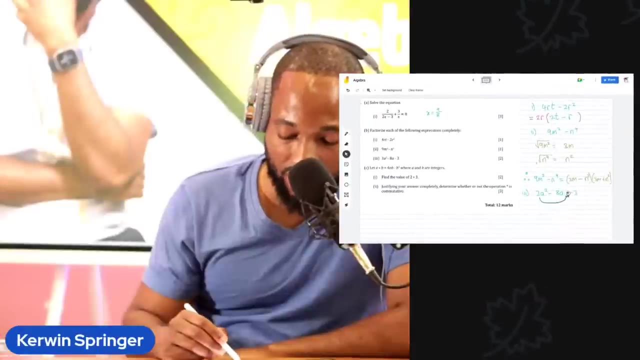 Two numbers that will multiply to give us a by c, So 3 by negative, 3 is negative 9. But the numbers should Should also add to give us negative 8.. And so immediately I begin thinking of the factors of negative 9.. 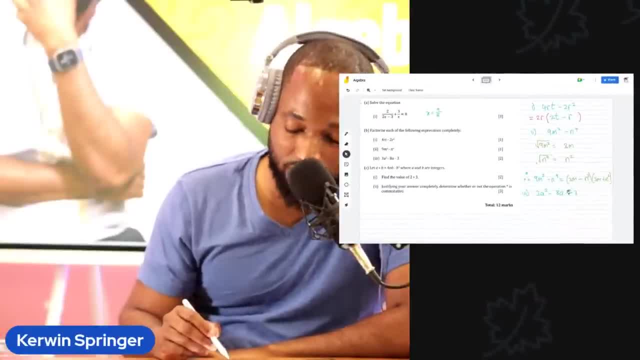 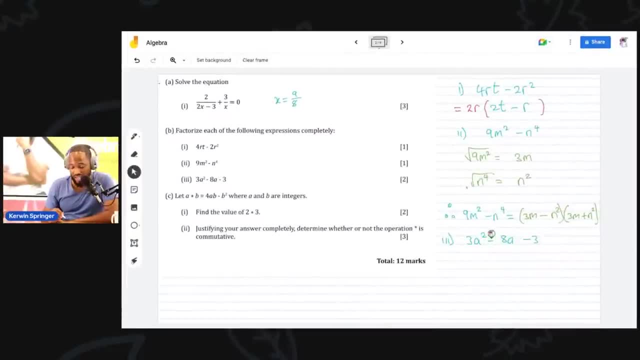 3 by negative, 3 is negative 9.. The factors are 3 by 3 or 9 by 1.. And I need to get an arrangement that will give me negative 8.. So an arrangement that will give me negative 8 is negative 9 and 1.. 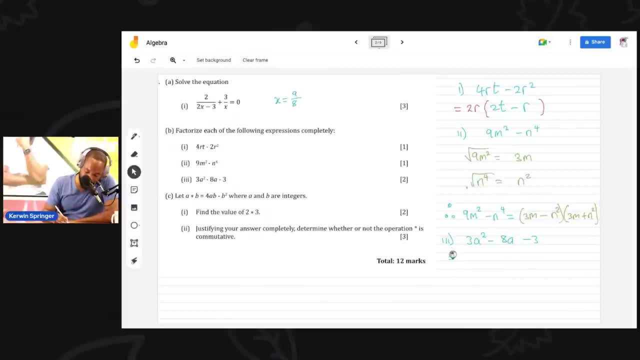 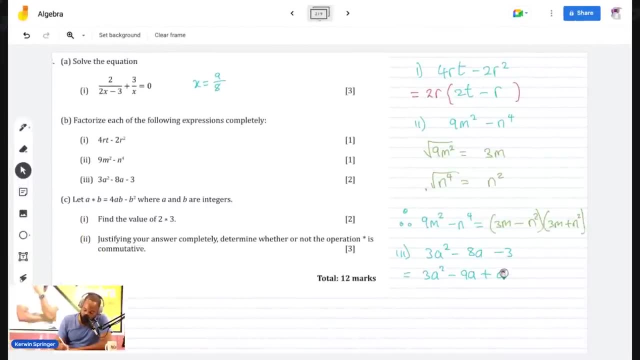 Seen it, It takes a lot of skill to Initially to get the hang of quadratics, And then when you have it, you're unstoppable. So that's, That's the intermediate line there, And then you factorize 3a. 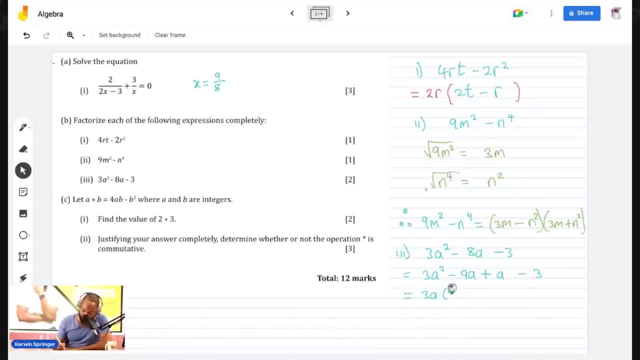 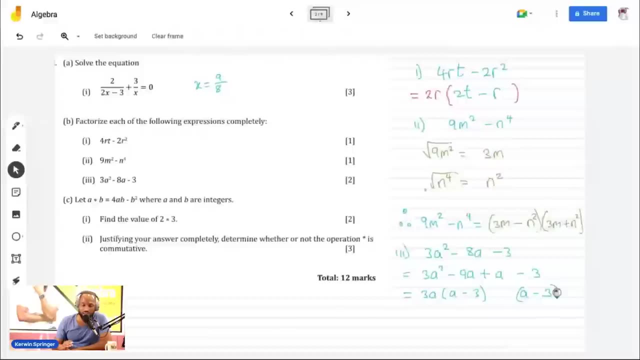 I don't want to take my time and explain this quadratic thing. If you're struggling with quadratic, please watch my videos on quadratics. It will help you from zero. If you need to take it from zero, you'll watch it and you'll understand. 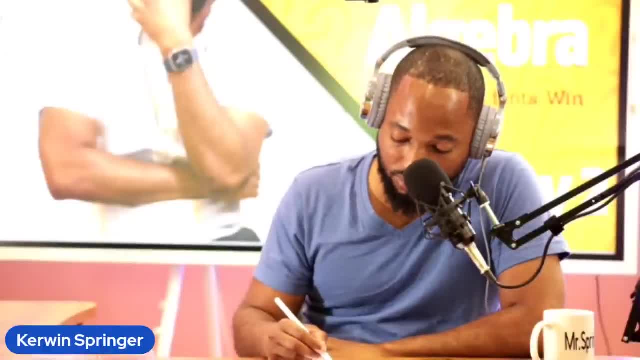 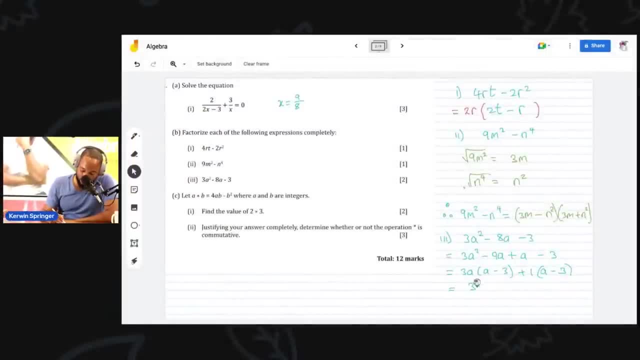 I think it's my most watched video on YouTube actually. So what happened in here? Once you factorize, you take that and you put it back there one time And then you just join this: 3a plus 1.. 1 and a minus 3.. 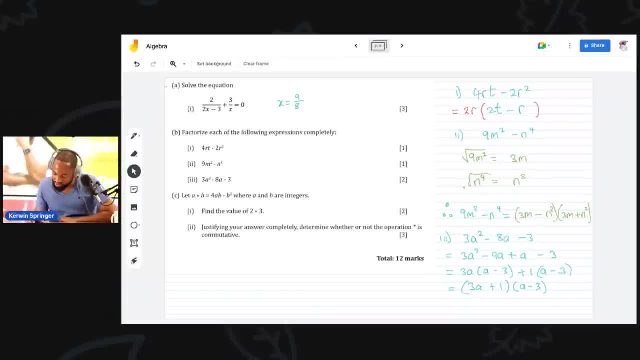 How are we looking? 3 plus 1, a minus 3.. You have to get a long time tomorrow, Jason. all of them cooking it around. So we just knock off one mark, one mark, two marks. Why this thing moving? 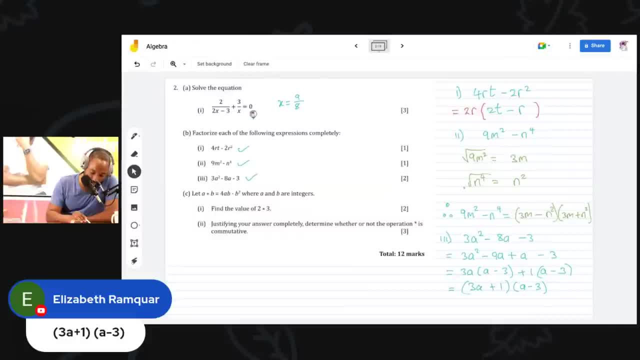 Why I never tell you to move. And three marks from before. here too, Three marks. what is this boy? Or how did you fill sample where this is 12 marks? It's not 12 marks these days, eh, So be careful. 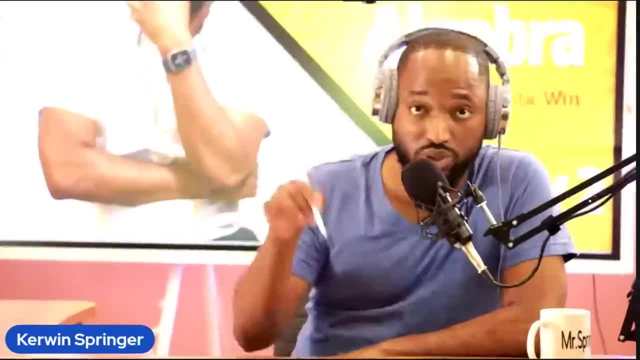 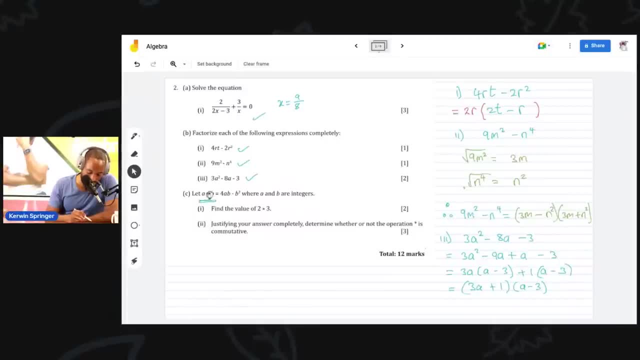 All right, Nine marks. Nine marks for the entire question. These question twos will be out of nine marks. So what is this called? This topic here is called binary operators, bro, Binary operators. Did you know that topic? And that topic is just basically fancy substitution. 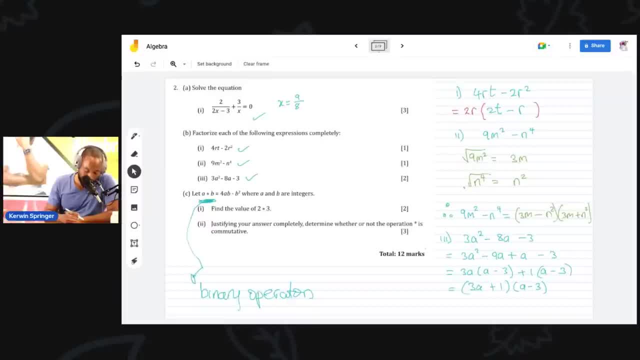 Yeah, so I bust my lips. It's kind of hard to talk right now, but the math must go on. So, binary operators: How do we do binary Binary operators? I'm telling you, it's just fancy substitution, but it will let them hot up your head. 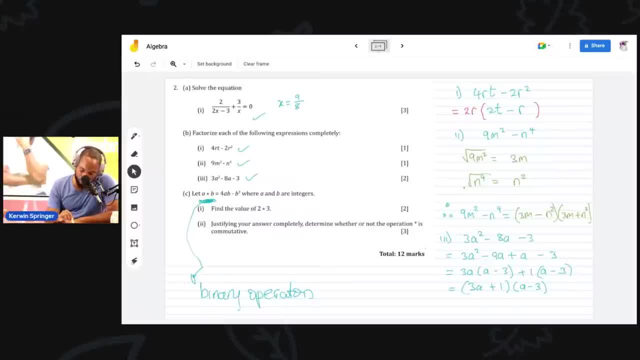 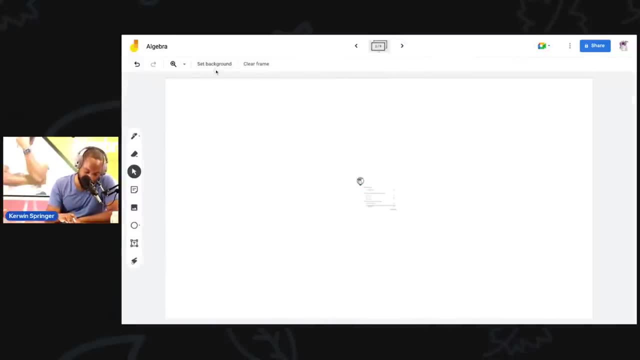 So let me pull back in the page two. Let me go back to page two now. I'll just pull this binary operators part And let me just knock this off. So hit them the lines there So you see the binary operation here. 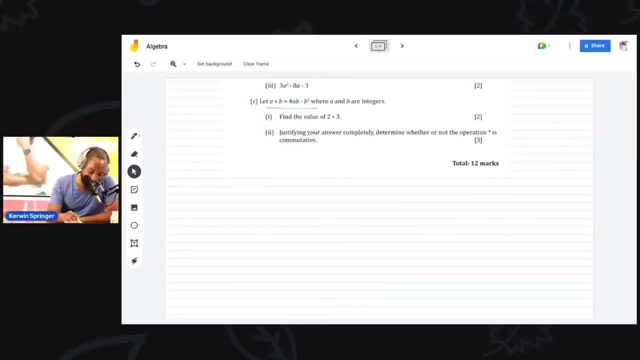 As I said, it's just, it's simply some kind of fancy. It's simply fancy, Fancy substitution. You're seeing it a bit true there. All right, So fancy substitution. So we have A star B equal 4AB minus B squared. 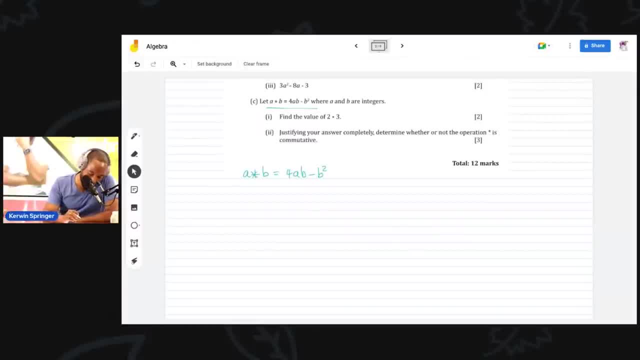 Hold on, I'm not seeing the lines on my screen, My realizer. Oh yeah, there it is. There it is. A star B is equal to 4AB minus B squared, And now they want us to find the value of 2 star 3.. 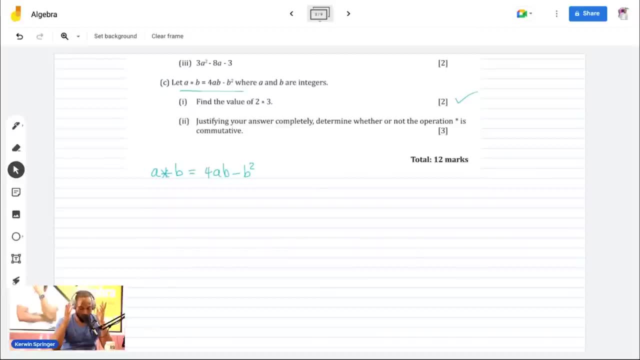 So stay with me, Stay with me, Stay with me. So A star B is equal to 4.. It's kind of telling you what to do. This is: the 2 is in the position of the A And the 3 is in the position of the B. 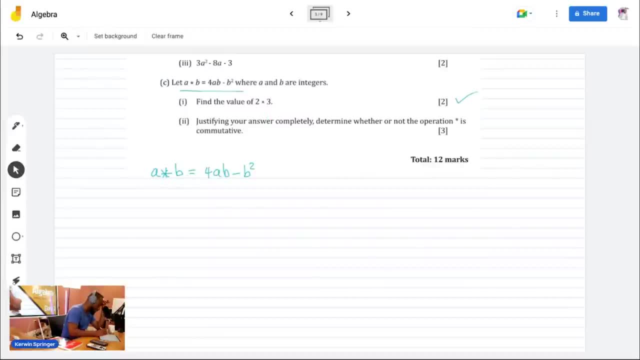 So it's telling you who to substitute. So, in other words, what's this next line I'm going to put here? This next line might explain what happened: 2 star 3 is really 4 by 2.. Instead of putting A as substitute. 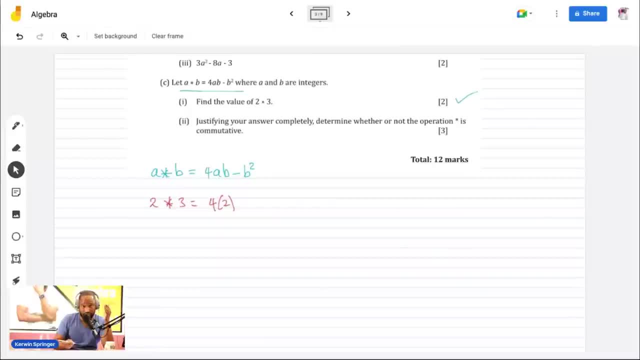 Binary operation, Binary operators, is fancy substitution, And I like how they ask this question, Because they bring this every now and then. The next part. now, What's the next part, Dave? For those of you who figured it out already, You all understand the substitution. 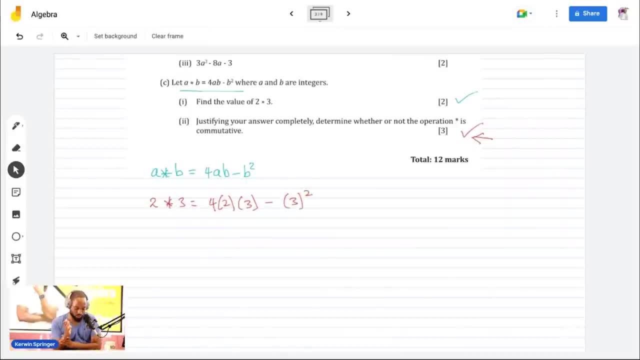 Why is it? each had to be a catchy substitution, So I replace all the A's with 2.. It was only one A, And I replace all the B's with 3.. According to the information given here, And now I just work it out, you know. 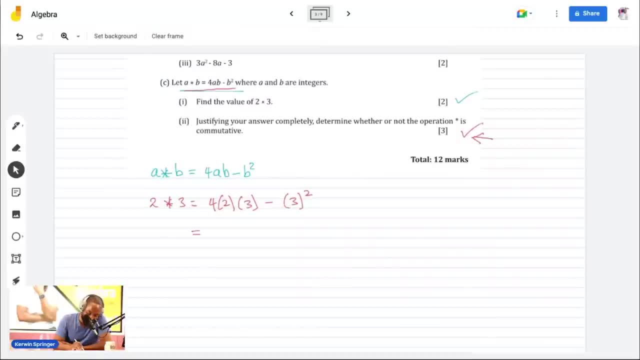 I'm only getting 15.. So let me try and make sure I get 15.. 4 by 6 is 20. 24. 24 minus 9 is hopefully 15.. So 15 is the answer And you get 2 marks for that. 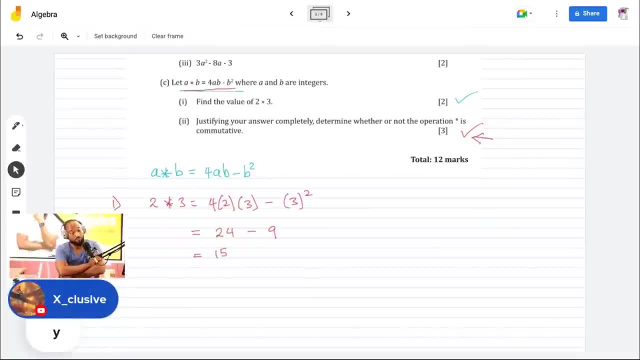 And usually you do get 2 marks for these fancy substitution binary operators. I find that's fantastic. And then the next part is something that I ask every now and then, And I want you to learn how to do this. You see how they're bringing this with commutative. 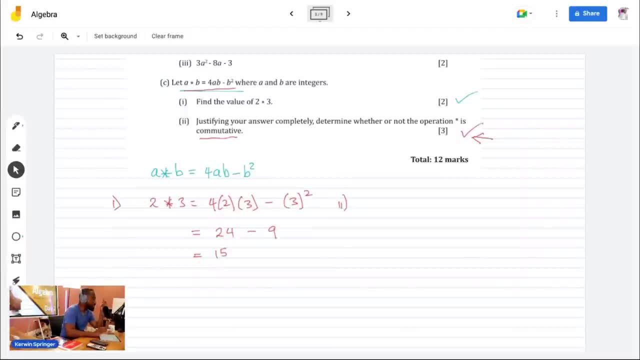 You all know the three operative laws, The three main operative laws: Associative law, Commutative law, Distributive law. This is how they're bringing the commutative law, And the commutative law is an operation that can do this. 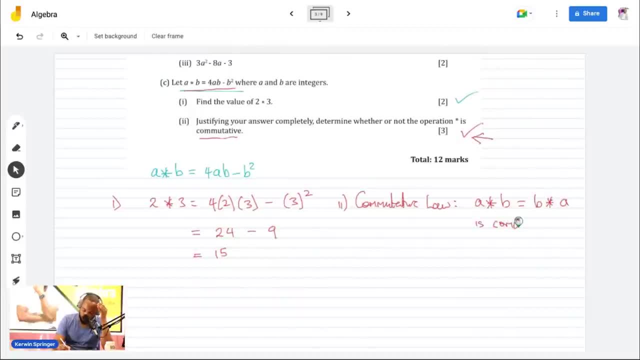 Is commutative If it can do that. So the commutative law is saying that if you could change it around, it's commutative. So the commutative The fastest way to justify this in the exam. they could actually do a whole proof, which 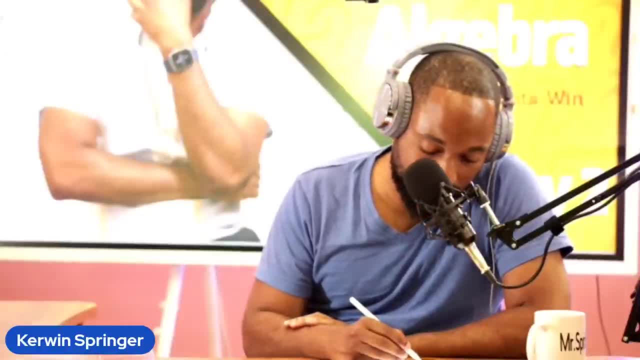 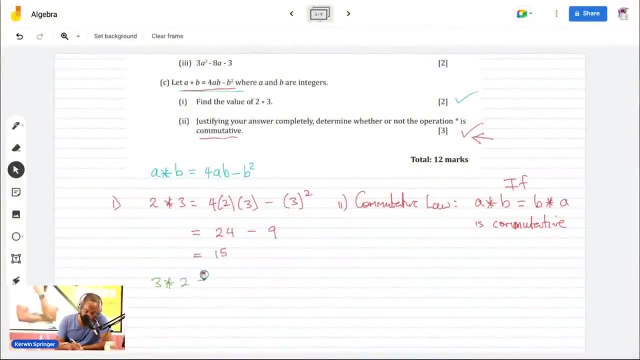 is not what they will be testing you on. The fastest way to justify this is to switch it around. So let me hit the switch around and see what will happen. If I say 3, star 2. Now the A is 3.. 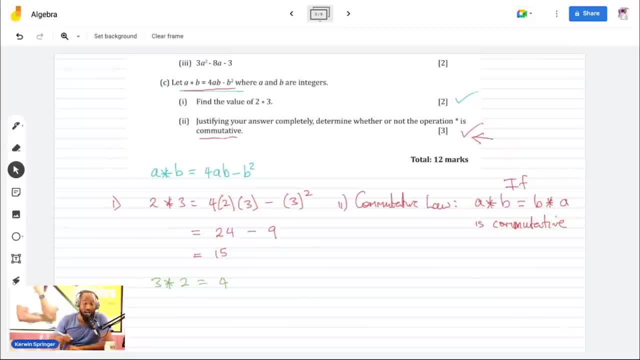 Instead of the A being 2 like before, the A is 3. And the B is the 2.. So I'm switching it around to see if I'll get the same 15.. Because if I get the same 15, it means it's commutative. 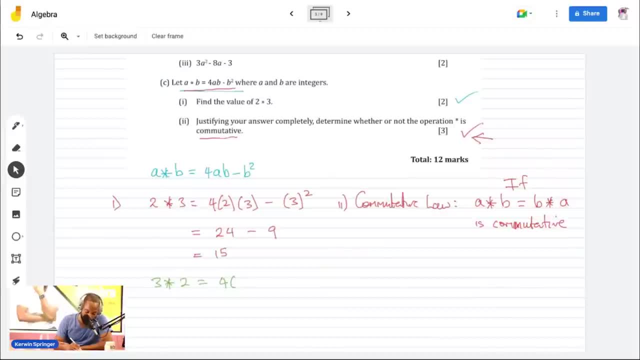 And I won't Most of the times I don't. So 3, 2, minus 2 squared, And how much do you get with this? How much do you all get with this? 4 by 3 is 12, by 2 is 24.. 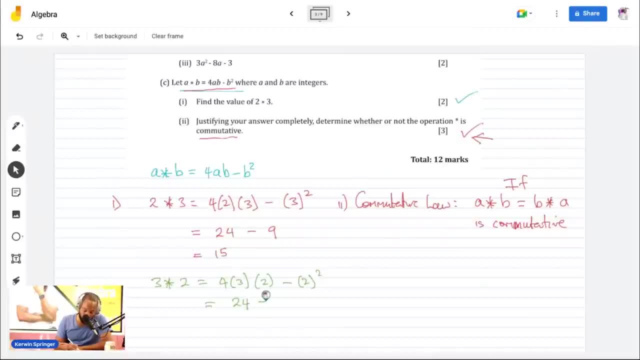 But this time I'm subtracting just 4. I'm getting 20.. Right, So 2 star 3 is equal to 15. But 3 star 2 is equal to 20. Therefore, this is not commutative. 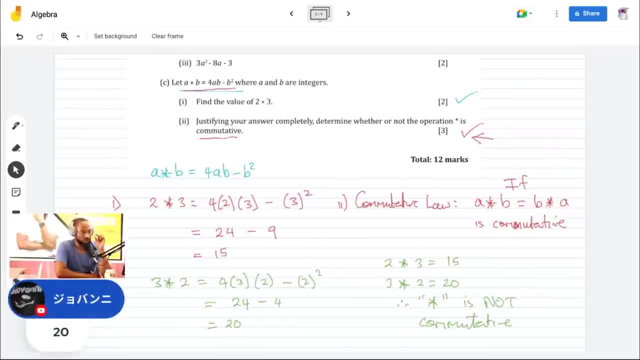 So it's easy to prove if something is not commutative, If you could find a case that shows that it's not commutative By showing that yo I used 2 and 3 and I switched it around and it didn't work out. 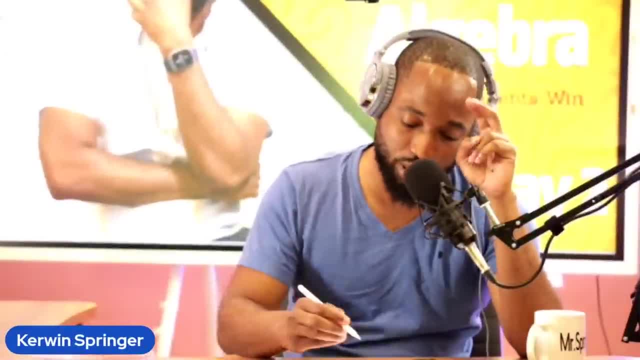 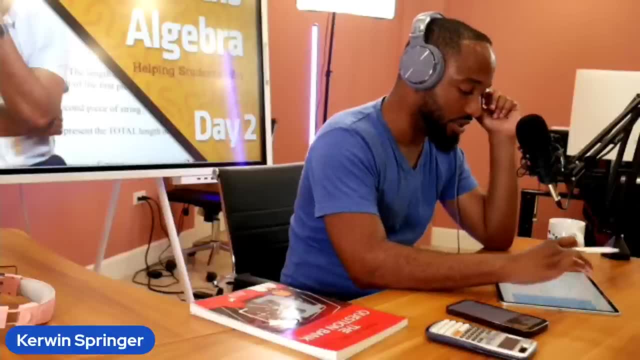 You prove it. Understand how to do that, Because you could see it. You normally put this for 2 marks. now It will keep you. It will hold on at 2 marks during the exam. Let me do our next question. How much of these algebra questions do you want to do, boy? 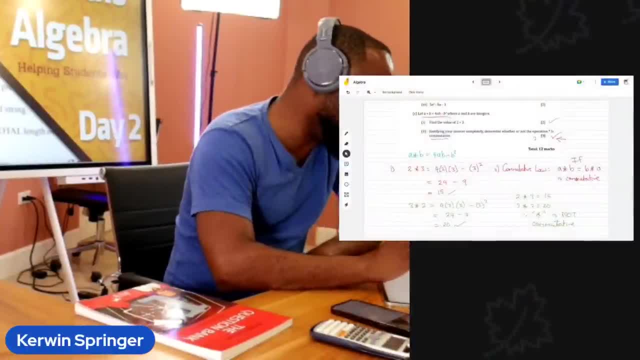 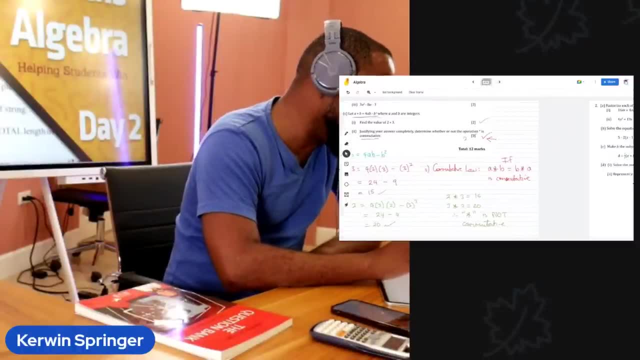 Let me read them. My next one: Factorize each of the following expressions completely. So more factorization at the start of algebra On page 4 here 16m plus 4m squared. So what is it looking like? 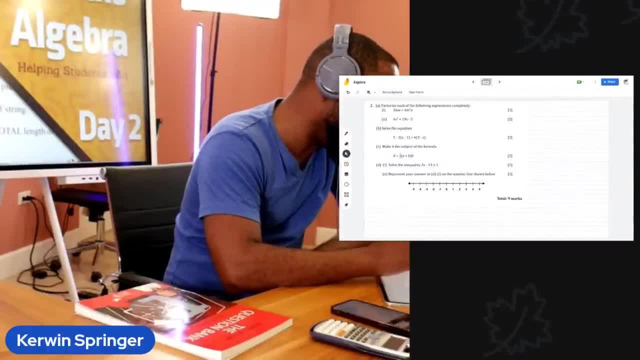 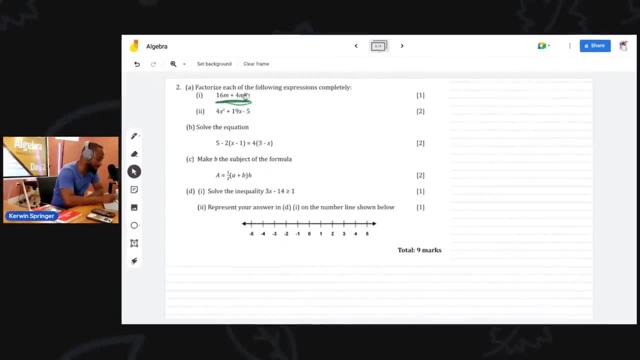 What type of factorization do you all think we're going to do for this? You're talking about 3 die here. What type of factorization do you think we're going to do for this one? What type of factorization Basic? 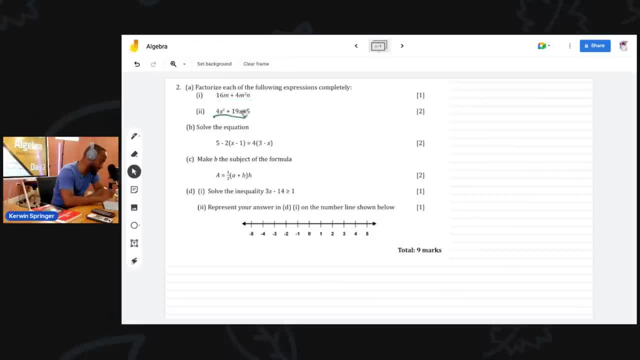 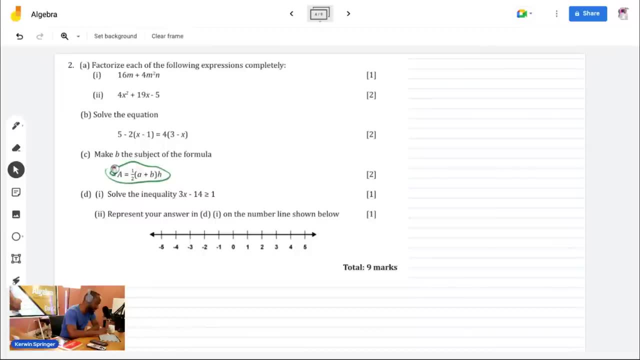 What about this one? What type of factorization are you feeling here? And then we need to solve, Then we need to do a transposition. So this is linear equations. I'm giving you all the topics every time. So linear equations. 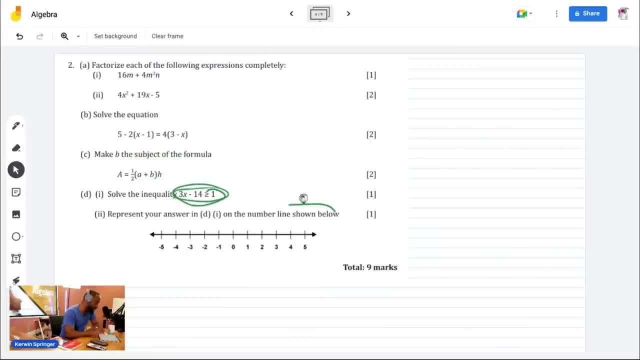 Then transposition, or subject of the formula, Then inequalities with a number line, Which has been very popular these few years. So there you go. This first one Is basic factorization. Why? Because all I'm seeing the m squared. 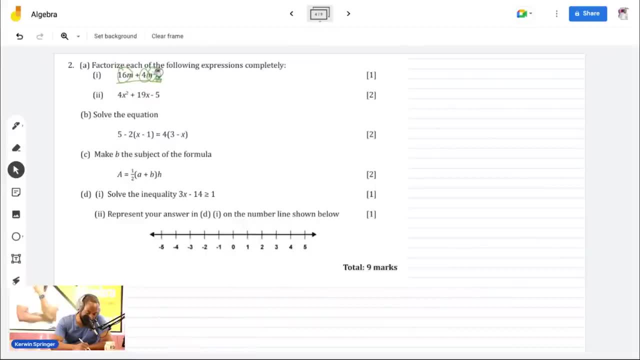 All I'm seeing square numbers. I am seeing a, n. What are n doing then? I'm messing it up. It has two variables, So I can only start off with basic factorization, And maybe sometimes there's a nested something inside there. 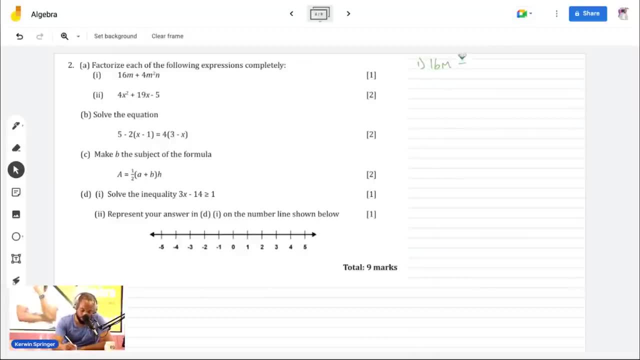 So let's see what happens for part 1.. I'm writing part 1 here And then I'm going to pull out what is common. I ask myself what is common? First question: I'm seeing 4 can come out of both of these terms. 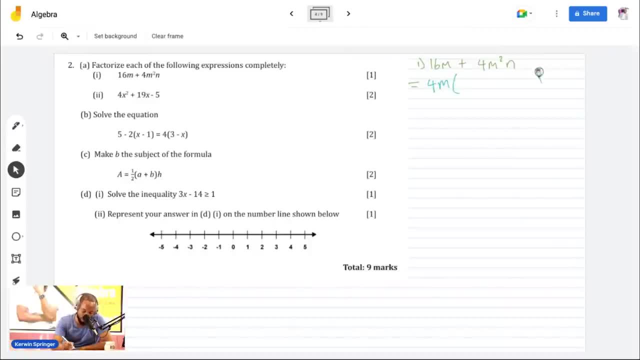 And in terms of letters, an m could come out. And now I'm going to put back what is missing. For the individual terms. I'm seeing 4 is missing Because 4m by 4 is 16m, Right. 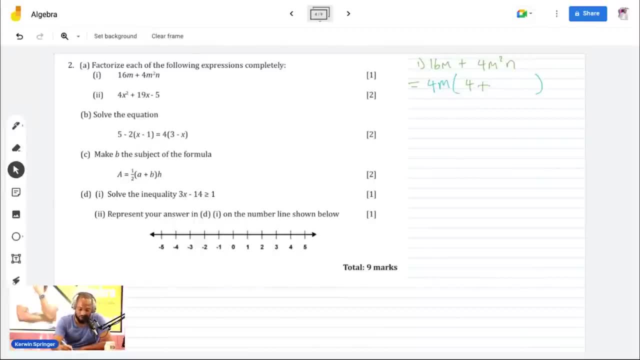 And then what is missing for the next term? We already have the 4. But we're missing one of the m's and the n, And that's it: Basic factorization. You're done, One mark. It will always be one mark. 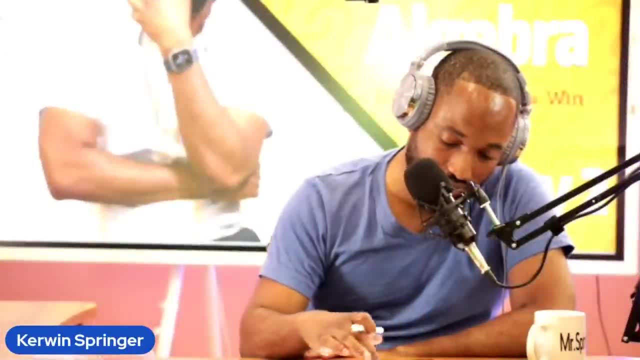 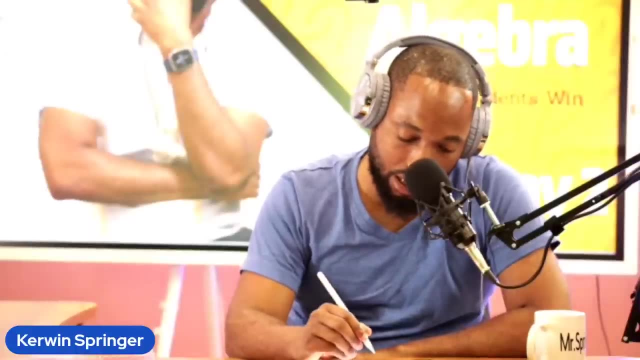 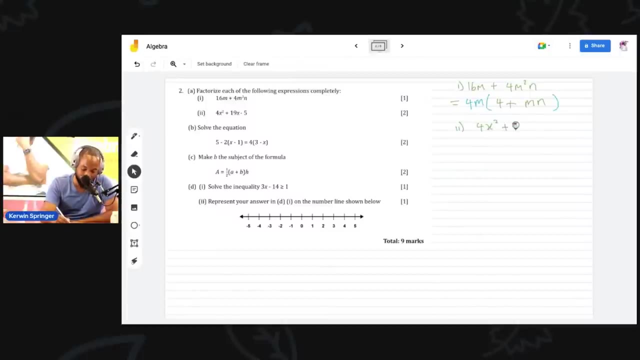 Unless it's like a really long kind of expansive thing. How was that? You all understand everything so far. How are we doing So? part 2. This is clearly a quadratic. It's even written in the quadratic format. So once again, we're going to use the popular AC method. 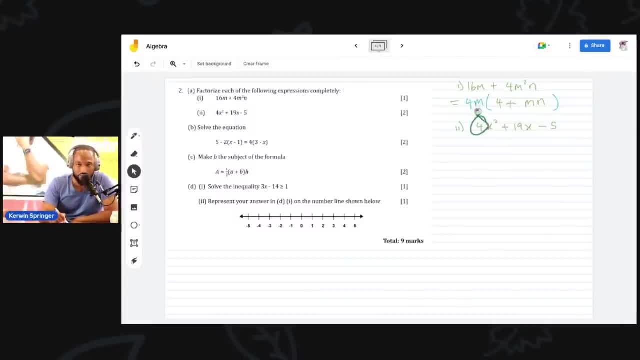 4 by 5.. 4 by 5. Or 4 by negative, 5 to be exact, Negative 20.. So two numbers that will add to give me 19.. But multiply to give me negative 20.. Now when the number is really close to the number that I want to get, 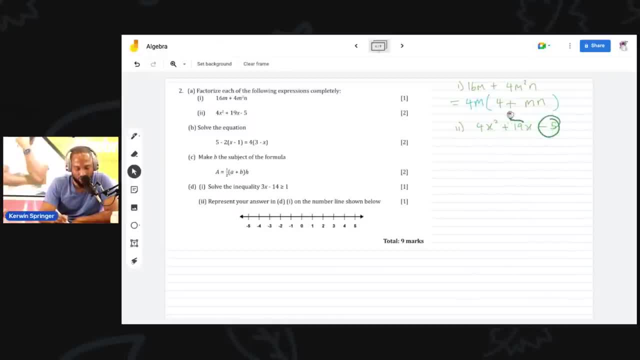 4 by 5 is 20.. 19 is really close. I usually know it has to be the number plus 1. Number and 1. And in this case I want the 20 to be positive, So that the number here would be positive. 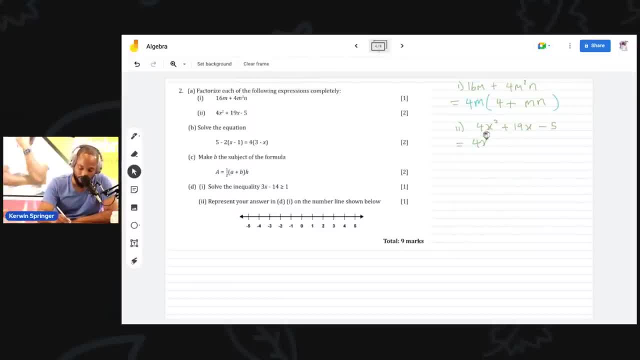 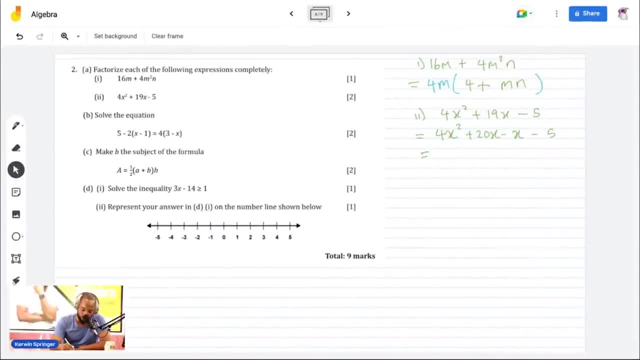 Right, Revise your quadratics if you don't know what's happening here. So I'm going to put 20x minus x minus 5. And then I'm going to do some. This is factorizing Four terms, aka grouping. 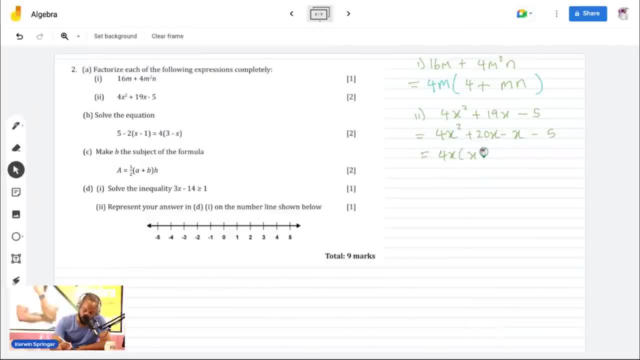 4x into x plus 5.. So I'm going to put x plus 5 here And I'll pay it back one time. And to make this possible, What I'll do is just put a negative 1 here. Negative 1 by this would create back that. 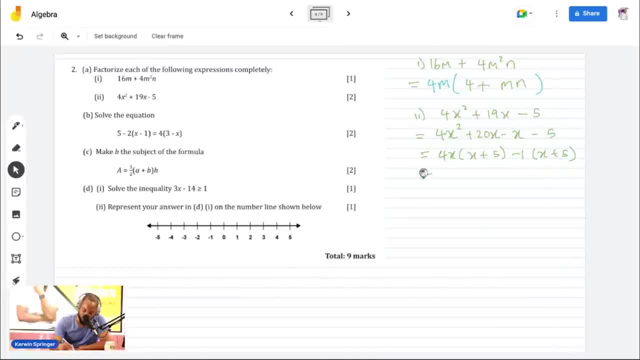 Right Group up: 4x minus 1 equals x plus 5.. That's how it works And we won't ask to solve. So we just factorize. And I'm seeing a whole bunch of people: Hey, we reached 300 by. 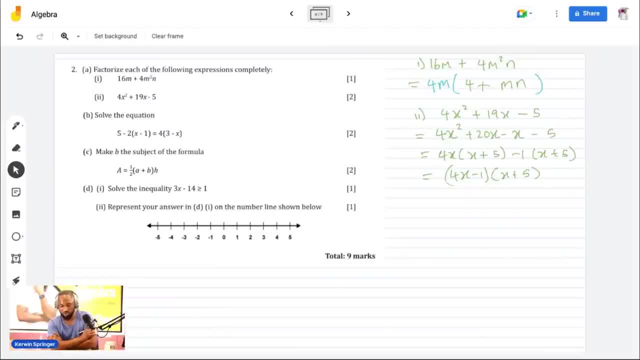 A whole bunch of people on this show. So make up yourself Part B now. So that's part A. Let me see if I can squeeze in part B right here. Make who the subject of the formula. Make B The subject of the formula. 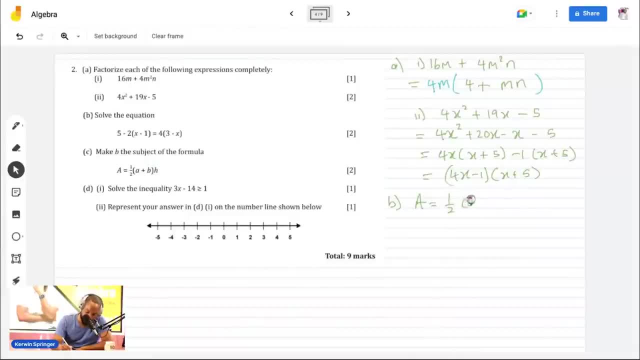 So A is equal to half A plus B, H. You want to make who The subject of the formula, So you want to get across everything that is not B onto one side. So H is not B. Let me get. 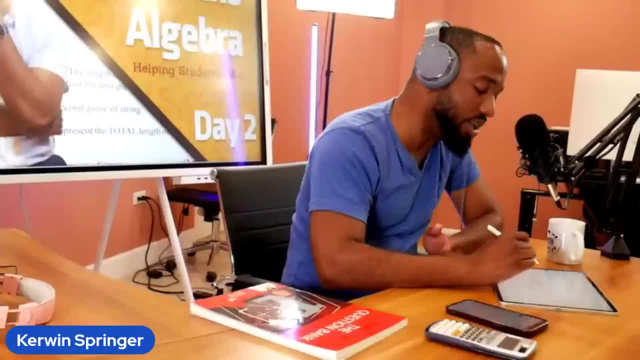 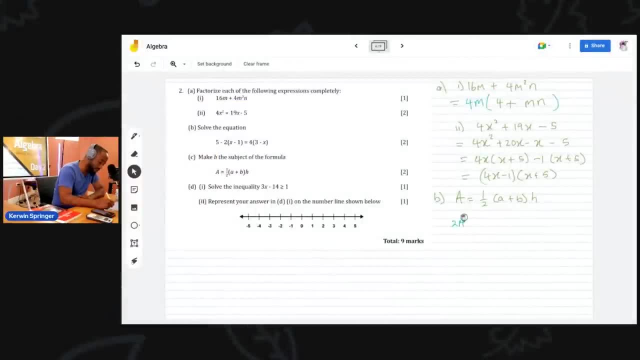 What's the first thing to get across? The half and the H could take a hike. So if I bring, If I multiply everything by 2, then If I multiply everything by 2. I'll have 2A And the half will disappear. 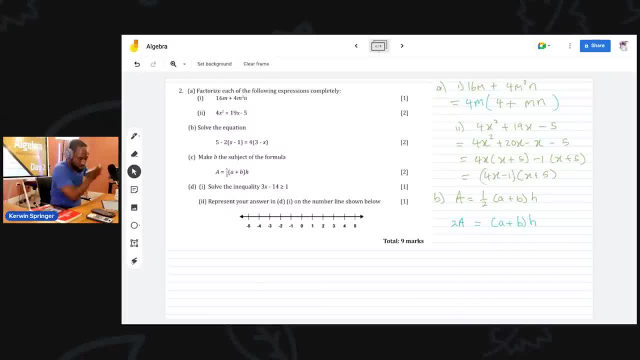 So I do it step by step. I could do this way faster, But I want to make sure you follow everything, Or multiply everything by 2. Whatever you want to think of it, I just get rid of this half and bring it onto the next side. 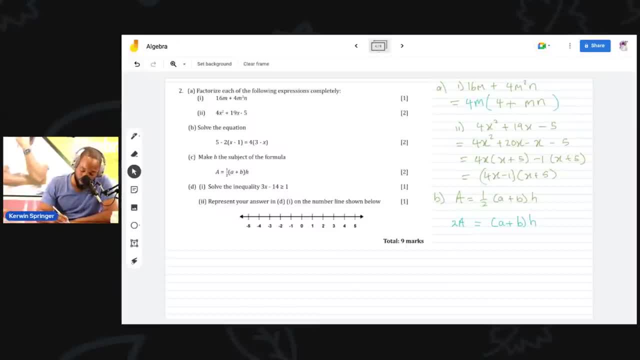 If it wasn't division on that side, When I come across it into multiplication Then I'm going to bring across the H, So I have 2A over H Because it's the B I want. by himself I couldn't bring across the. 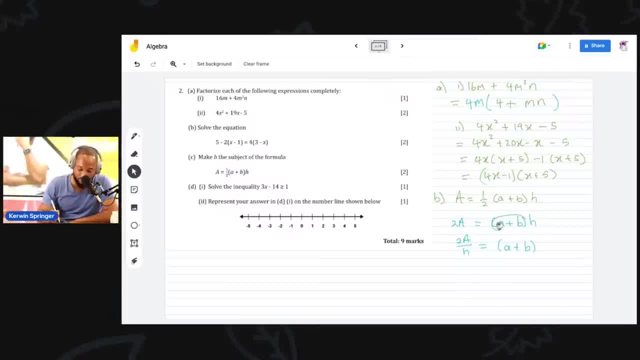 I couldn't bring across the A yet Because the A trapped inside the parentheses, Inside the brackets, So I couldn't touch that A. So 2A over H And you have A plus B And 2B on that side. 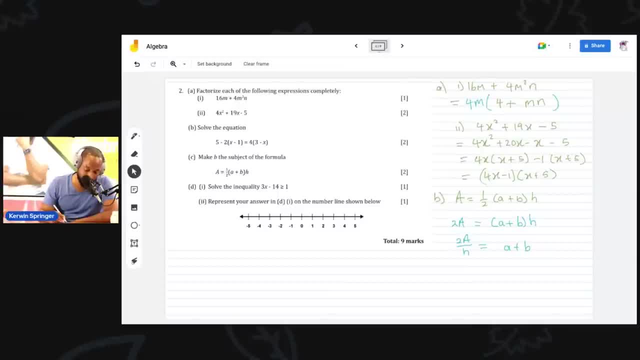 It's fair for me to just drop the brackets there now. So now, what's left to do? Just to bring across the. Just to bring across. Oh, I forget to do part B. Alright, thanks, people, I'll swing back to part B just now. 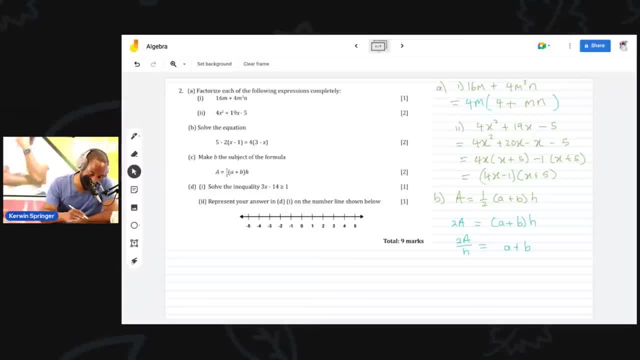 So just bring across the B, Put the answer for C, Or maybe we have to tell C to wait. Wait for me there, C. Wait for me there by C. I'm going to go and do B. No, no, no. 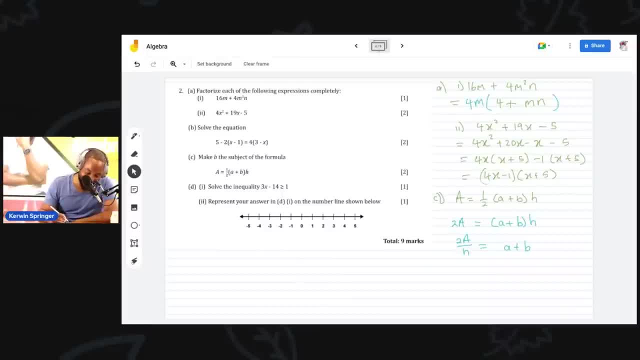 We finished C now. We finished C now The indecisiveness boy. So we're going to make B the subject of the formula. So 2A over H minus A is equal to B. I can write it this way: 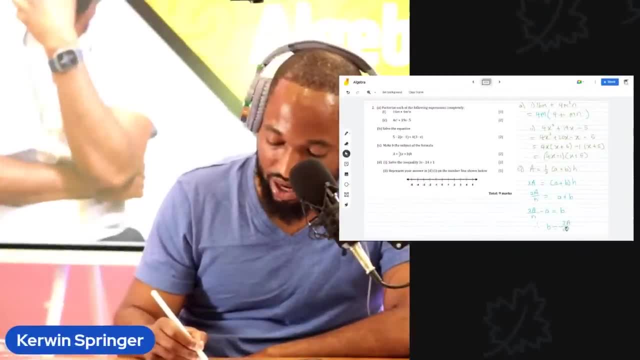 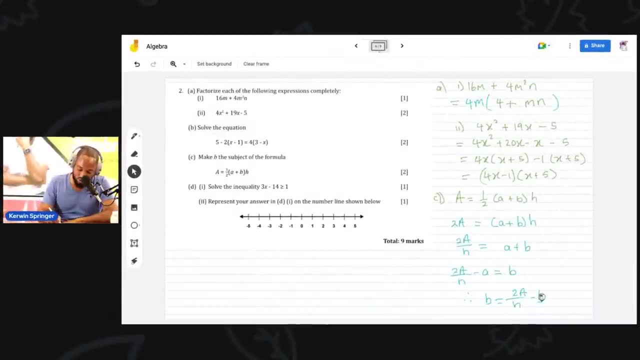 For those of you who like it this way: 2A over H minus B, We can make our talk back, We can make our swing back. So 2A over H minus B And we're good to go. If you can't transpose in mathematics, 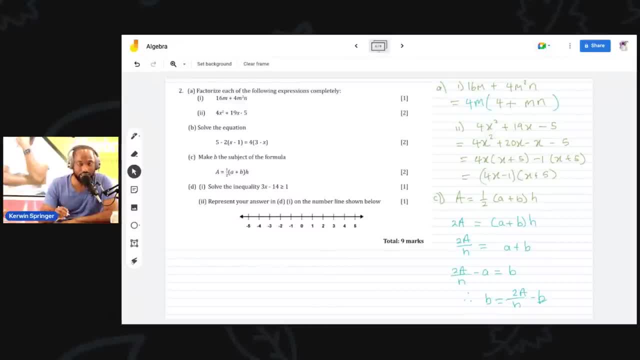 You will have a very bad time in the exam. You're going to come just straight up with L axis to transpose. There's so much formulas where you'll have a missing thing And you need to find it And you need to rearrange the equation. 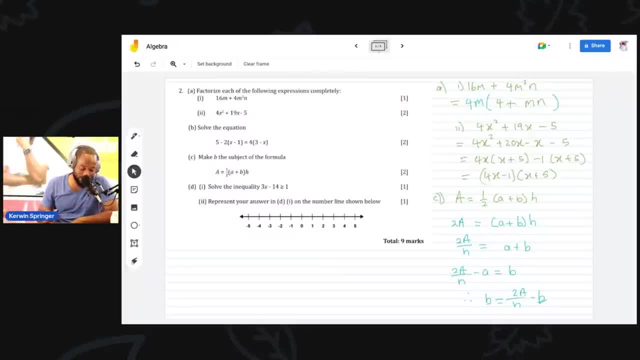 How much time will you rearrange an equation in mathematics? It must be a thousand times. since you start secondary school, You must know how to do that. So now you go and do the part B that we leave out, And then we can do part B. 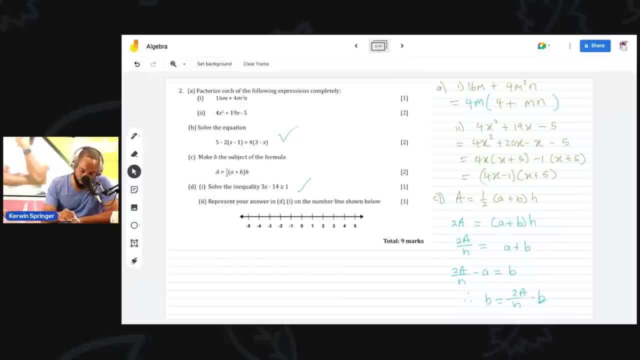 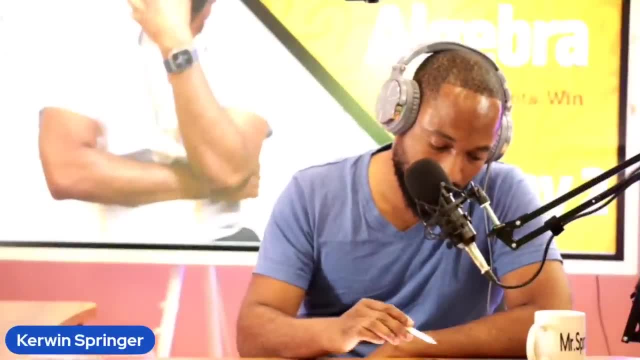 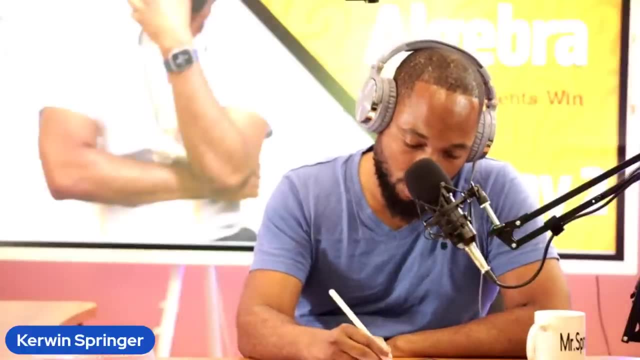 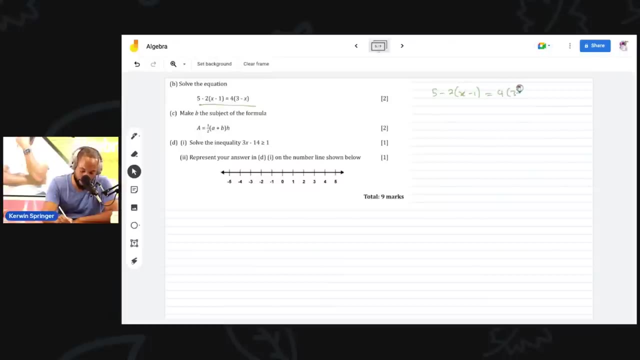 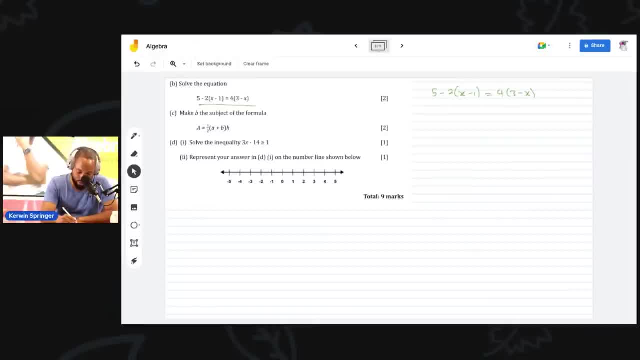 We have some distribution to do here, So it's going to be 5 negative 2X. And watch a common mistake here: When you have a negative sign with a number outside the bracket And you need to multiply the negative 1.. 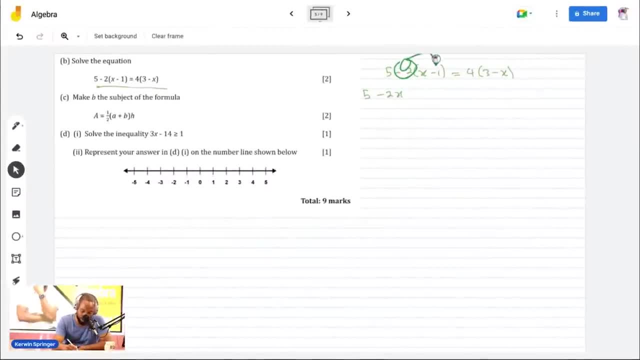 Keep that in mind. Two negatives make a negative. Positive 2 will be there, And this one is 4 by 3 is 12.. And then 4 by negative, X is negative, 4X. Why is any chat following you? 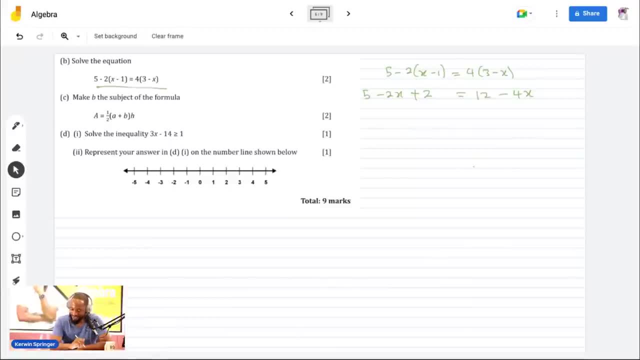 Have you seen it? Rearranging like we're doing interior design, Sanjay? how do you do it? All right, So what we really want to do when we're solving is: bring all the X's on one side, Bring all the numbers on one side. 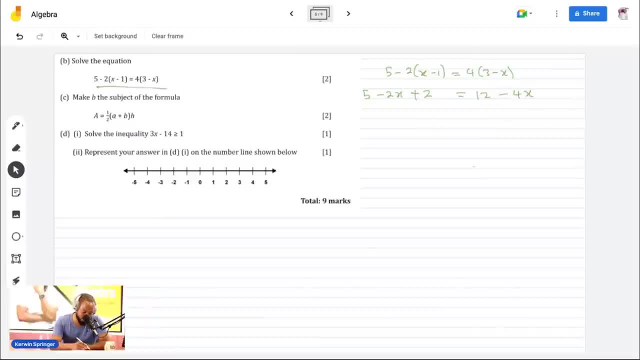 Bring all the X's on one side, Bring all the numbers on one side. We have negative 2X and negative 4X. Let's bring them to meet each other And at the same time. One time I'll bring across the 5 and bring across the 2.. 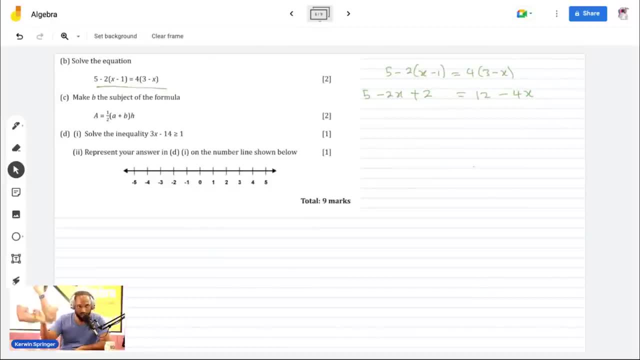 All we need to record is that we, If you're bringing it across, you're going to switch the operation. So the negative 2X stay in here, But coming to meet him is the negative 4X, But because it was negative there, it will switch to positive. 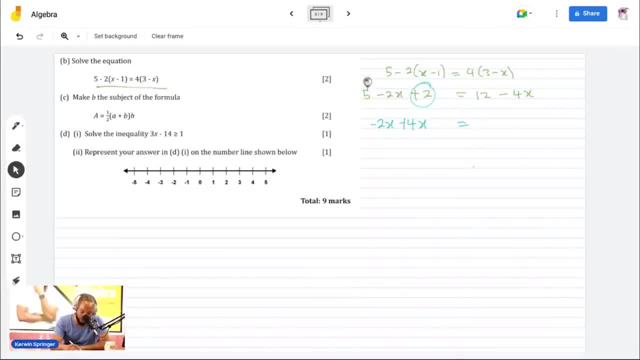 And then the 5 and the 2 are positive, Don't think the 5 negative. The 5 is positive. The 5 belongs to the term that comes after it. So it's really 12 minus 2.. And then minus 5 again. 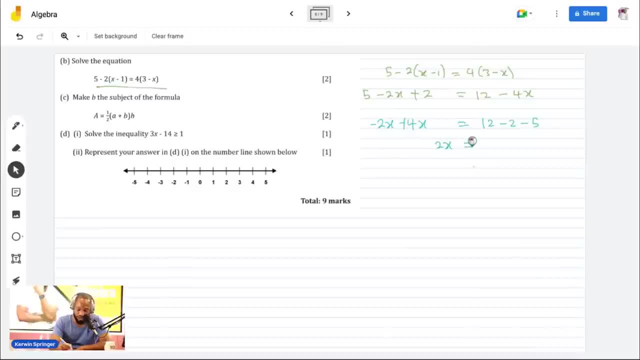 So negative 2X plus 4X is 2X And 12 minus 7 in all is 5.. So at the end of the day, X is equal to 5 divided by 2. And that's the answer, right there. 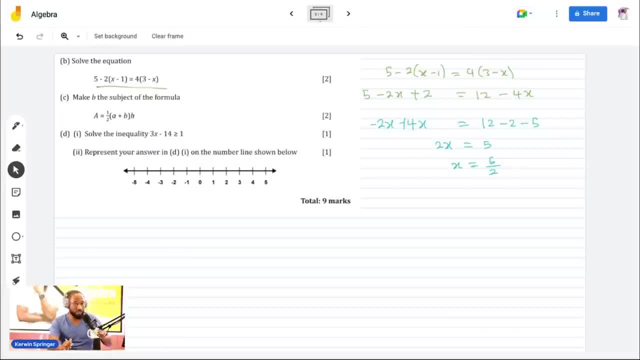 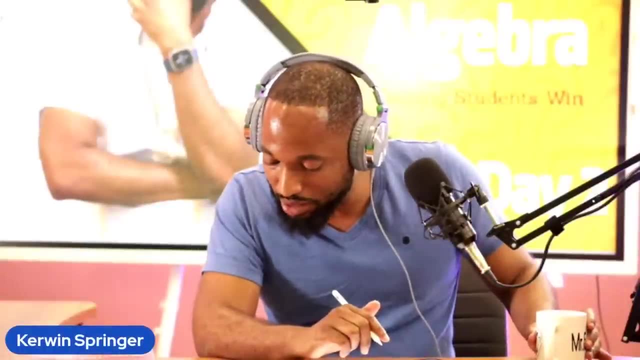 You don't need to change it to decimal. 5 over 2 is good enough. So that's 2 max. Why doesn't each other fully understand? So thank you for joining us. Thank you for getting my brother into Fatima. 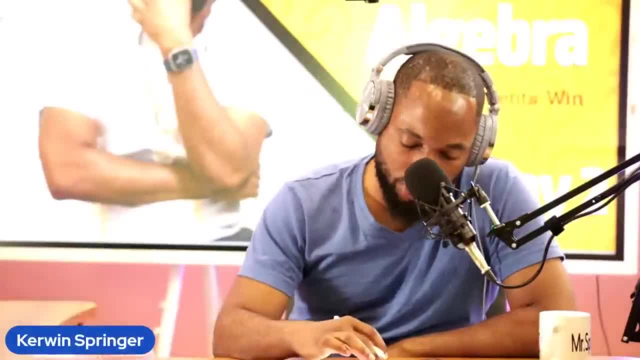 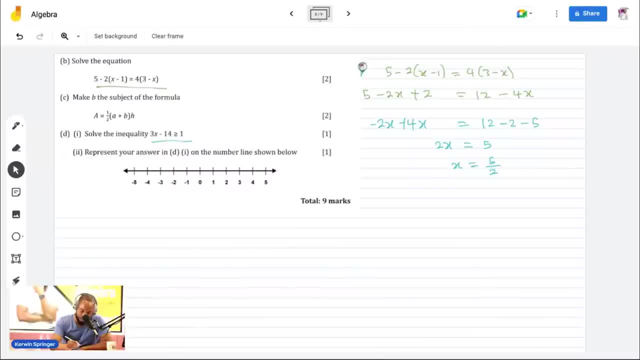 Big up your brother, big up yourself And you're welcome. So let me just finish off strong with this inequality. We need to solve the inequality. As soon as I see an inequality, I think about the most important thing to think about with inequalities in this question. 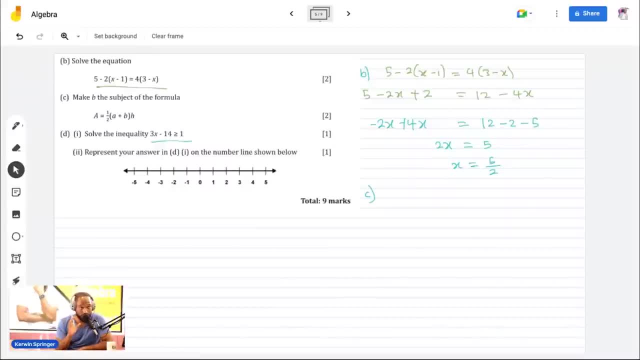 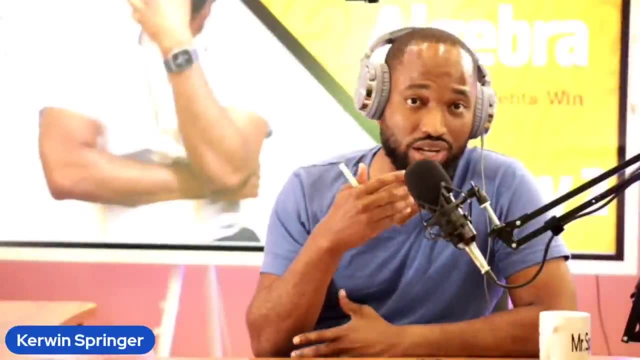 The trap cards I call it. If you swap both sides, or if you multiply or divide by a negative number, you have to flip the inequality sign, Otherwise you're going to get it wrong, my friend. So let me see if we're going to activate any trap cards. 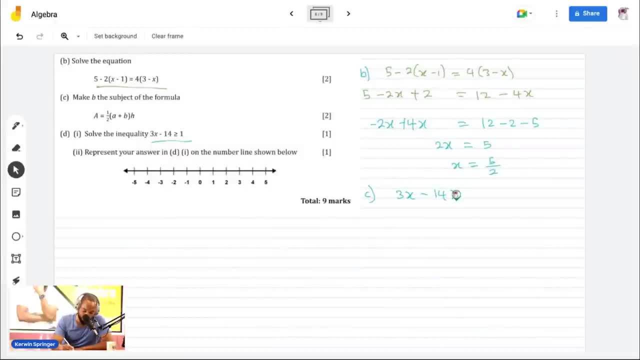 3x minus 14.. Other than that, you're just working normal. So that's how we start off, And now we want to work it out, So we're going to bring across the negative 14.. That's not activating a trap card. 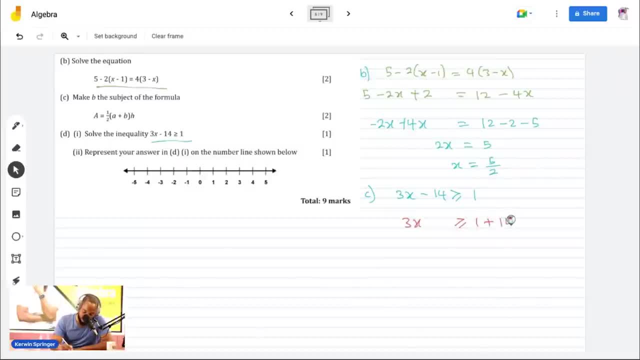 We're just bringing across numbers. We'll change to positive 14.. So you get it's greater than 5.. 3x is greater than 15.. Sorry, why did I say 5?? x is greater than 15 divided by 3.. 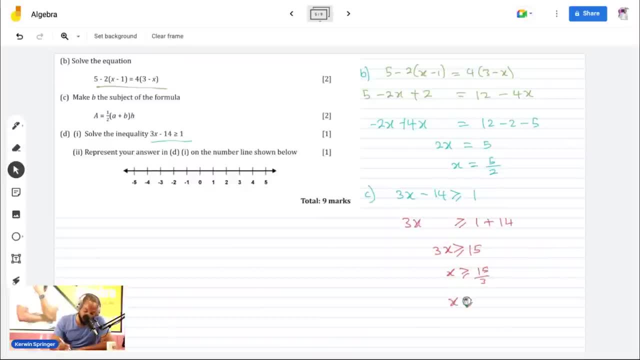 So x is greater than or equal to 5.. So now represent your answer on the number line shown below. What kind of weird number line is this? Because I'm supposed to say x is greater than or equal to 5.. 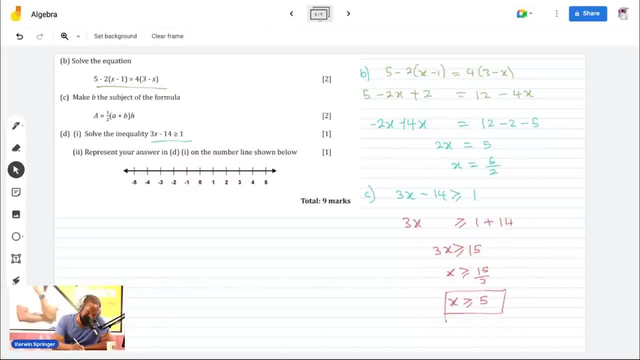 Add 5 right here, And what you're really supposed to do is draw a circle on the 5.. And since, If it was just x is greater than 5, that would leave the circle like that, But since it's greater than or equal to 5,, 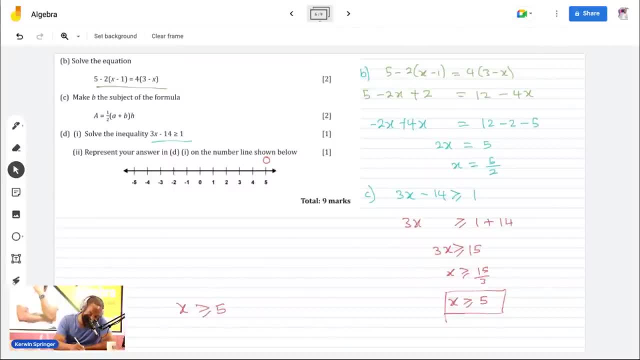 you need to shade in the circle Right And then you need to point in the direction this way, And that's how you collect your mark. Make sure you know how to do that. Another one? Yeah, man, Let me do our next one. 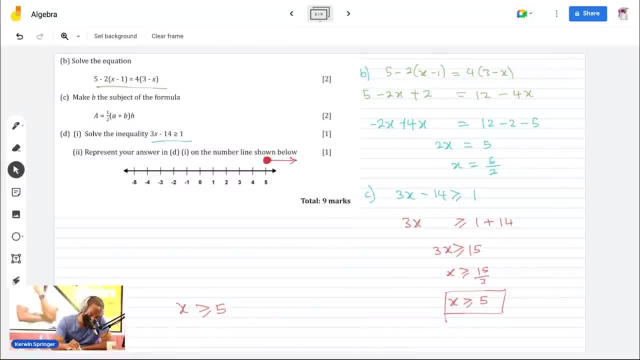 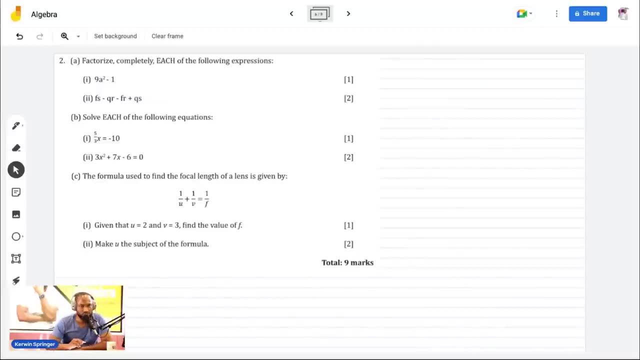 Let me do another one. On page 6, we have our next question here. Let's wind up. What type of factor is So the chances of you seeing a factorization Very high, And make sure you know how to do all of them. 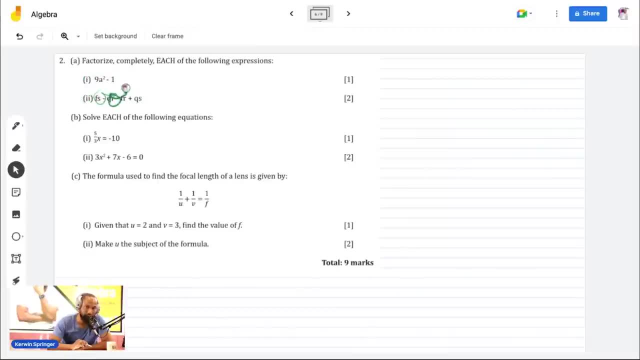 So this looks like 4 terms. From the time you see 4 terms, think about grouping. Most likely it is. We have a difference of 2 squares here, because 1 is a squared number, 9 is a squared number. 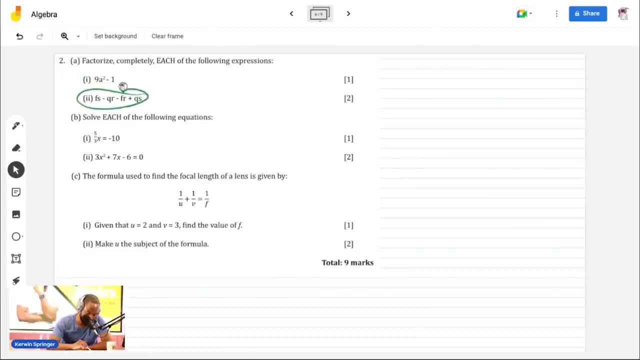 a squared And there's no extra term, It's just a. So if we solve a linear, then solve a quadratic, then we need to do what? A substitution, a substitution and a transposition- Classic, We're done. starting to see repeated ideas already. 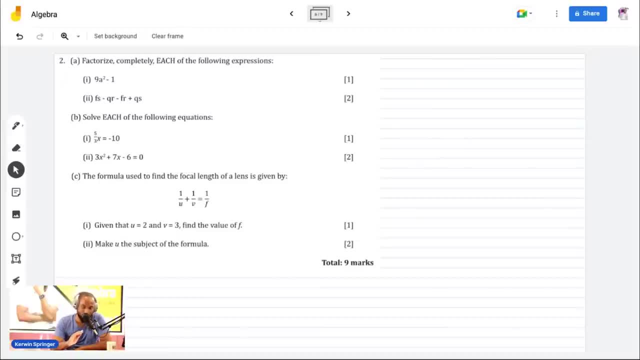 And I love that. So let me go. Let me see if I can fit all the answers in one page. Let me conserve the real estate here. So 1. 9e squared minus 1.. So you need to write out your answers for. 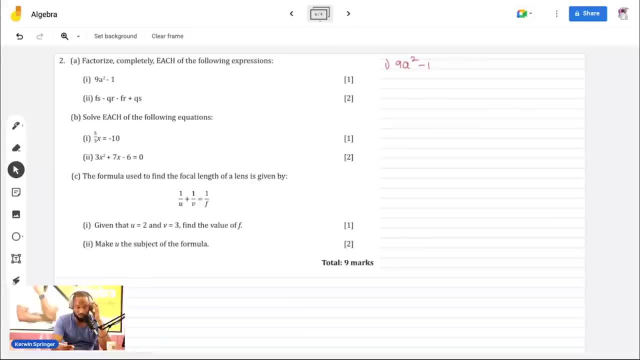 what do you call this thing? Difference of 2 squares? Right now we're working with this kind of technique where we get the square root of each of the terms, So that's 3e, And then the square root of 1. 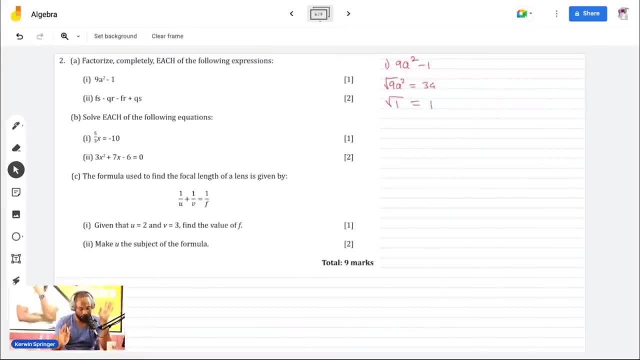 is 1.. Not the negative sign, Just humble it right now. And then you write: therefore, 9e squared minus 1 is equal to the square root of them, 3e minus 1.. 3e plus 1.. 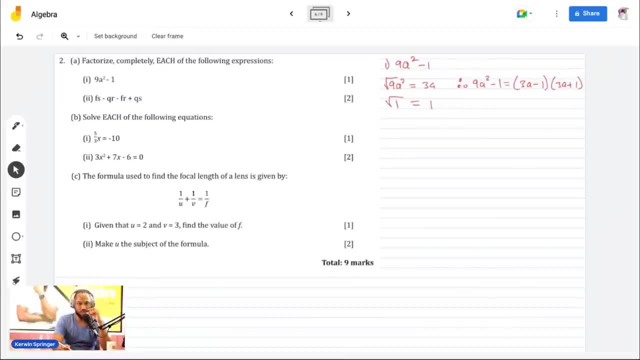 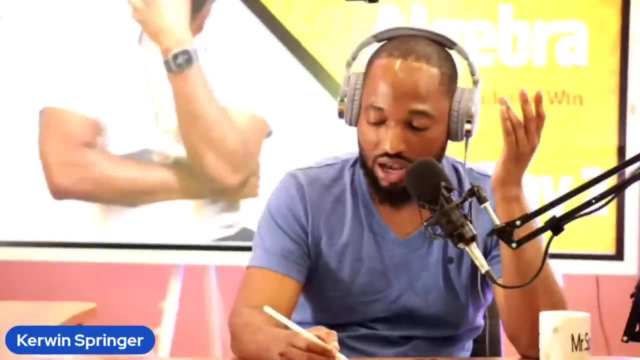 So if you want, you can look up a video I have on factorization where I show how to do the four types of factorization And you can get really good at it. and just hit your debug, You notice there's like four marks coming out all the time. 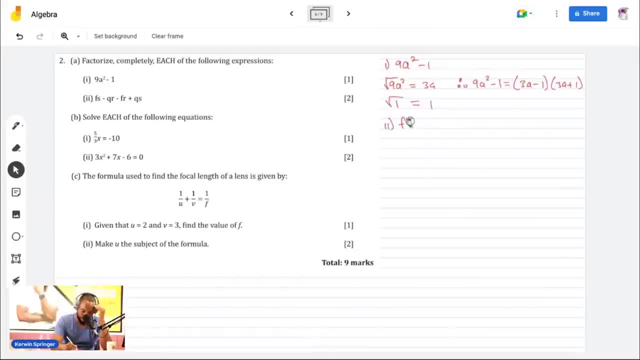 And fs minus qr minus fr plus qs. fs minus qr minus fr plus qs. Hmm, Well, this is four terms, Right? So normally you're supposed to pull out something common here. but there's nothing common there. But I see an f over here. 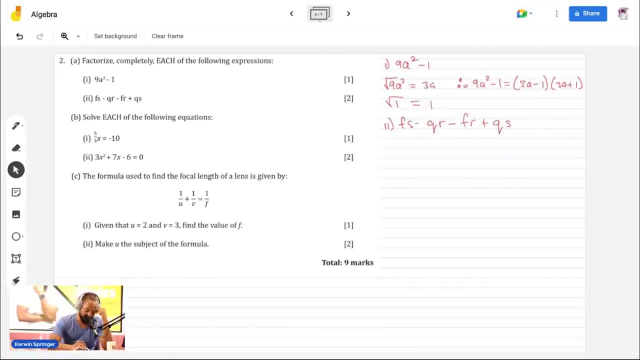 If I bring this here and then I bring the q there, I might get lucky. So let me just rearrange before You all understand what I'm going to do. I'm going to rearrange to see if I could get a little better setup here. 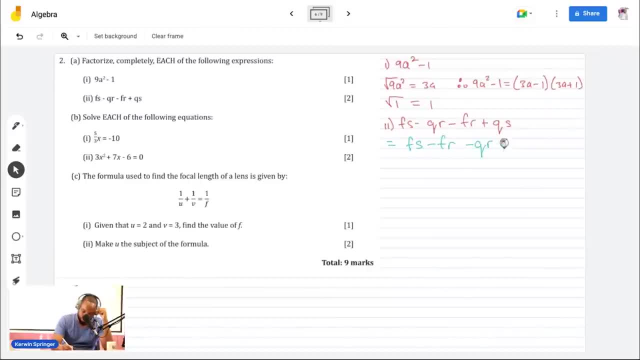 fs. I bring in the negative fr there. Negative qr could go there. I just swap the two terms there. I don't need to change the signs qs. And now, what is common When you're doing this four terms grouping thing? 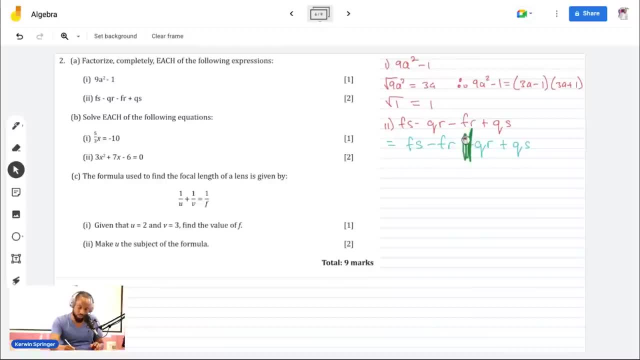 you have to imagine an invisible line here. So between the four terms And f is common, So I'll take out the f, fd And then s minus r will sit down there. Good And as seen, yo, as seen. 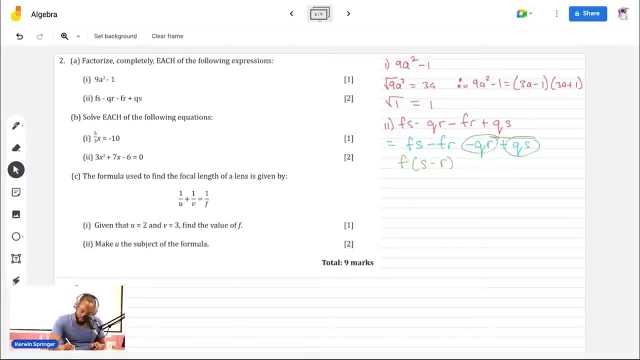 q is common here, but it was s minus r. So what you are going to do here? Tell me if you've already seen it, Because I want to put back the same s minus r there. That's how these grouping things work. 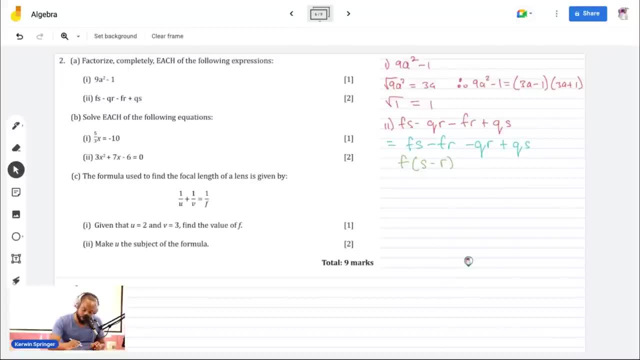 Some of the brilliant people have seen it already. What I will do is just rearrange these two, So think of it like I'm just rearranging it up there so you could follow even faster. qs, minus qr. But when you see minus qr. 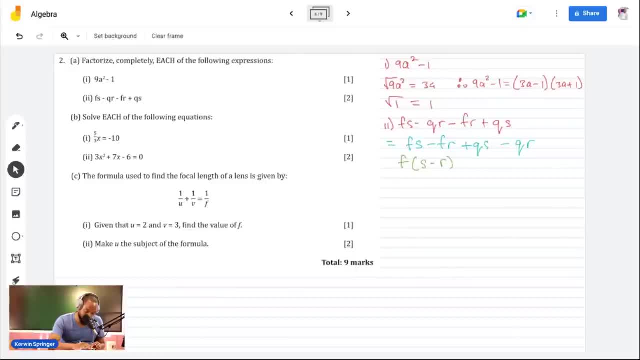 this negative could stay with the r, So I could pull out the q. See that, Pull out the q And I have a next s minus r there, And since both of them have s minus r in the brackets, I have f times this. 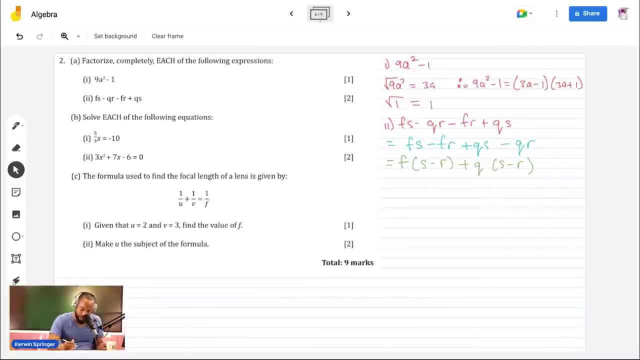 and q times this, I could say it's really f plus q times that. So f plus q will go in brackets and then one of the s minus r goes there, And that's how you do this. Make sure you understand that, folks. 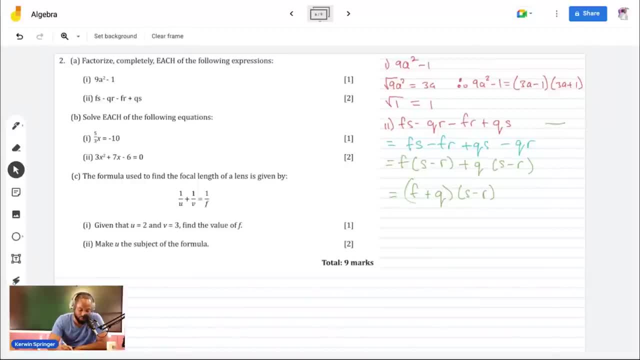 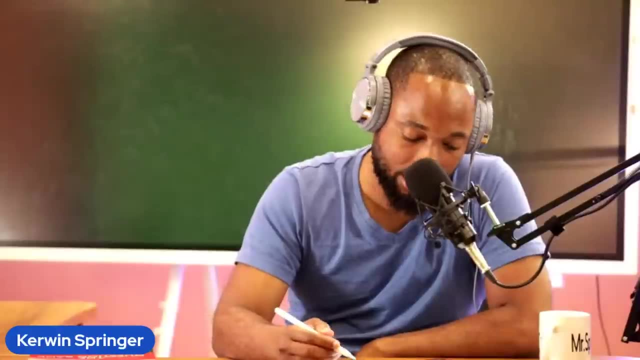 This is a nice little twist they put on it. It wasn't that straightforward. You're still in the mid to lower levels of what could come in the CSEC maths exam, but make sure you understand and you collect these easy maths. Part b: 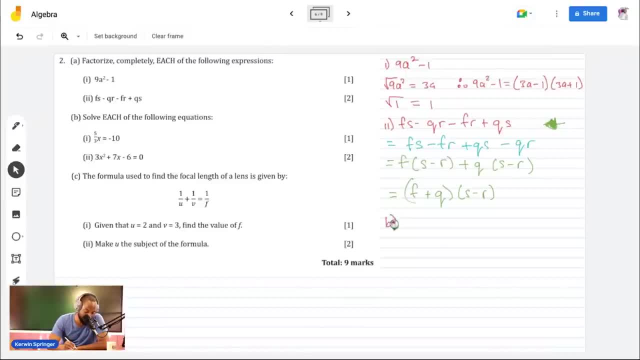 What we're trying to do is put the whole answer on one sheet of paper. It might work. Solve each of the following equations: 5 over 3 by x is equal to negative 10.. Here see nothing. Nice food, And this is. 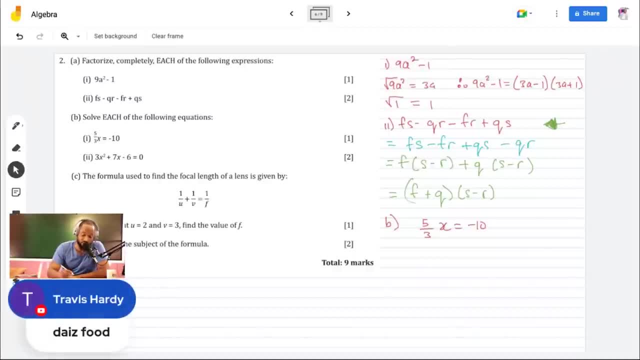 fantastically easy to solve. We're just going to bring across the tree. So 5 by x is equal to negative, 10 by 3 is negative 30. Then bring across the 5. Negative 30 over 5.. You understand? 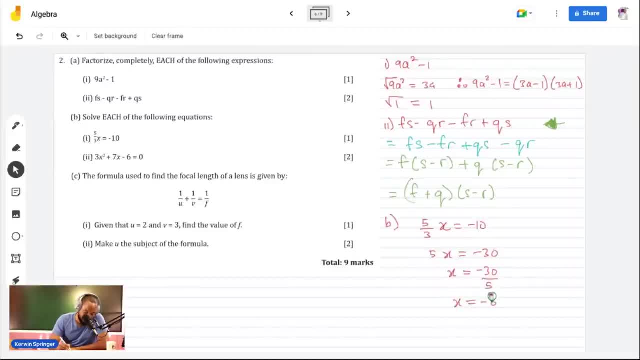 Swap the operations. So x is just straight up, negative 6.. And I forgot about writing to make this fit in one page. Hey, I need to insert a page here. Hold on, Because the next page is the next question And these questions are pre-lined up. 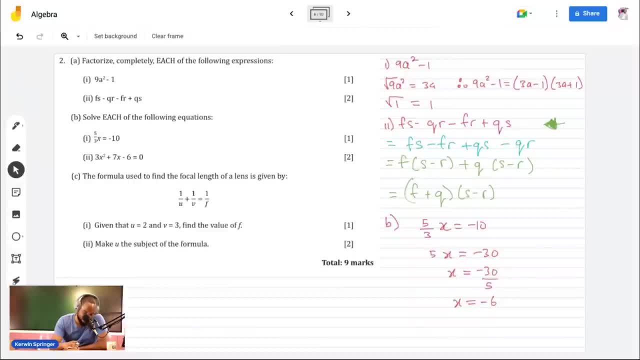 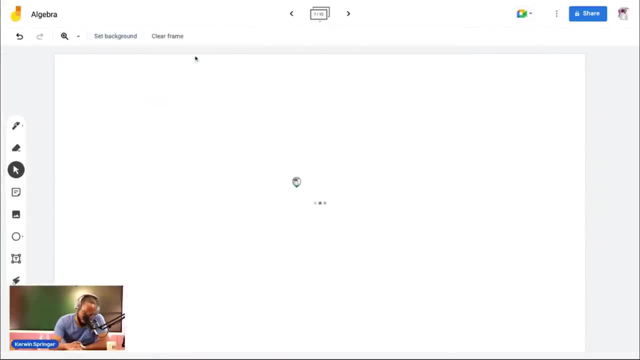 I do. Alright, I inserted a page here, The new 7, now everybody. And now what I want to do? I want to bring back up this last piece. Anybody know what this formula is? Anybody doing physics and all? 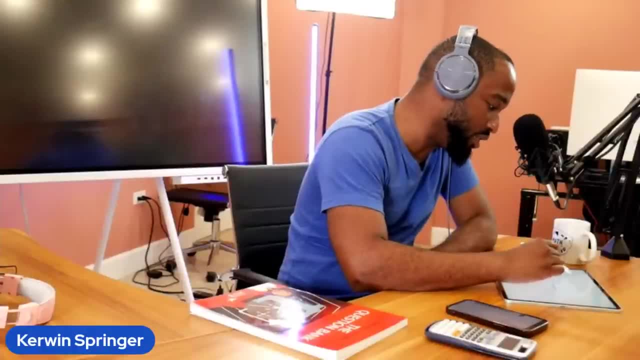 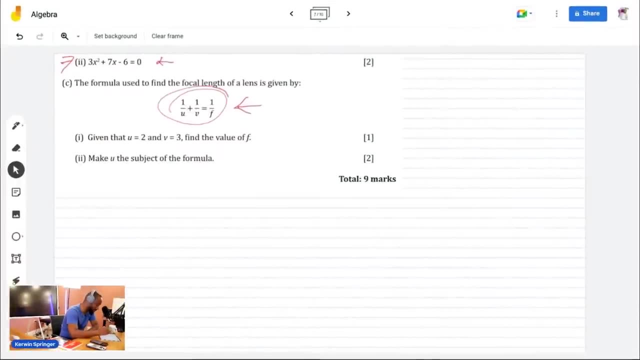 you know what this formula is called. I know you still have to do this one. I'm not going to skip a question again, Hopefully, But you know what this formula is called. All the revising, all the physics, They kind of give you a hint here. 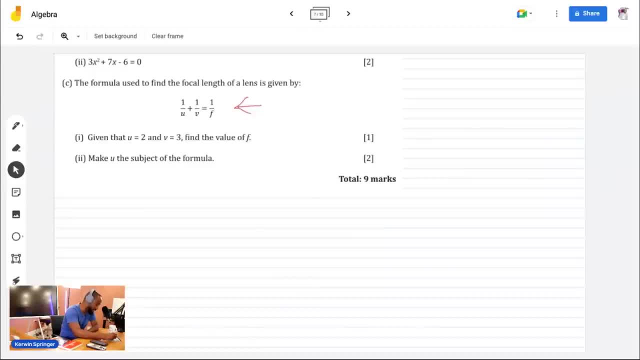 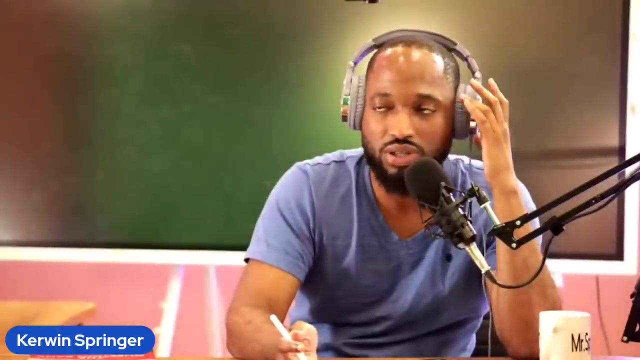 So we need to solve a quadratic. How much quadratic are we going to solve? Imagine going into your maths exam and not knowing how to solve a quadratic. I feel you One of the things I used to tell parents all the time. I used to talk to a parent who interviewed you. 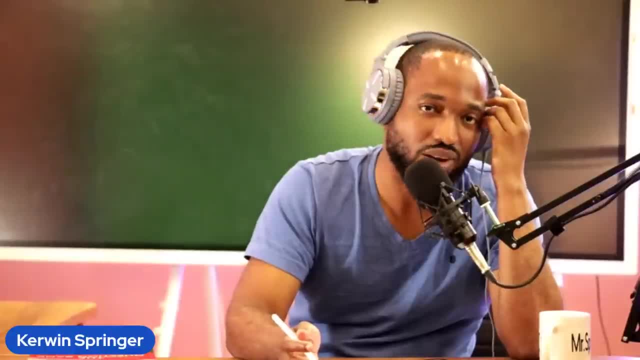 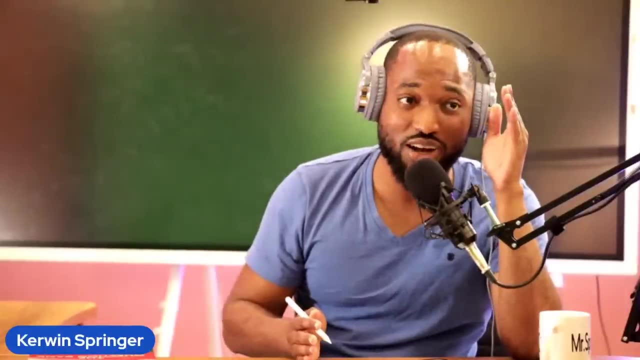 What I will do is ask them to solve a quadratic. If they can solve the quadratic and know, they're at a certain level in maths. if they can't solve it and know well, they ain't even reaching half mark in mathematics yet. So 3 by 6: 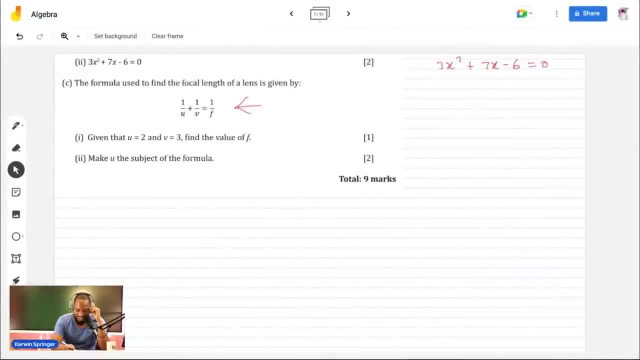 3 by 6 is 18 and I want two numbers that would add up to make 7.. So I've already seen that 9 and 2 kind of play go in a playoff there. I'll make the 9 positive. 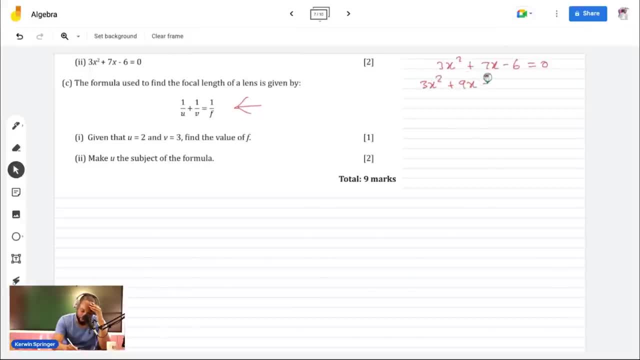 3x squared plus 9x minus 2x minus 6 is equal to 0.. And I'll say 3x into 2x plus 3.. Put back the x plus 3 one time and I see that little negative 2 could go there. 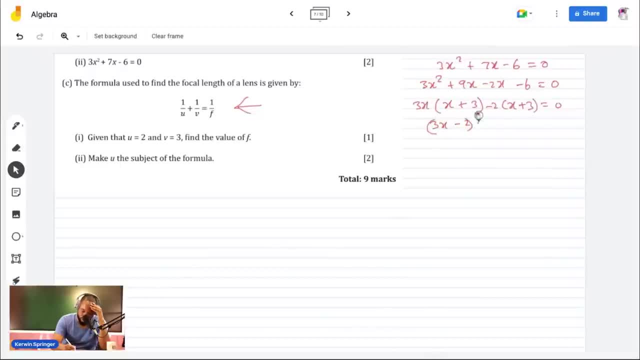 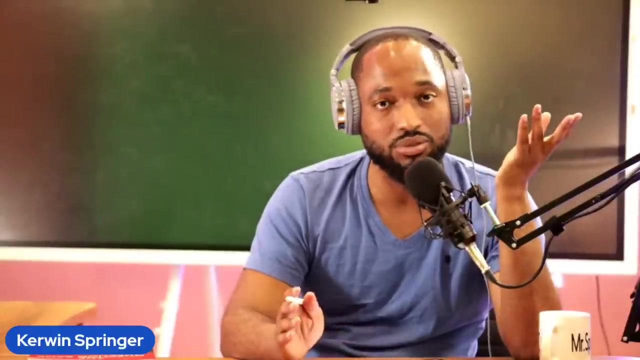 Really nice: 3x minus 2x plus 3.. Will we be supposed to solve this? Yes, we will Either if two multipliers, two factors, giving you 0, one of them has to be 0.. This is, coincidentally, 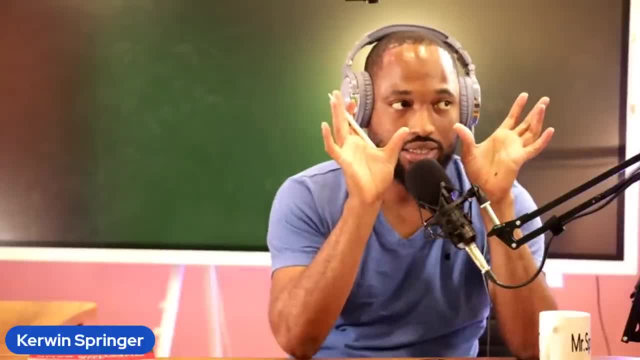 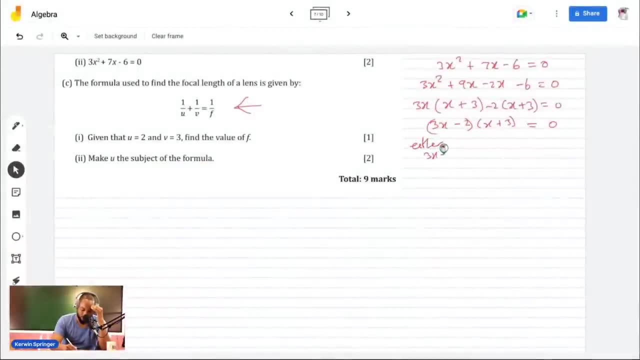 called the root. So anytime you have two numbers that multiply to give you 0, one of them has to be equal to 0. So either the 3x minus 2 is equal to 0 or the x plus 3 is equal to 0. 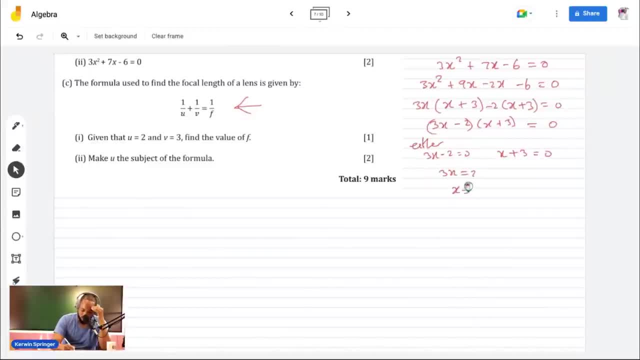 So 3x is equal to 2, x is equal to 2 over 3.. I just solved that for x, Or x is equal to negative 3.. And that's my two answers there All again, long time. And here this is the Lenz formula. 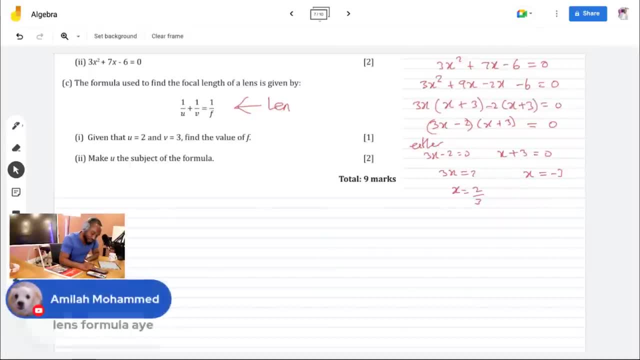 Well done Amila And everybody else who say Lenz formula, I'm representing. It's the Lenz formula. So what they want us to do, given u is 2, given v is 3, find f. So let me rewrite it as 1 over. 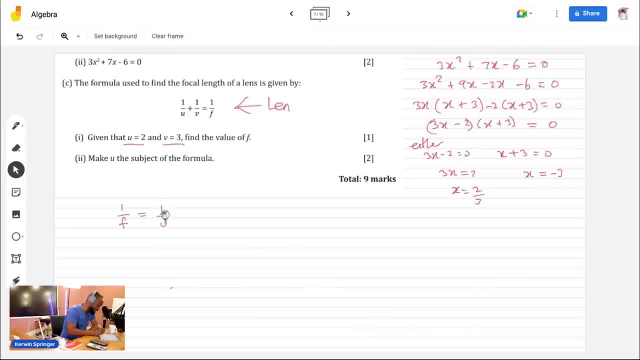 f is equal to 1 over u, that is the object distance, plus 1 over v, the image distance. I hope all the physics class, or physics later, will tell you: Don't feel we still have class, We still have class. 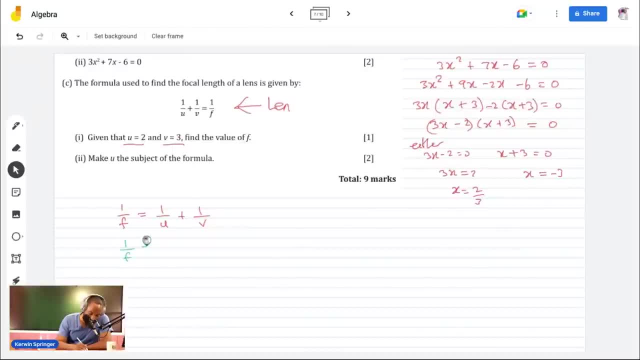 So, whatever f is equal to 1 over u- in this case 2.. So when u equal 2 and v equal 3, we're going to get this situation taking place here, Plus 1 over 3. A half. 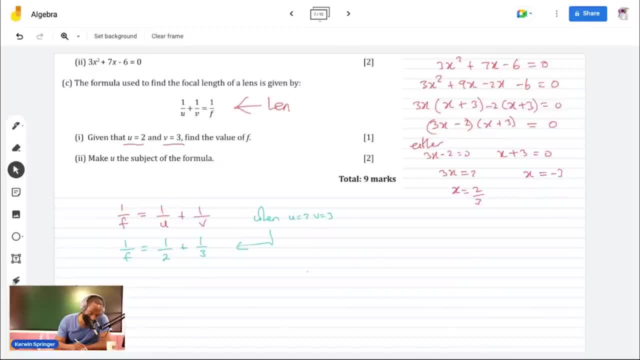 plus a third is how much? So what I can do is say the LCM. I can say the LCM of 2 and 3 is 6. 2 by 3. 6. 2 into 6, 3.. 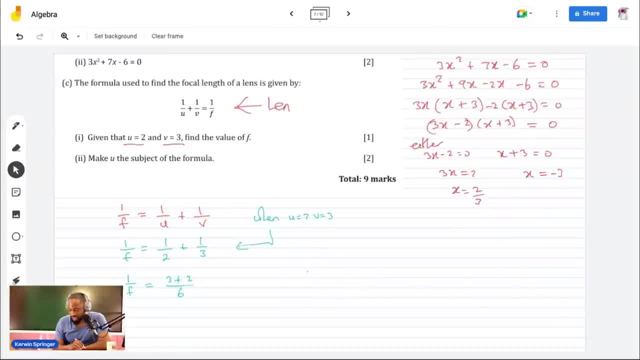 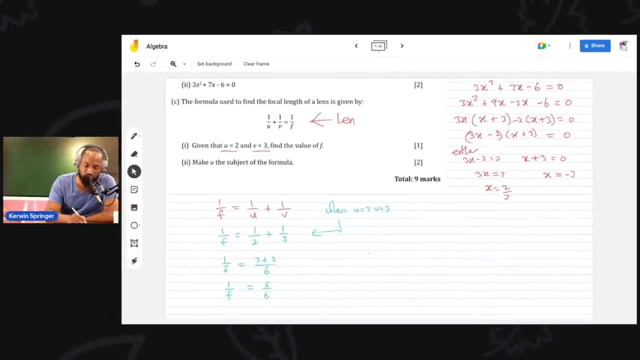 3 into 6, 2. A half plus a third is 5. 6.. Yes, So 1 over f is equal to 5 over 6.. But the answer doesn't want you to find what is 1 over f. 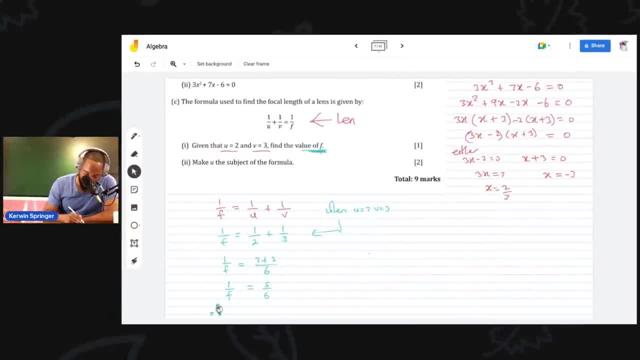 It wants us to find what is f, Therefore f. Why did I write 5?? Anybody write 5 when you're trying to write f. 5 at f is equal to 6 over 5.. f is equal to 6 over 5.. So, if I flip, 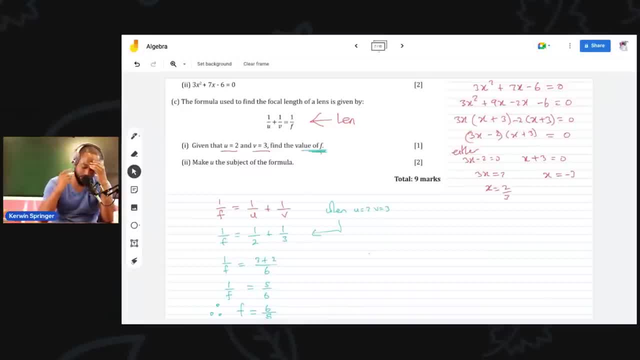 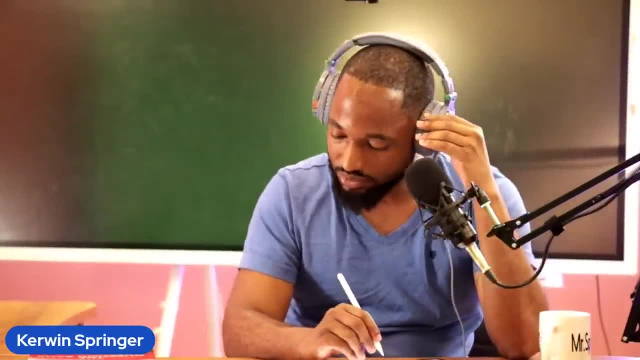 the 1 over f, I'll have to flip the 5 over 6. And there we are. There we are. Last one is to make u the subject of the formula. Make u the subject of the formula, So we have 1 over f. 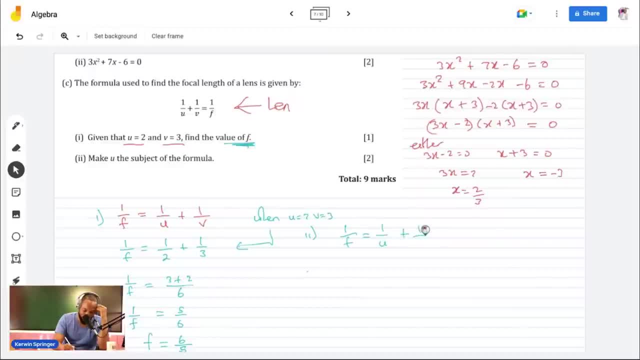 is equal to 1 over u plus 1 over v. Where is u There? it is, Wait. no, There it is. So we're going to make u the subject of the formula. Hmm, So let's get everything that's not u on. 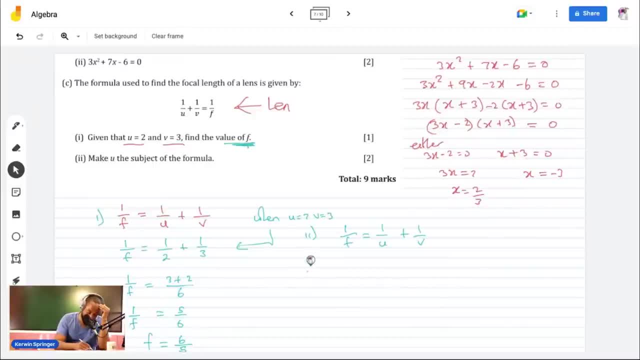 one side. So 1 over f will be here. Take away: 1 over v is equal to 1 over u. All of you follow that. I'll just take that whole 1 over v term and say, go so, And let's switch the operation. 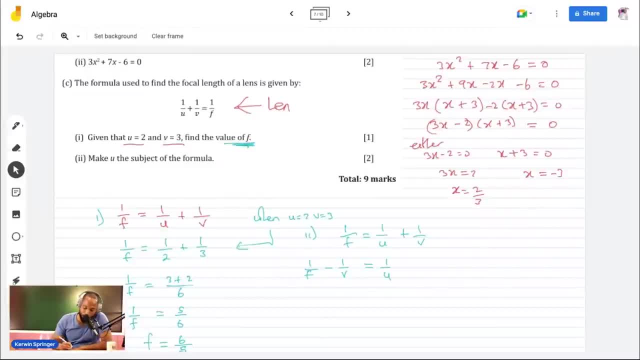 So instead of being plus 1 over v, it turns negative 1 over v. I know I need to reciprocate this, but I can reciprocate something if both sides have a solid fraction. It's hard for me to reciprocate this. 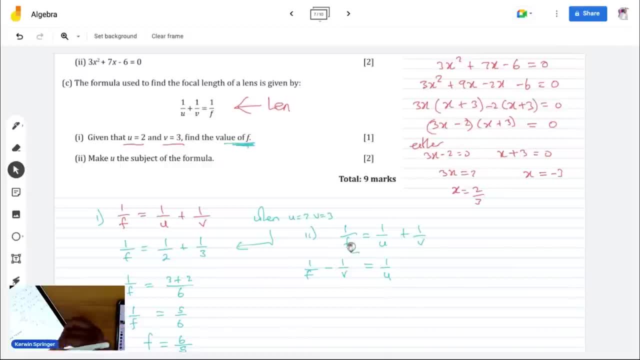 if this is not one term, So I actually need to make this one term. first, Those of you all who flip this and just flip these two things separately. that's wrong, Wrong, Don't do that. You have to make this into one term. 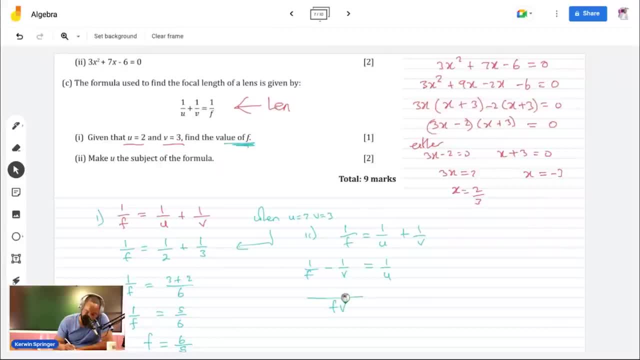 So this is going to be f v, f into f, v is v, v into f, v is f. Don't forget the negative sign. And now I reach here. Now is when I could reciprocate it and be like: well, if I flip this, I need to flip that. 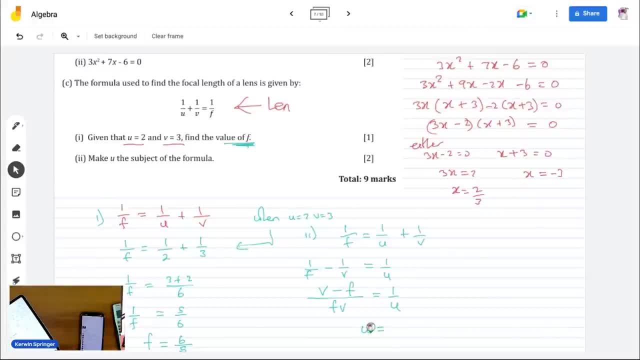 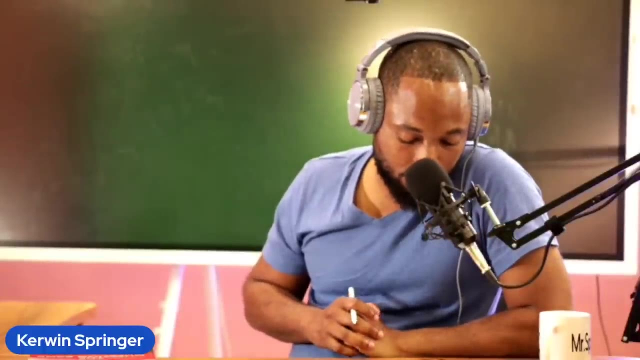 and that's the answer there. So I'll get: u is equal to f, v over v minus f. ladies and gentlemen, What do you think You all understand? Mash up, Mash up. We have space for one more, One more second. 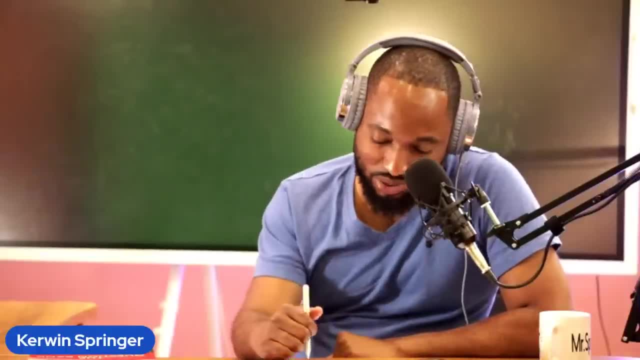 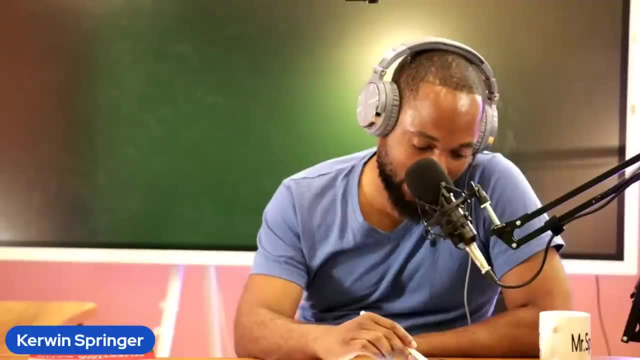 Huh, Ah, yeah. we are in time, man. We have space for one more. We have space for one more, Two more, One, one, one, one more. Wait now, This is the fifth question already. That is performance. 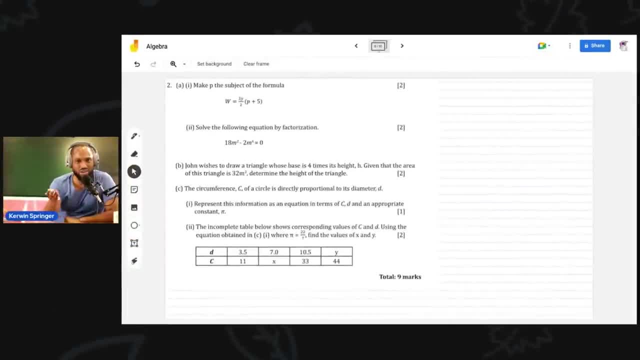 One more. So already for the algebra question, is things just like this going to come? This is based off of like the last five SATA exams. So if you could do, if you find this was tremendously easy, you're in a good place. Go and do the last five. 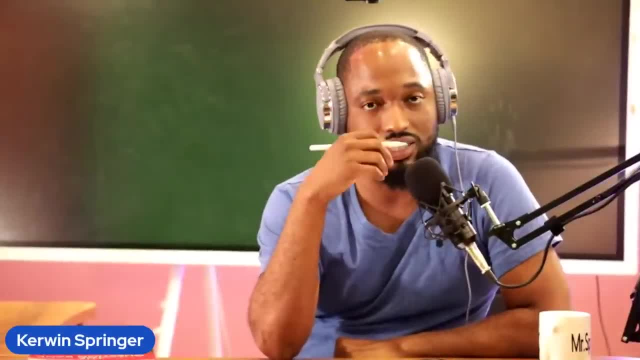 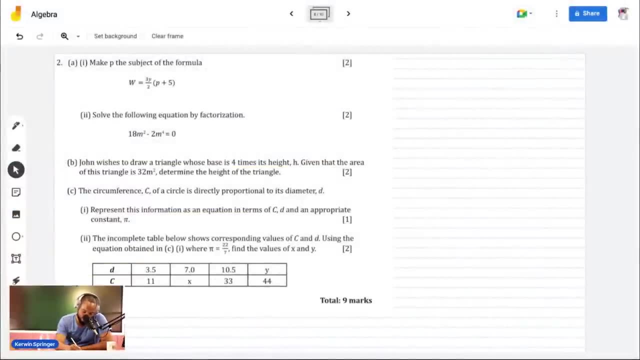 years of algebra. It's coming in question two, and you're starting to look good. You're starting to look good, ladies and gentlemen, So let's just do this. last one W is equal to three y over two. I don't even know what the question is saying. I just started writing. 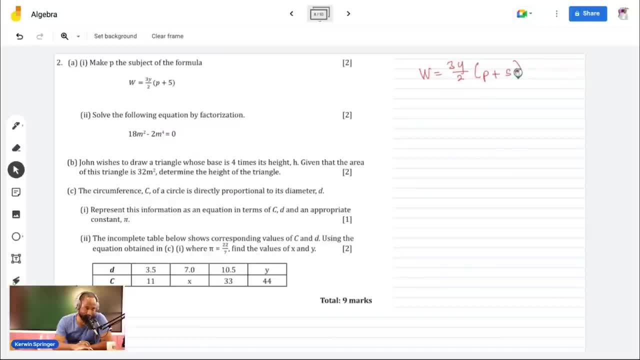 one time I'm like a teacher. W is equal to make p the subject of the formula. So we need to make p the subject of the formula. P by itself, Alright. So anything that is not p, you get it out. 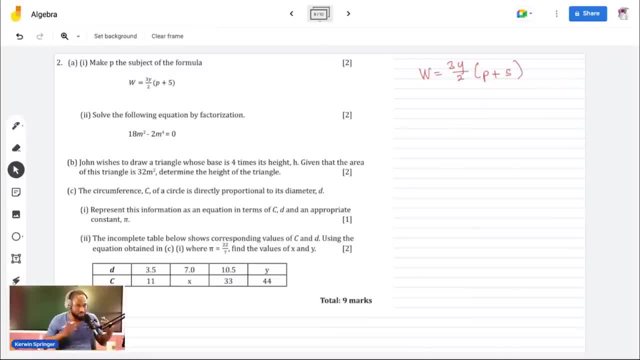 Now we can't go and bring across the five one time and the five trapped in the brackets You have to is like when you start a job, the last person to get hired is the first person to get fired. if anybody had to get fired, So the last. 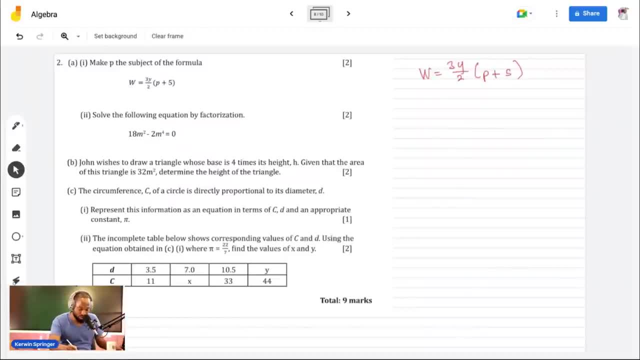 operation. you think this away in terms of operation from the p you need to come across first, That's this term: Three y over two, Or like you could do it separately, You could take the two and then you could take the three y. Let me do it separately so. 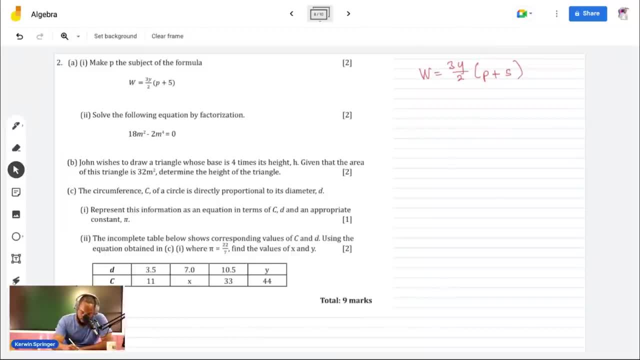 everybody could follow along. So I'll bring across the two and I'll end up with two by w is equal to three y p plus five into p plus five. You all understand that, Because the two was dividing. Bring it across and multiply Then. 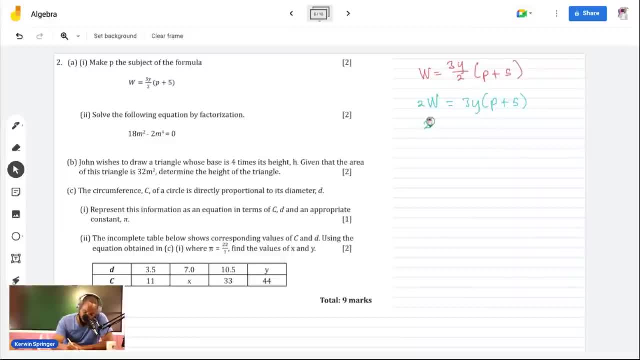 the three y is multiplying. So when I bring it across, are you agreeing with me that I should have something looking like: three y here is equal to, and I have the p plus five there. And now it's just to finish strong enough. 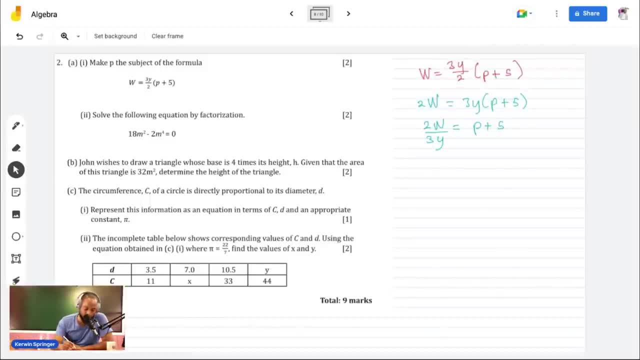 Joshua and them done mashed it up already. So to finish off strong, the p would be p. I'll just bring across the five and it'll be negative. I'll swap in these sides one time. I hope you all okay with that. 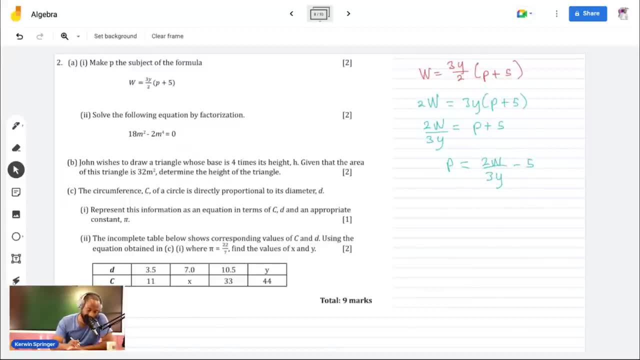 And that is we ready, Ramco. Oh yes, Solve the following equation by factorizing: Another factorization, because they must bring a factorization in question, two, Otherwise it's not sexy. A factorization doesn't come like one. 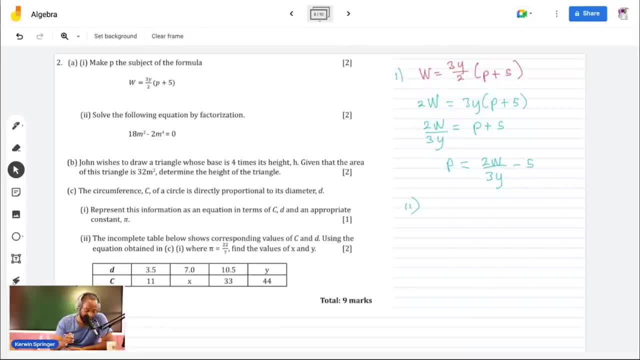 in every ten times. It must have a little factorization. So who is this boy? This one looking highly suspicious, Detecting a piece of foreplay? So, um, hmm, looking like a type of difference of two squares liming in this. 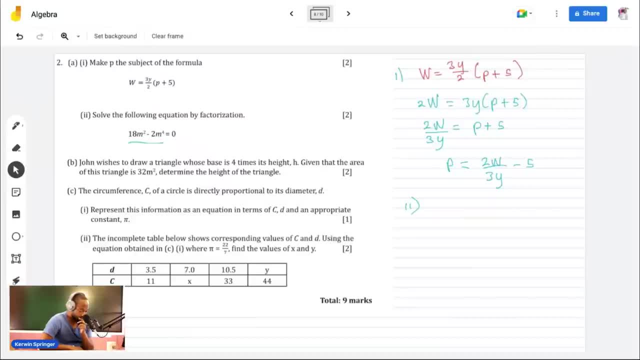 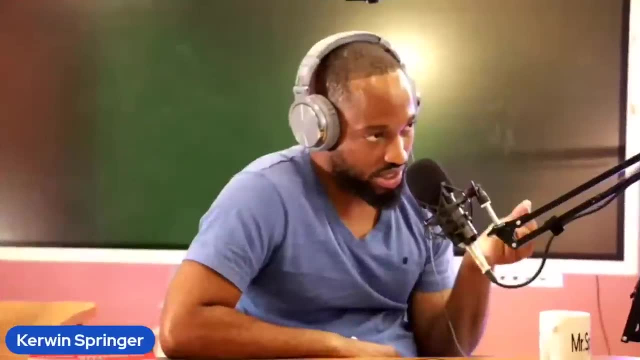 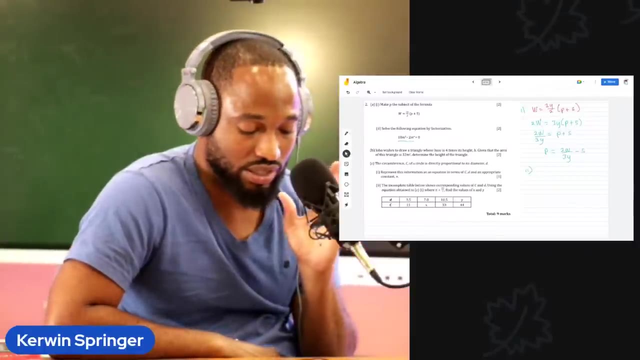 Because the way to factorize and solve. So I could do it. I could take all the two and I'll see the difference of two squares. But I want to pretend like I wasn't seeing the difference of two squares. Let me see. 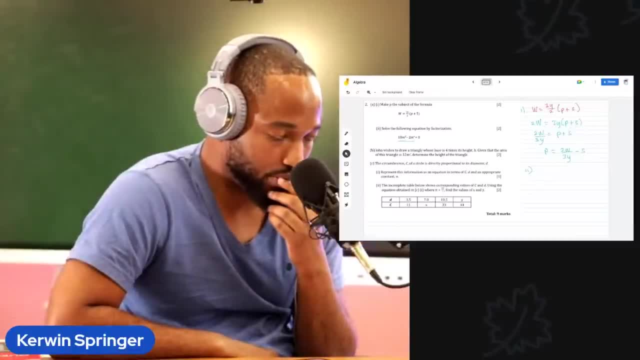 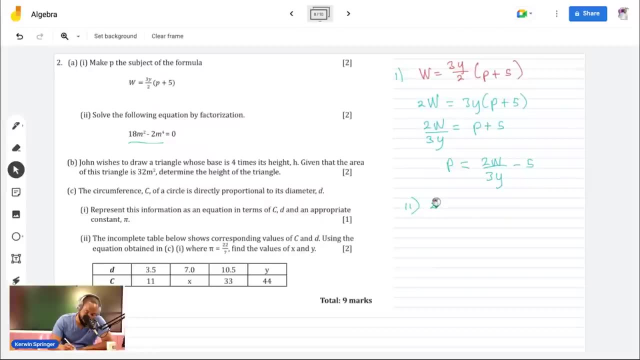 if I take out, factorize it fully, what would happen If I took out the two and m squared, I will end up with nine minus m squared. Agreed, I'm watching this term here. Let me write it. Let me write it on top. 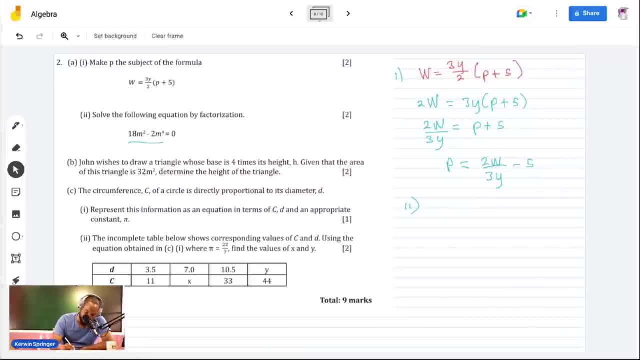 We are on the last question. I could roll it, I could do this thought exercise with me, So this two m squared could come out. That's the most things that could come out, The most amount of common things. So I'll end up with just nine here, minus. 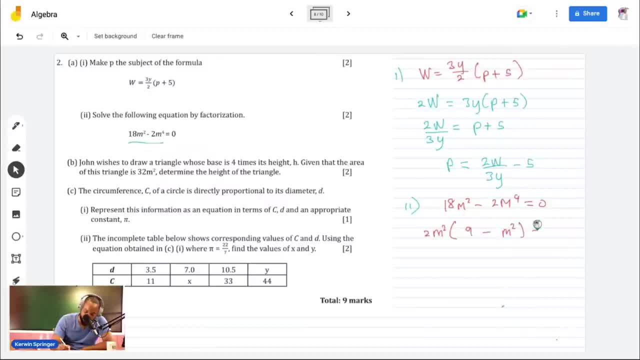 and just m squared there. So at the end of the day, this is going to give me two m squared into three minus m, into three plus m. Those of you all who understand that, fantastic. Those who don't. this is difference of two. 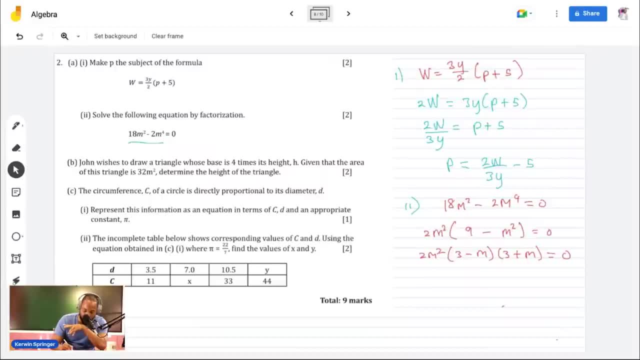 squares here. you know, Nine is a square number. The square root of nine is three. m squared is a square number. The square root of that is m. And then our product. It has three factors. So it's either: 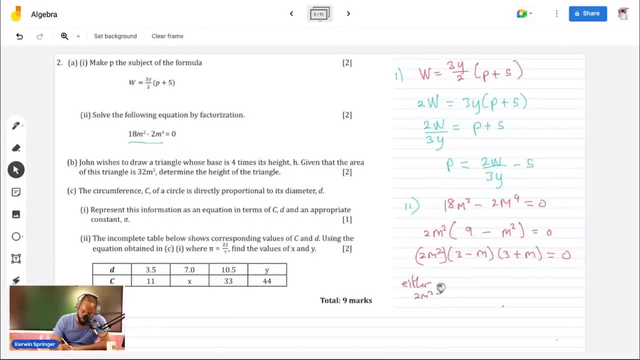 two m squared is equal to zero, which would just mean m is equal to zero. Bring across the two: divide by zero Zero, divide by two is zero And square root of zero is zero. So or three minus m is equal to zero. 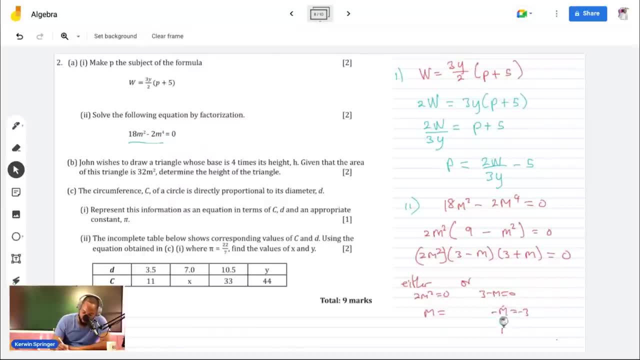 So negative m is equal to negative three, So m is equal to three. Or three plus m is equal to zero, So just m is equal to negative three. So m could either be equal to zero three or negative three if I do it that way. 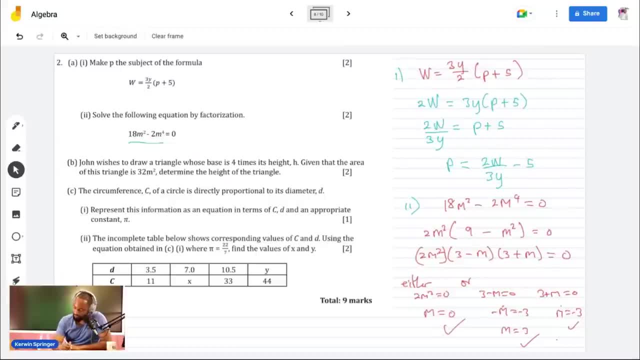 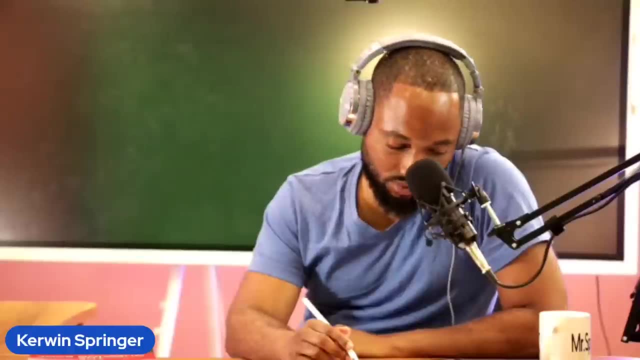 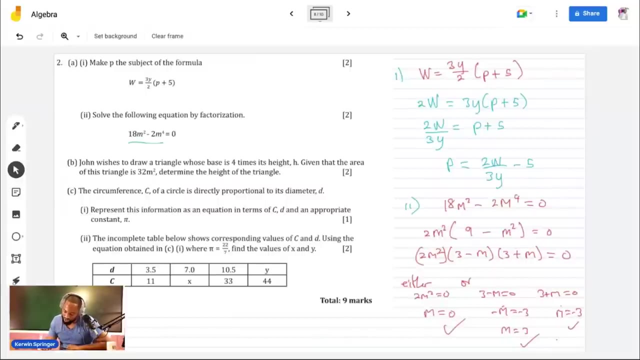 Let's try the other way that we can do this. Eight m squared minus three. Mash it up, Is that one? I mean? now, where is it coming out? I hope I didn't make any mistake anywhere. Nice, Or what is this? Eighteen m squared minus two. 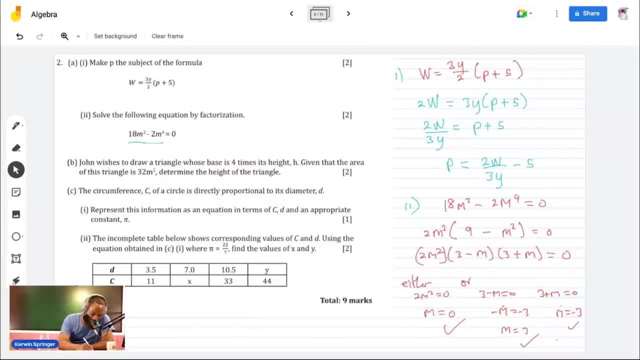 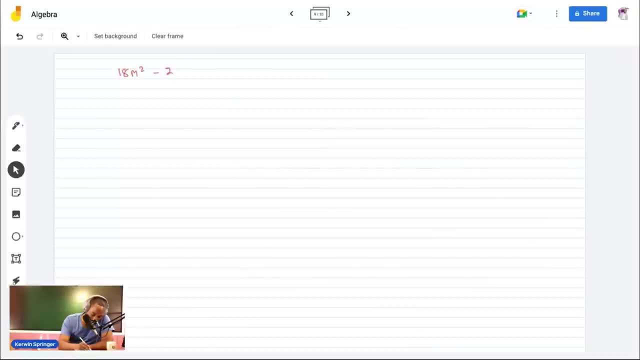 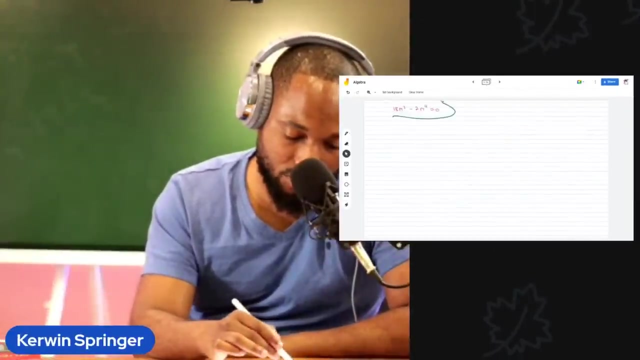 So we're going to the next page. Eighteen m squared minus two. I'm going to just wait for the lines. Two m to the power of four equals zero. Okay, okay, I can just be a little more. a little more. what is the word I'm? 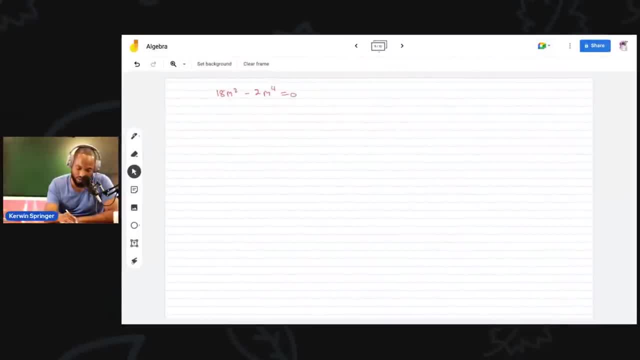 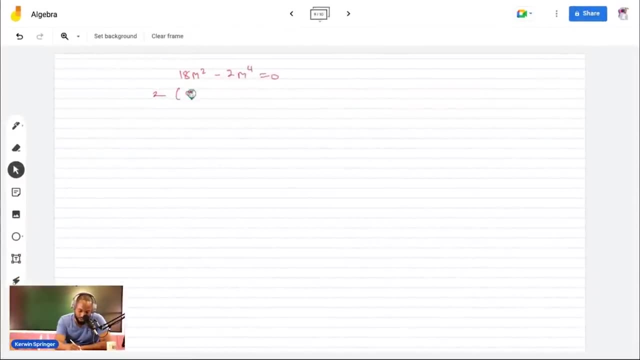 looking for Conservative with the things that I'm taking out. So I can kind of partially factorize this. Maybe I can just take out two, Maybe I can just take out two and humble myself. So if I want to just take out two, I'll end up with 9m squared minus m to the 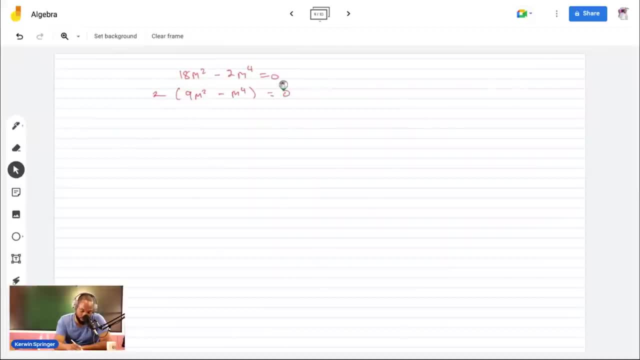 power of 4.. And then I do the difference of two squares, So I'll end up with 2 into, and the difference of two squares here will give me 3m minus m squared and then 3m Plus m squared, Which means I can still factorize out a m. So yeah, all of them have a m inside. 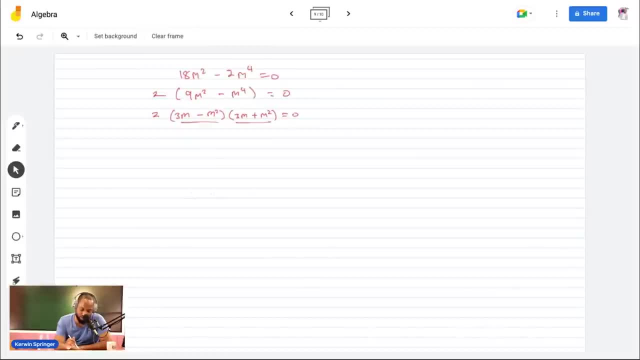 them. So it's best if I actually take out an m, I have to take out a m, Otherwise when I'm solving this I will end up with the next. this will just be too problematic. I'll end up with. I can solve this. you know, I'll end up with a lot of factors. I'll end up. 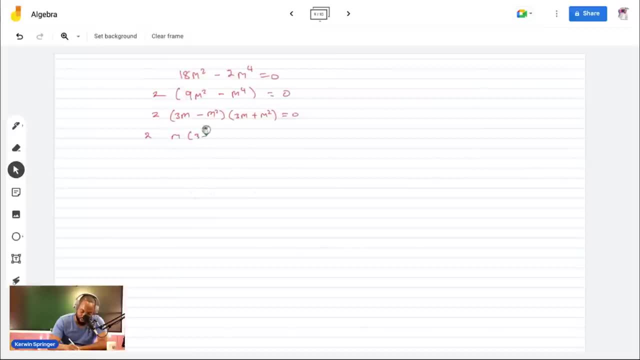 with 2 into m by 3 minus m, And then another m. here I'll end up with m by 3 plus m And I'll end up back in the same place that I end up with. b4 equals zero, Which is hope you're all following, and again confused, which is: 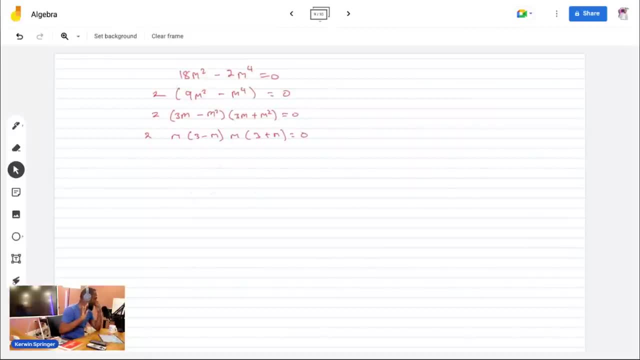 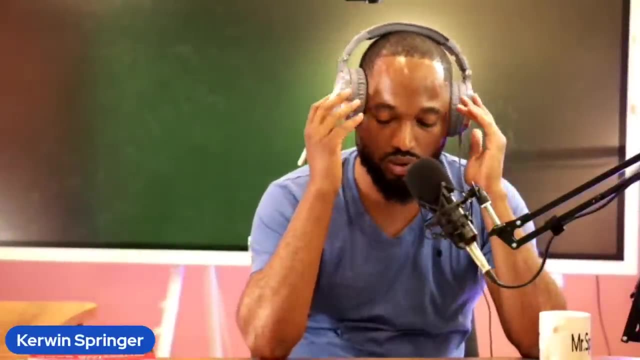 the same thing here, So this one was a little challenging If you're not accustomed to polynomials that go above the power of 2, but this is the idea behind it. Sometimes you do what you want to take away from it is. sometimes you do it. Sometimes you do it, You do it. 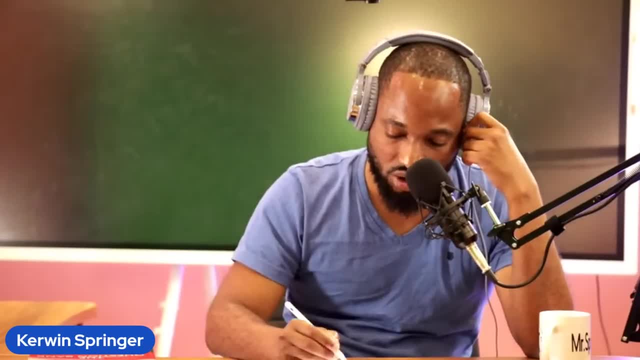 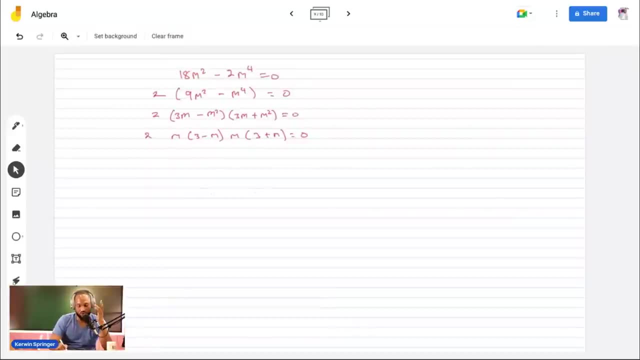 to do a basic factorization, because i just took out the common term here, which was 2m squared, and i end up with another thing like maybe i'll end up with a quadratic inside or difference of two squares, so i do that separately. i can show my working for this on the side too, if i want. 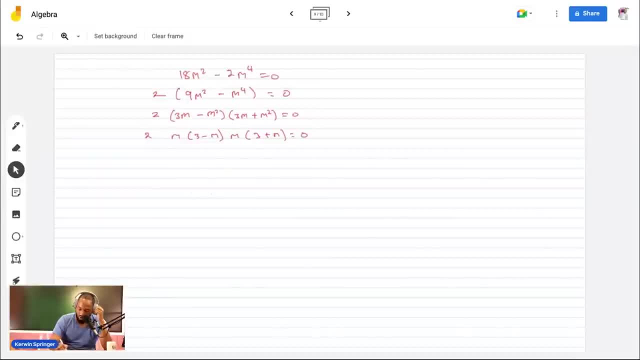 and do that separately, and then all three of the factors equal to zero, these three terms equal to zero. so either this one is zero, this one is zero, or this one is zero, and you solve all of them and you'll get some working for this. so let's finish off strong with the last part of this. um, oh no. 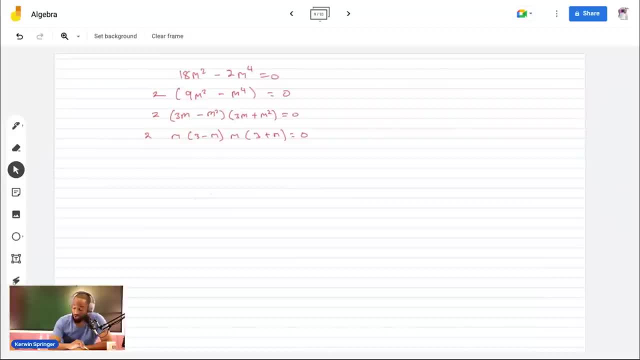 there is a question after this. are you ready to do a question of 375 people here? how much likes it up on this video? are you pressing like and thing? take a screenshot. wait on instagram. tag me. let me have something to repost when the live finish. now, so let me do the last part of the 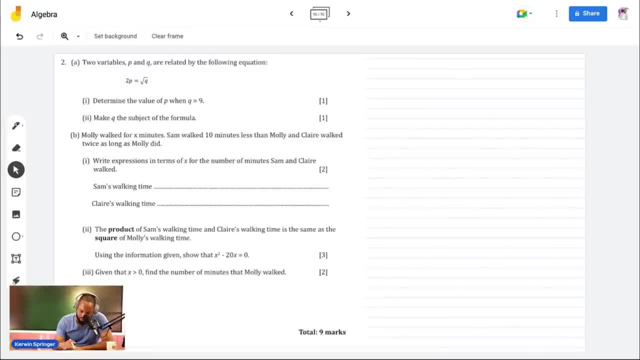 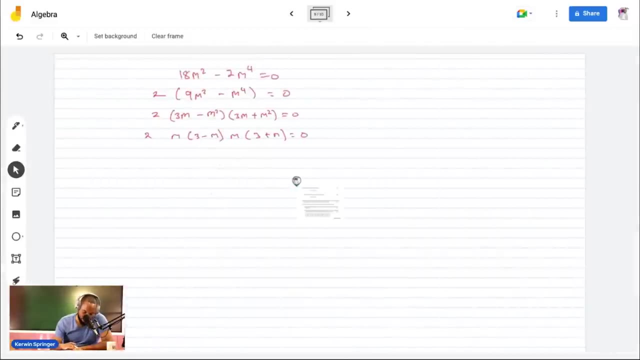 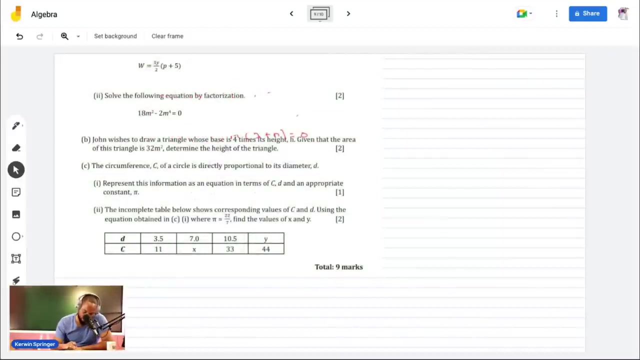 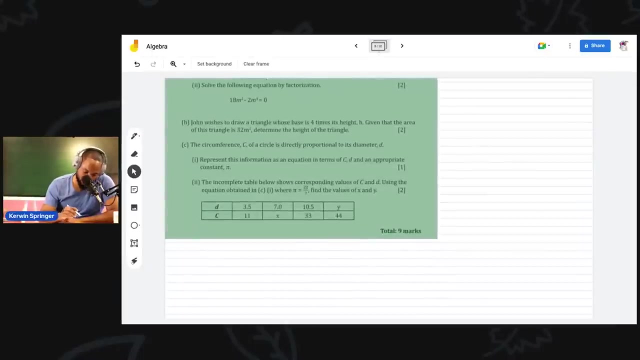 question. you could add sticky notes and thing. um, um, I want to do it on page nine and the last part of this question and some triangle talk and all kind of thing. some triangle talk: um, John wishes to draw a triangle. are we reading that? you seen it? 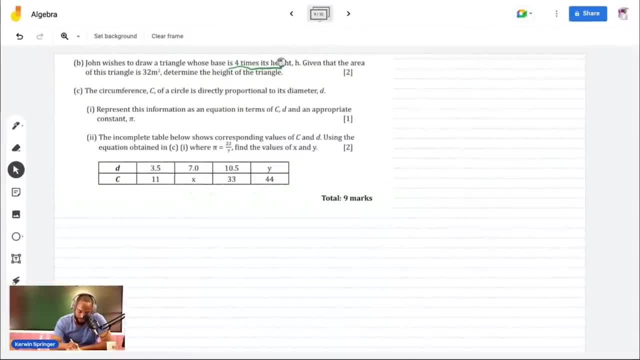 you should to draw a triangle whose base is four times its height. So the base of the triangle is four times the height of the triangle. Given that the area of the triangle is two meters squared, determine the height of the triangle. Let me visualize this. So this is the triangle. 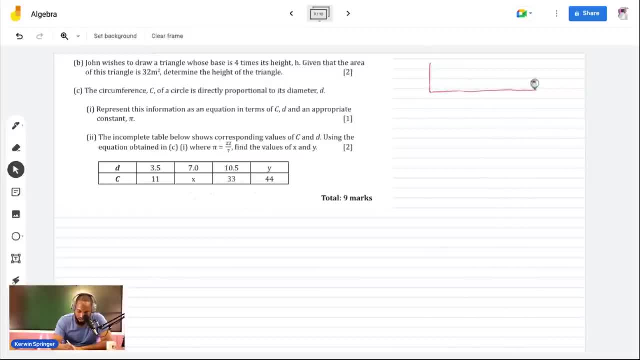 here, boy, That kind of long triangle. The base is four times the height. So let me say this is the height. I could write base here, but it's better for me to write four heights here. You understand what I'm doing there. You understand that. So the triangle is h. 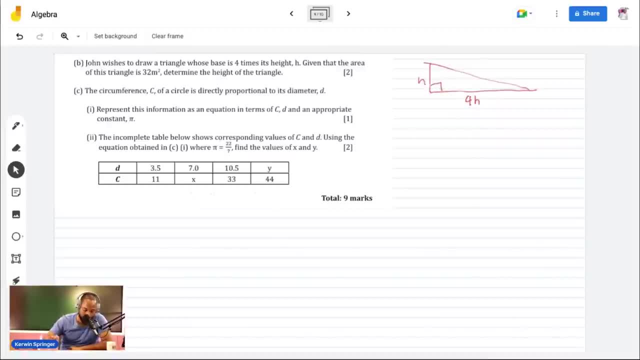 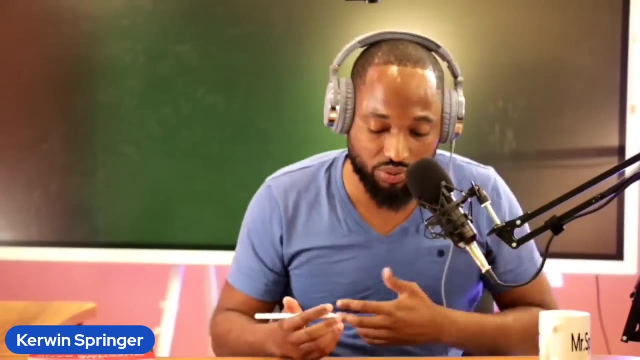 high and four h base, And the area is 32.. So this is where they tie algebra into geometry, into measurement. So they give you something and you need to generate an equation out of that. What was the area of a triangle? Area of a triangle is base, the simple one base. 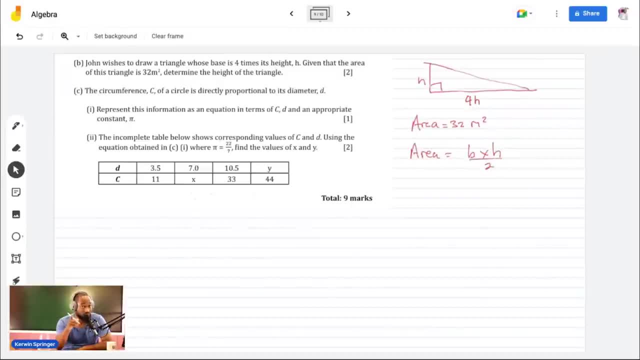 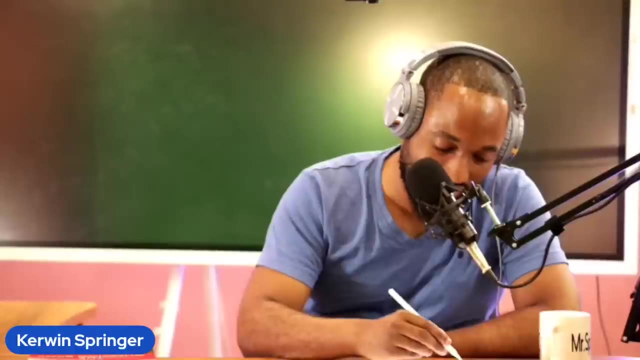 by height divided by two, But the base is four times the height. So the area of this triangle, in this case, in this case- let me write in this case here, You know, make it look official- In this case, Your Honor, the area is actually four times the height by the height by the two, because 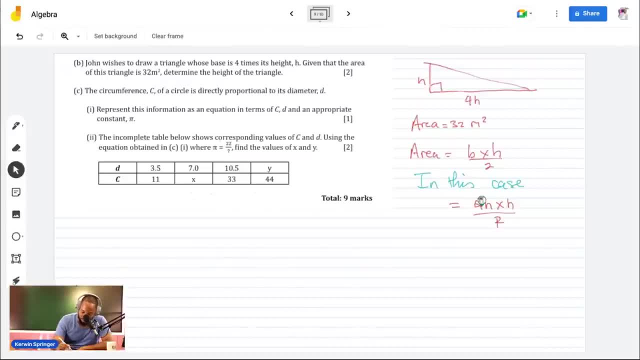 the base is really four times the height, And I do a cancel here one time- So it's really two h squared, Nice and neat and compactly. So the area is really two h squared, Which means therefore, since the area is really 32,, two h squared is 32.. And h squared is 32 divided by two. 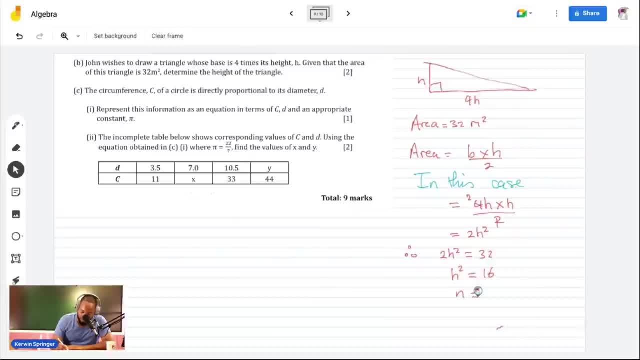 which is 16.. And the square root of 16 is four. It can't be negative four. The square root of 16 could be negative four, but we can't use negative four in this case, because you ever see a triangle that's negative. 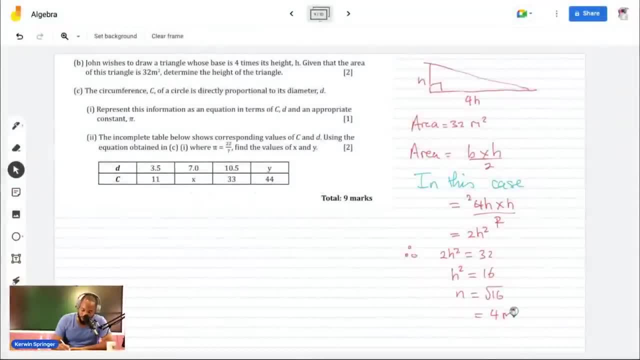 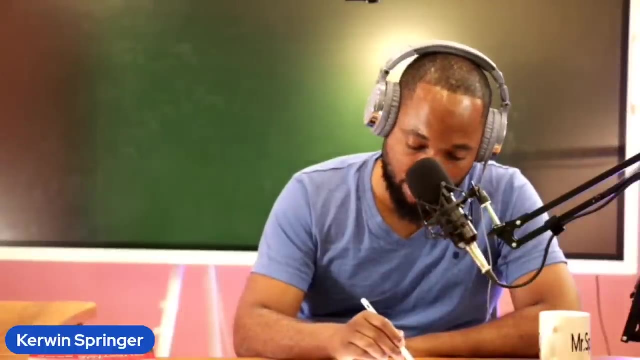 A negative dimension. So h is four. Determine the height of the triangle. It's four meters. And if they say, determine the base four by h, four fours are 16.. Last part, That was a nice question. Circumference C of a circle is directly proportional to. 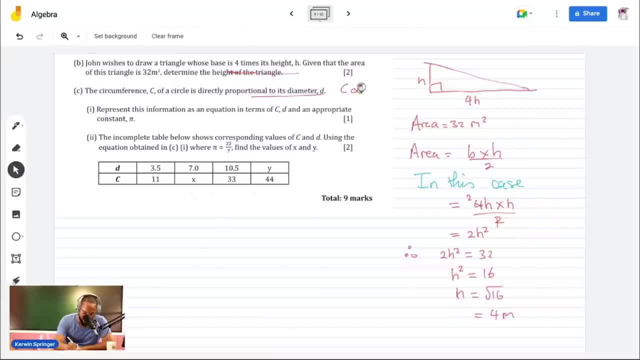 its diameter. So C is directly proportional to the diameter. Represent this information as an equation in terms of C and D and an appropriate constant, pi. Okay, All right now. So this is the circumference of a cycle, is pi? I don't know what I was. 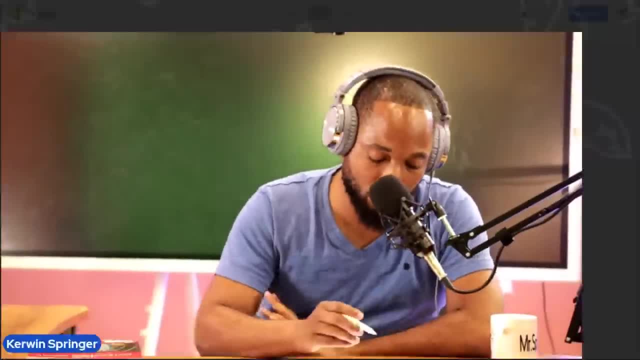 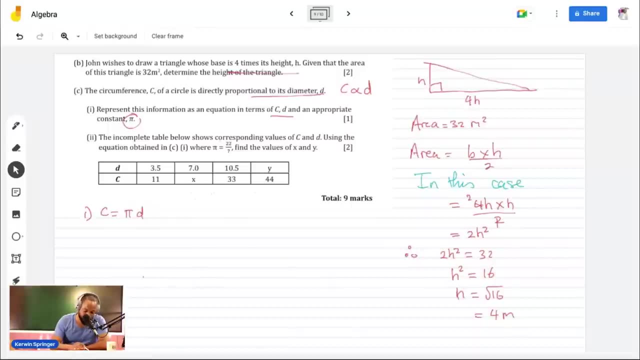 trying to be here, But anyhow. so now we have the pi as a constant, but it's actually an equation you know from since primary school. The incomplete table below shows corresponding values of C and D. Use the equations obtained in there. using that equation where pi is. 22 and 7.. So they want you to use pi as 22 and 7.. Find the values of pi as 22 and 7. Then use the equation where pi is 22 and 7.. So they want you to use pi as 22 and 7.. Find the values. 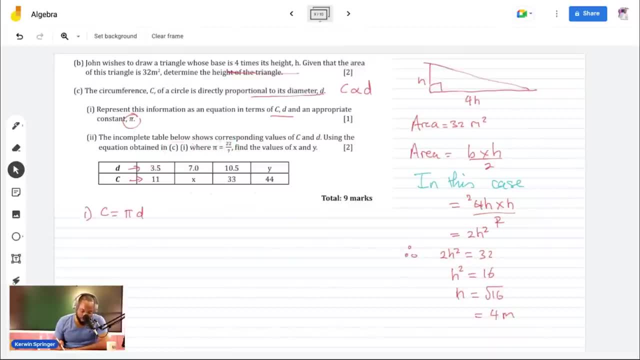 of pi as 22 and 7.. So they want you to use pi as 22 and 7.. Find the values of pi as 22 and x and y. So in other words, the same. take some free marks now. Take some free marks, So in. 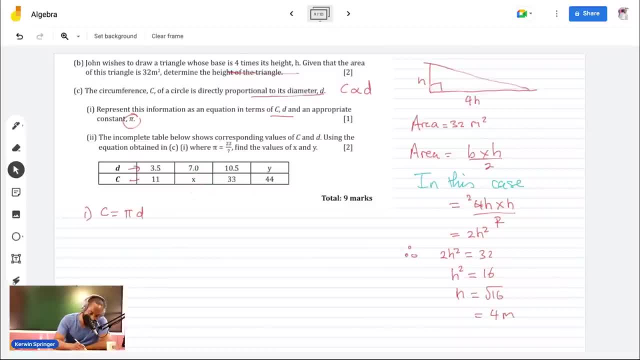 this case. in the first case where we want to figure out x, I would say, therefore, x is equal to pi times d, and d in this case is 7.. And since pi is 22 over 7,, by 7, it's equal to 22 free marks. And in the case of y, 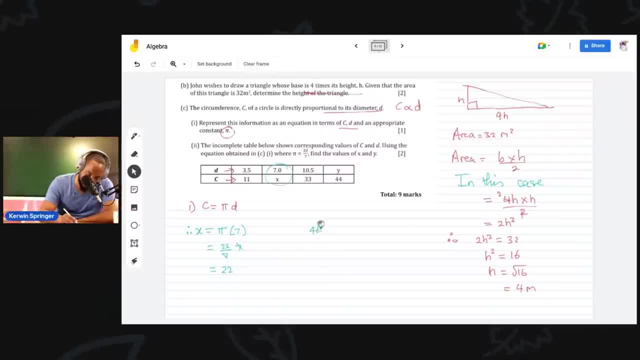 44, because 44 is c. so 44 is equal to pi by y, because y is in the place of d, pi d, pi by d. So you understand it's a substitution question With a little bit of variation. 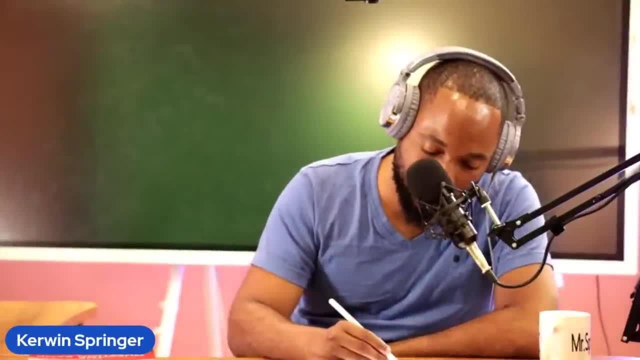 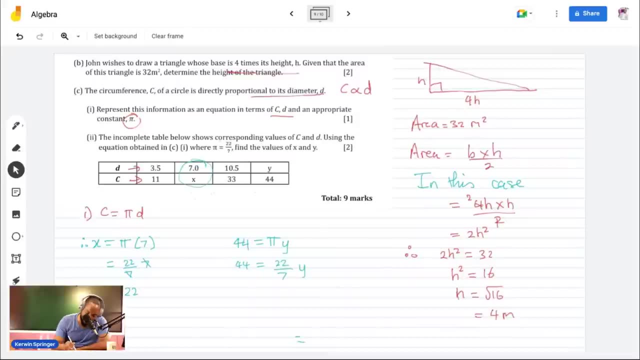 but in reality go deep into the variation technique. But pi is really 22 over 7.. Why? So anybody can multiply 44 by 7 and tell me how much I like it right. Well, the best thing to do is might be to divide. 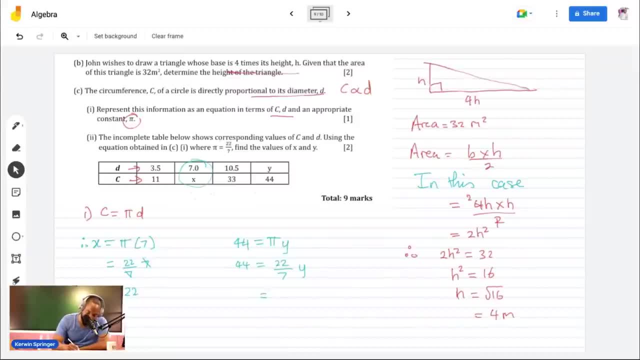 by 22 first. So 44 divided by 22 is 2,, 1,, 7,, y and then 7.. So y is equal to 14.. At the end of the day- you can go and check it out and make sure- The ring across is 7 divided by 22,, 2 by 7.. 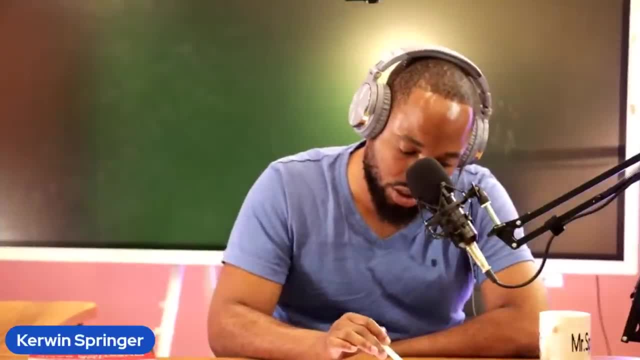 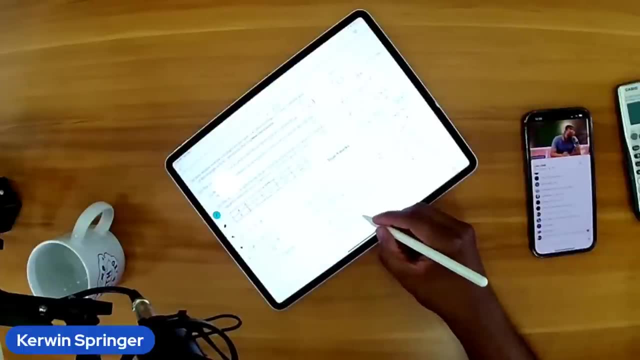 Yeah, but y is 14.. Hey, let me put some dimensions just in case, Just in case there were no dimensions given. So why would you just put units to make the thing look nice? Units, units. Did I put my dimensions here? I did One more question. please, One more for the road. 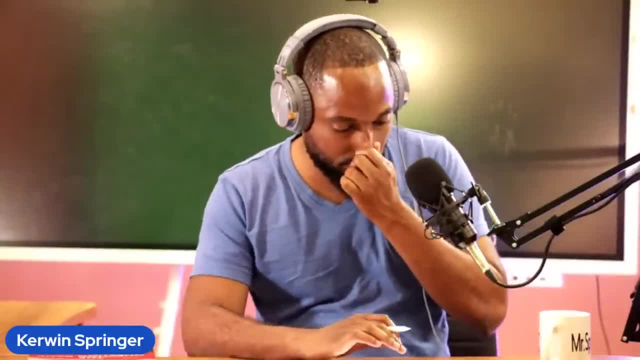 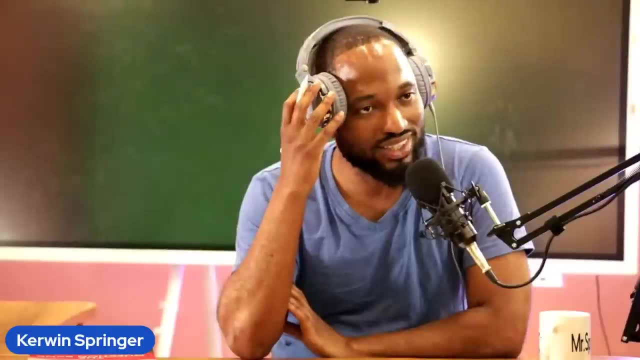 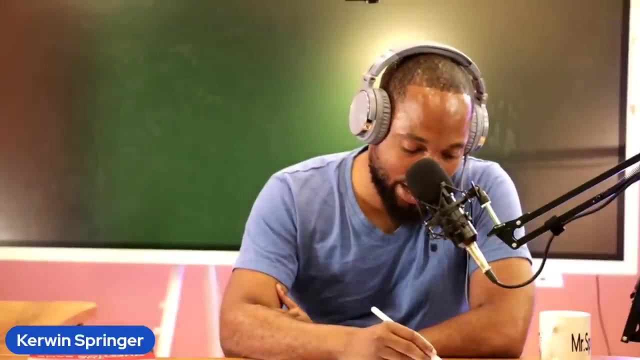 One more for the road. One more for the road. Last one, So two variables. What's that noise? Oli bin, Oli bin, Oli bin. Two variables, P and Q, are related by the following: Hey look, we get a next. 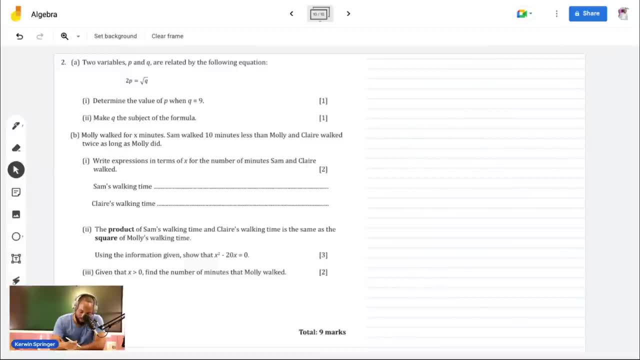 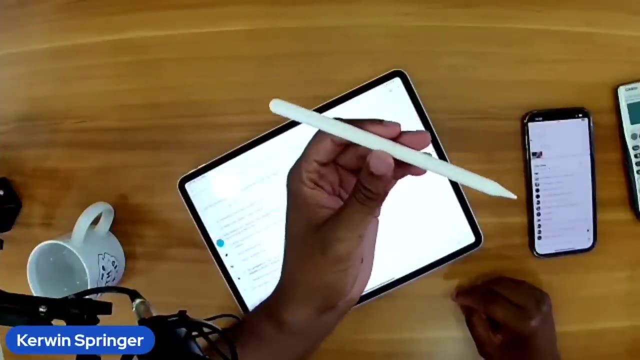 something. Wait, now is my battery dead. All right, Every time I say that my pen is talking about it, I zoom in on the pen. I zoom in on the pen. This pen is holding it down for you. right now, The official Apple pen is not working and I have a generic pen that's kind of doing it for. 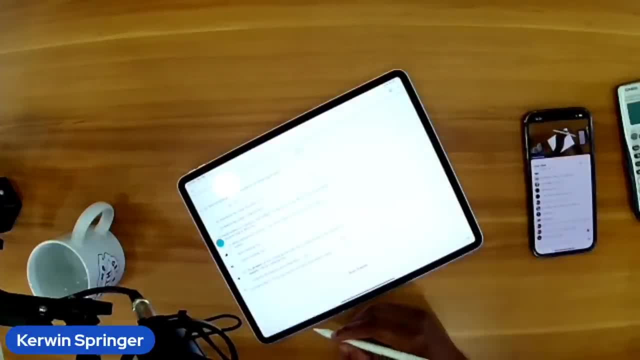 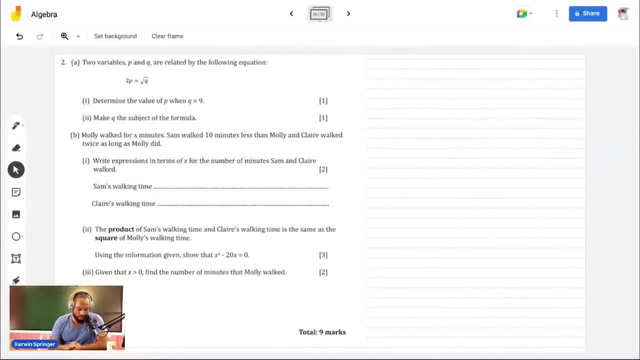 you right now. All right, Let me go to the question. So 2P is equal to the square root of Q. Determine the value of P when Q is equal to 9.. What, Oh, easy thing, Easy thing, right there. Easy thing Also easy It. 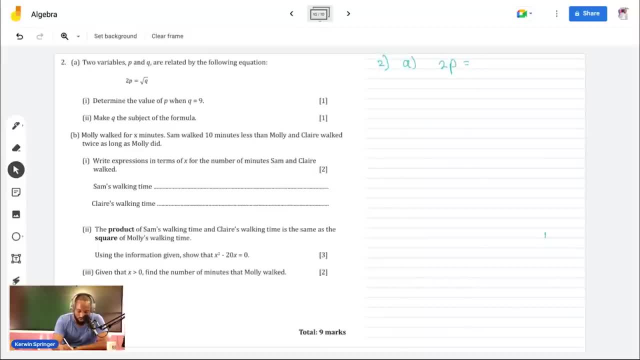 kind of fazes me all day. 2P is equal to the square root of 9 when Q is equal to 9.. 2P, that's not how you write P. 2P is equal to the square root of 9 when Q is equal to 9.. 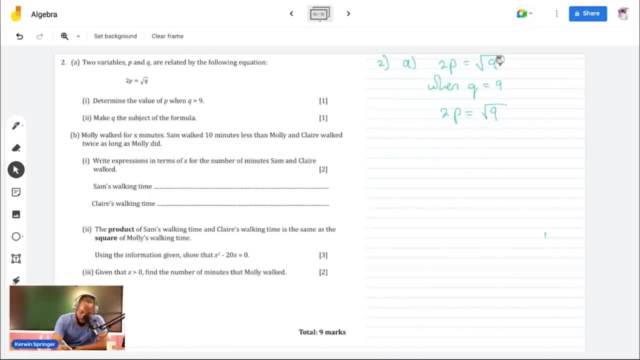 root of 9.. Why my Q and my P look in the same way, boy. Okay, so 2B is equal to the square root of Q. So when Q is equal to 9, 2B is equal to the square. 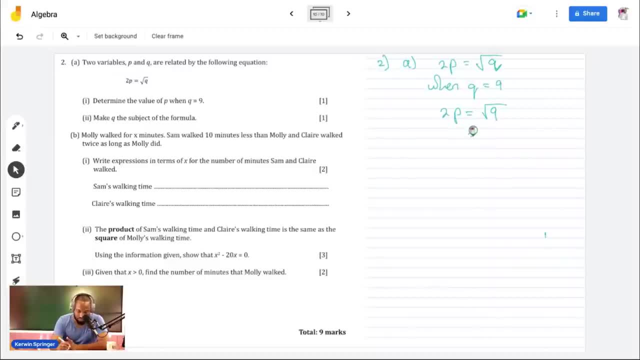 root of 9,, which is technically plus or minus 3. So 2B is equal to plus or minus 3.. So P is equal to 3 over 2 or P is equal to negative 3 over 2.. When you get the 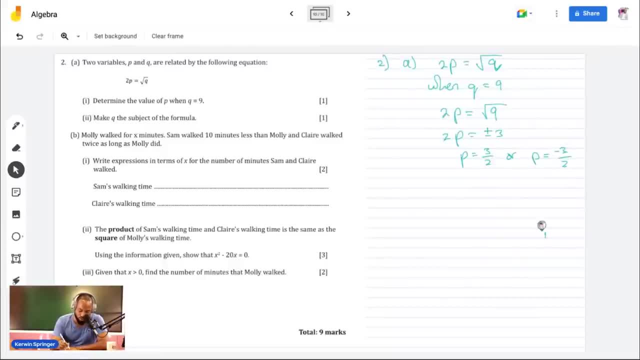 square root. it could either be positive or negative. Now, usually people make a big thing out of this right, Like if you don't put this, you're supposed to lose a mark. But usually in CXE and I think I saw- 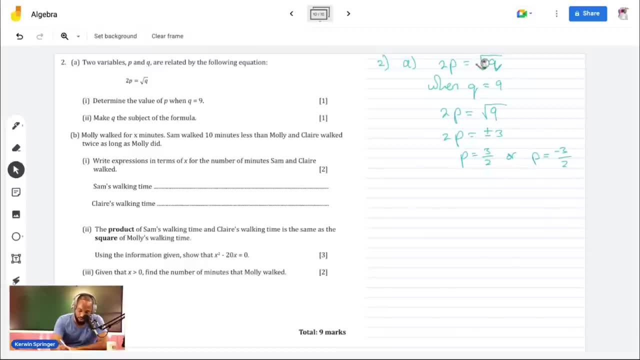 this in the syllabus: when you have the square root symbol, you assume positive unless stated. So when they want you to assume positive or negative, they'll usually do this plus or minus. So yeah, that's a little caveat there, but if you're feeling the 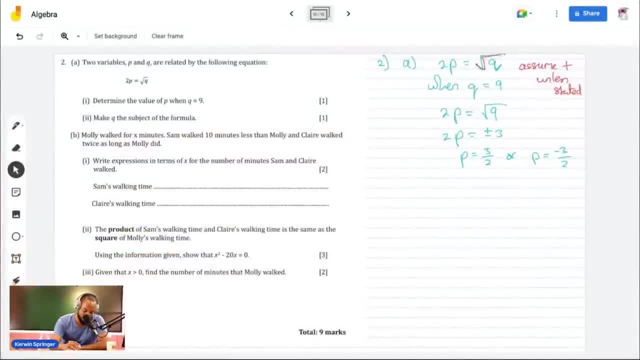 heebie-jeebies, and I would put in the negative as well. Make Q the subject of the formula. Yes, my pleasure, my pleasure, I can do that for you. So B make Q ratio whatever. 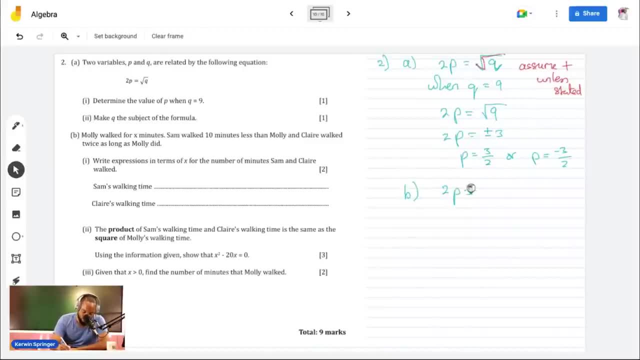 make Q right. so 2 P is equal to square root of Q. To get rid of the square root, we want to square both sides and we'll end up with a nice 4P squared, Because 2P by 2P is. 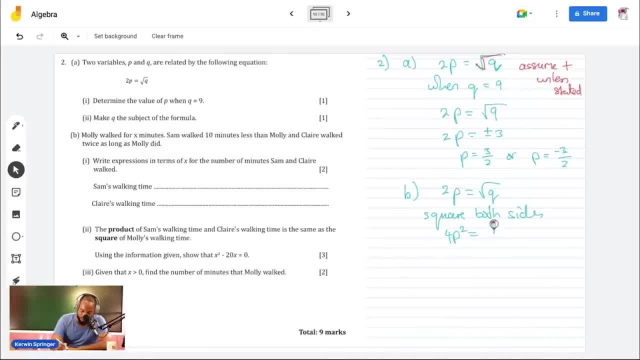 4P squared. and when you square a square root, you just end up with it's like you cancel it off, It's like it was a square root, and then you square the square root and you just you unclothe the. 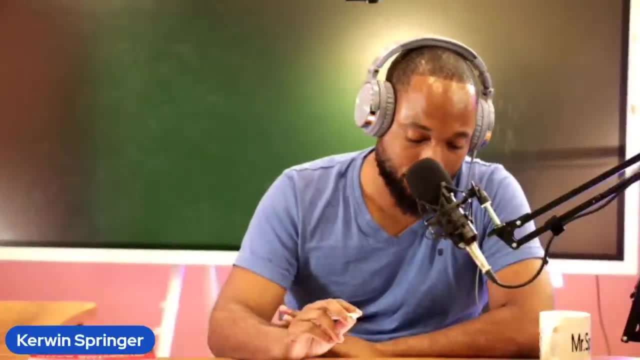 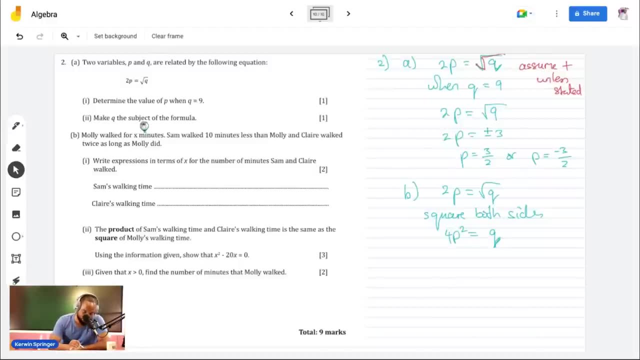 square root there. so you just stand up there, Exposed Q by the end there, Max. Let me do the next part. So Molly walked for X minutes. Sam walked 10 minutes less than Molly. Hey, I could fill that in one time: 10 less. 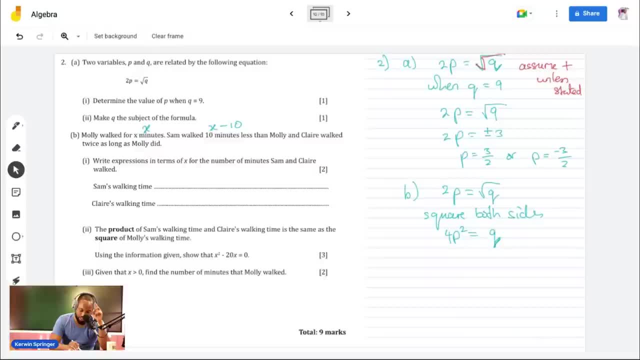 than X And Claire walked twice as long as Molly did. Hey, I could fill that in one time Twice as X Right expression In terms of the number of minutes. I don't have that for today: X minus 10 and 2X. 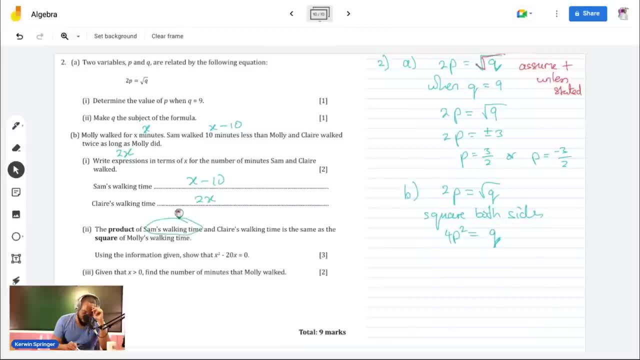 And the product of Sam's walking time and Claire's walking time is the same as the square of Molly's walking time. Jeez, that ages. We need a new page. We need a new page, All right. so let me see. Let me see. 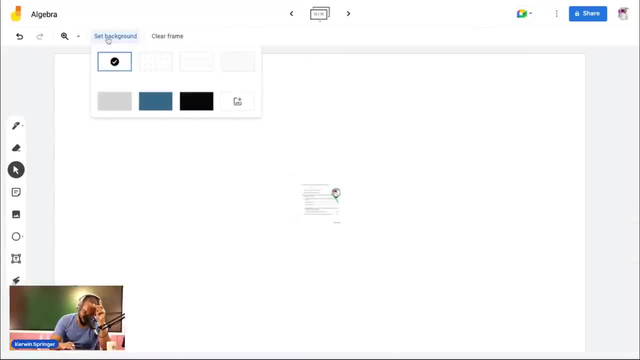 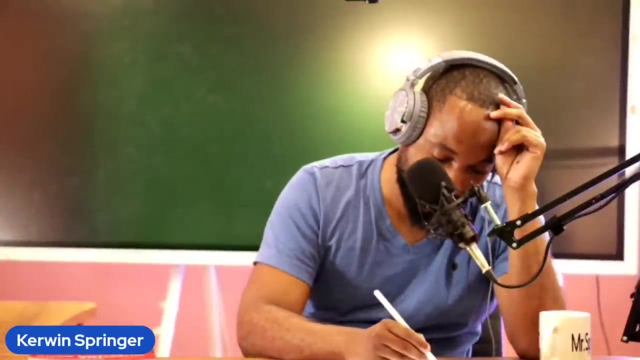 Next page. Next page: Last question. Last question, for real, this time For real. They are trying to get the question to open up, but they don't want to. Okay, So just bring it back. This man, Sam, was X plus 10.. 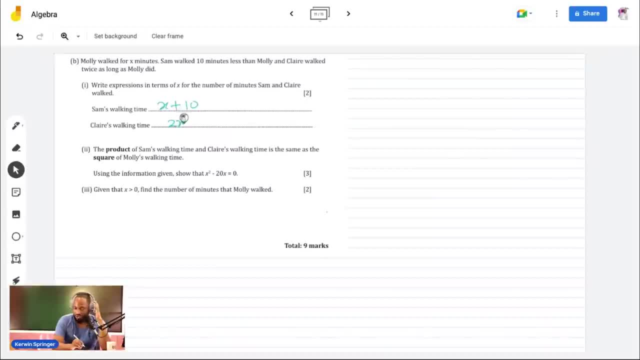 And Claire was 2X. I had a student named Claire, 2X from St Lucia, 2X Claire. if you're watching hello X plus 10, 2X- Right expressions in terms of that. 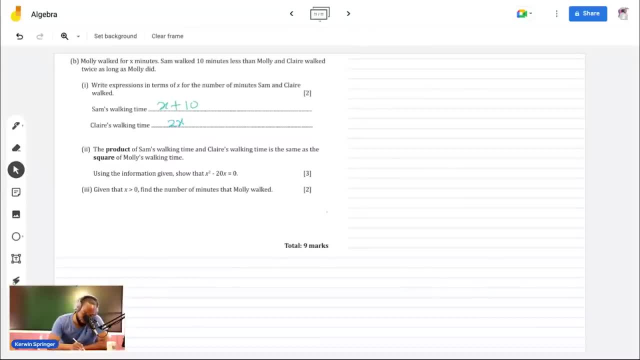 We collect with two marks, So let me take this one step by step: The product of Sam's walking time, So X plus 10 squared- And Claire's walking time. What we're seeing is the product of Sam's walking time and Claire's walking. 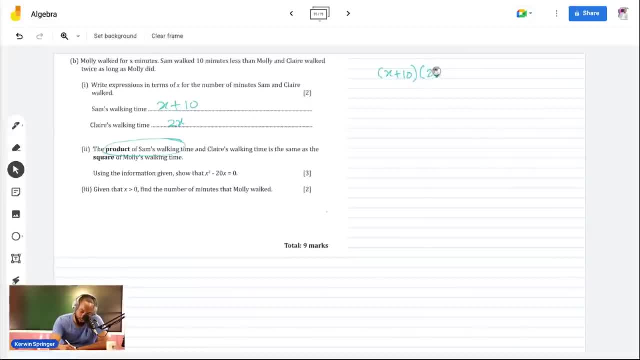 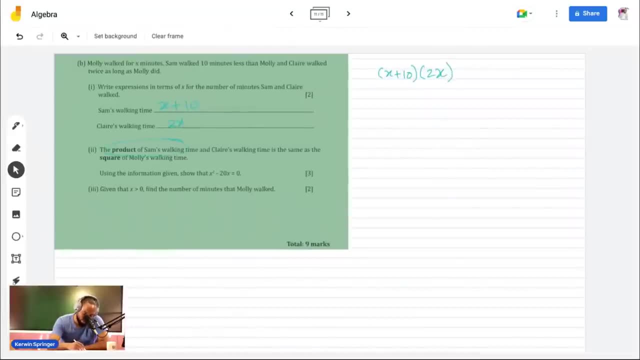 time. So I just need to multiply. the two product mean multiply, So the product of this and this, Sam and Claire, We going good so far, I feel like we going good so far. The product of Sam and Claire, Sam and Claire Is the same as. 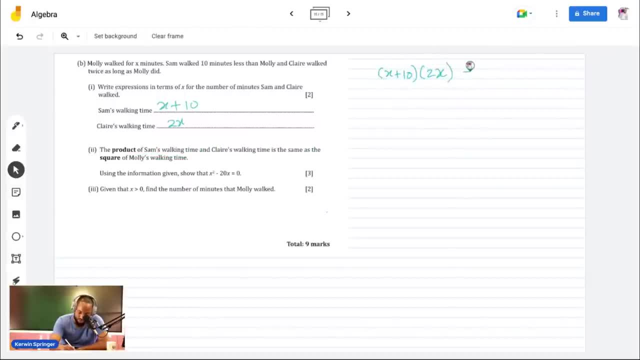 And when you say is the same as, what does that mean? Is the same as the square of Molly's walking time. So you had to take Molly's walking time- Who is Molly again? Molly is just the X And square that up. 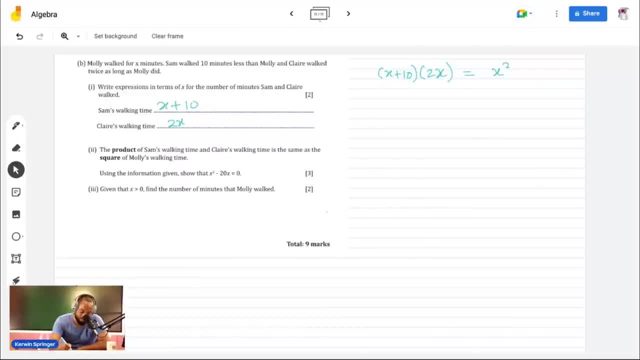 Nice, Nice, it is. Use this information. Oh, there's a show that question. We love them. show that question because you can work it out and see if you get your answer, Because they give you the answer, You just need to match it up. 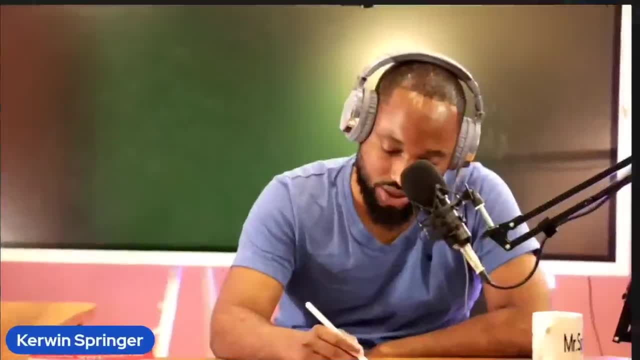 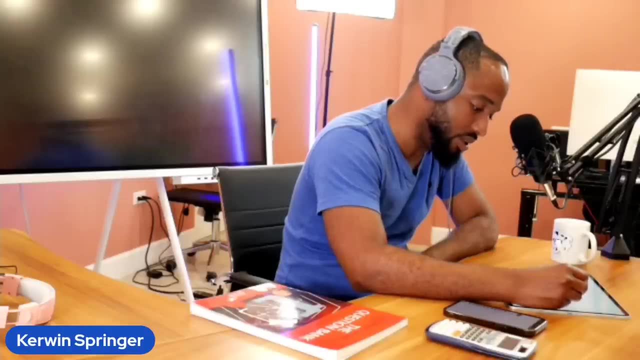 now. So yeah, we could do that for them. We could do that. So this is distribution. So this is really 2X squared plus 10 by 2X is 20X equal to X squared. Bring across that X squared to meet your friend. 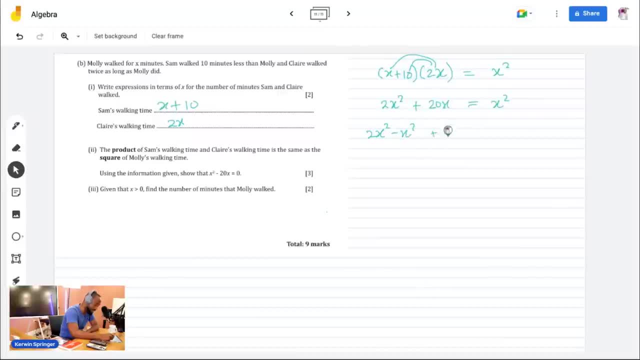 It's really 2X squared. 2X squared minus X squared plus 20X is equal to 0.. So at the end of the day, this is just X squared. Hold on, We're at negative 20.. Only, I make a mistake. 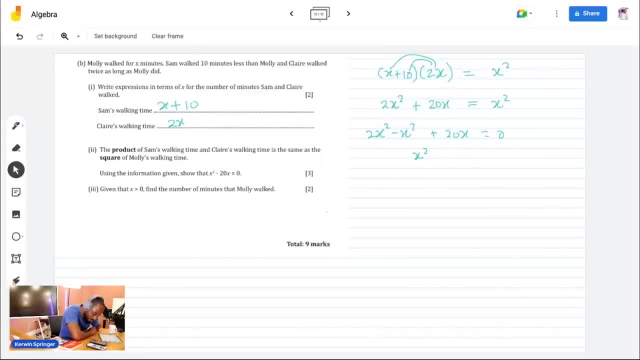 They was probably telling me that. in the chat We look at people telling me that And really make a mistake. Well, I make a mistake. I might be fair to myself, But you see I had the negative 10 on the previous slide. If we go back, 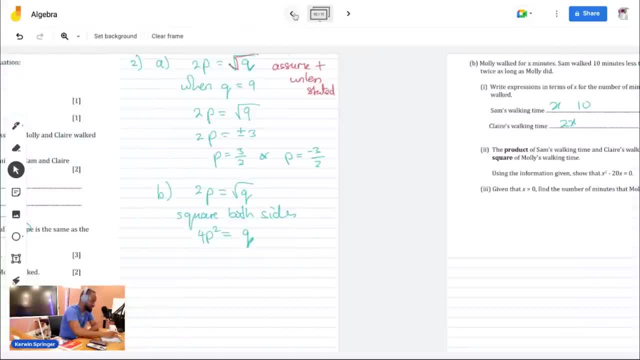 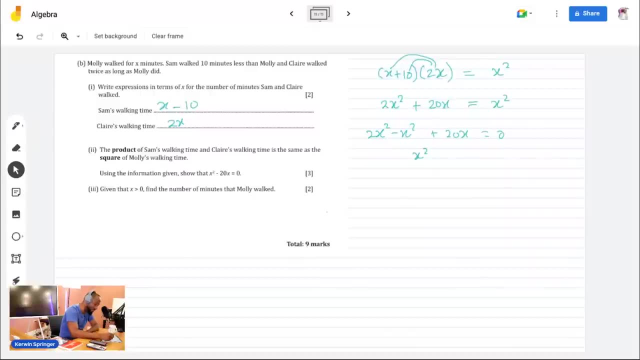 to the previous slide. you see the negative 10D. So I, just when I was bringing it across, I forget to put negative. My bad, My bad. Now I like them. show that questions for because if by chance I make that mistake in the exam when I reach. 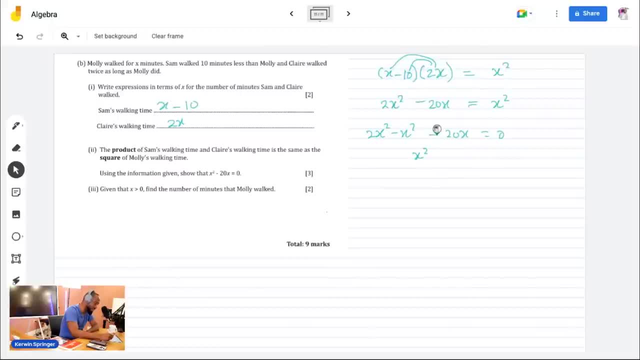 down there like where that negative come out from and boom, you realize it's supposed to be negative 20X. You could go back and fix the mistake. Love in the house. Love in the house. So it's negative 20X and we're good to go. 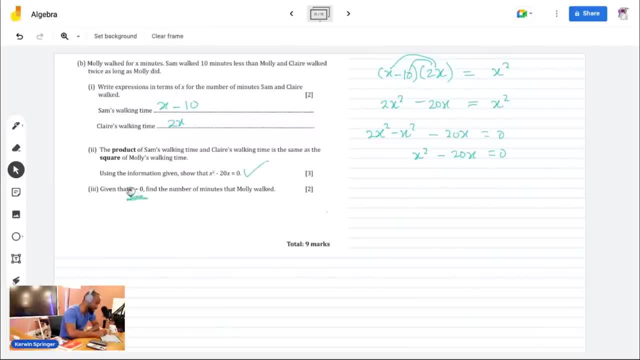 there Boom, And given that X must be a number that's greater than 0,, finding the number of minutes money walks. So we just need to go ahead and solve this now. Now, when you see a quadratic like this missing the C term, those quadratics are: 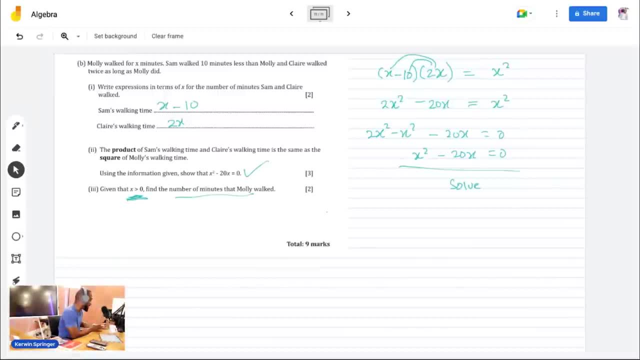 extremely easy to solve. You just factorize all the X and either that one is 0 or the next one is 0. And they're saying X must be greater than 0. So it's not a 0. So factorize all the X, I'll get X into.